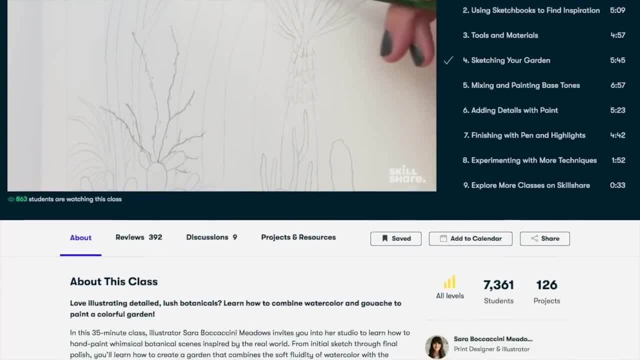 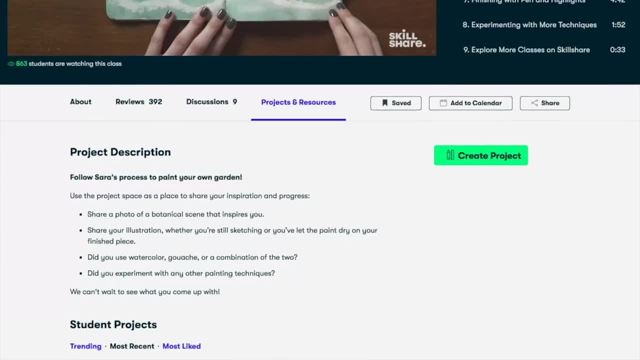 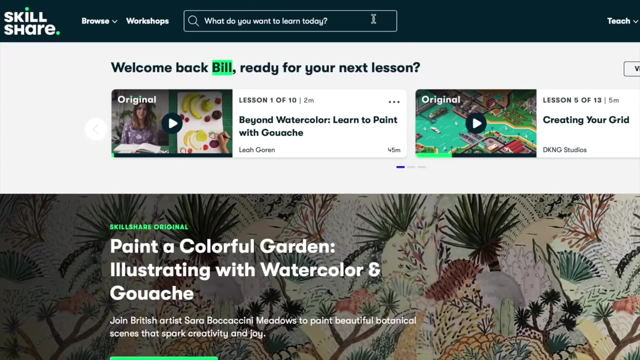 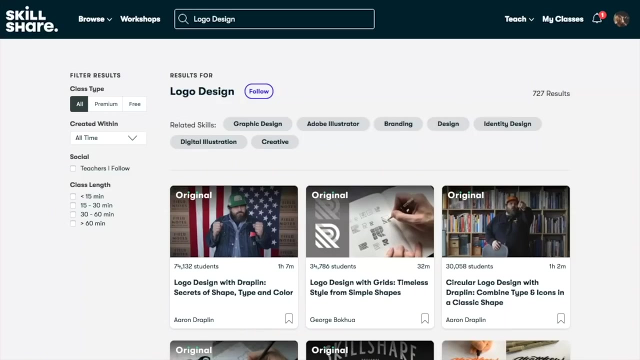 of various and exciting topics, varying from graphic design and web development to animation and production, and many, many more. If you're creative and curious, or even a lifelong learner, you will find something in Skillshare for you. Now, Skillshare classes include a combination of video lessons and class projects. Classes are intentionally made under 60 minutes in order to 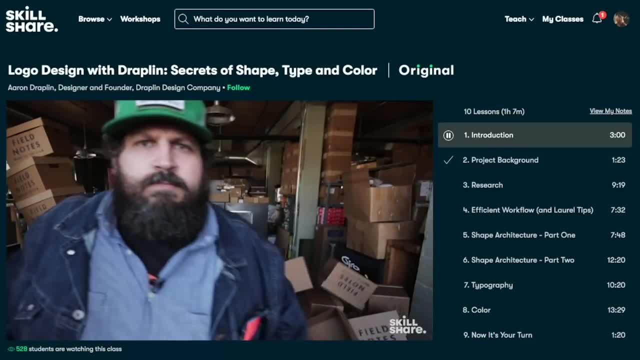 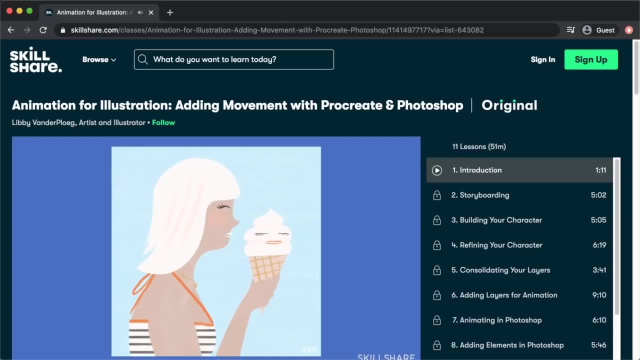 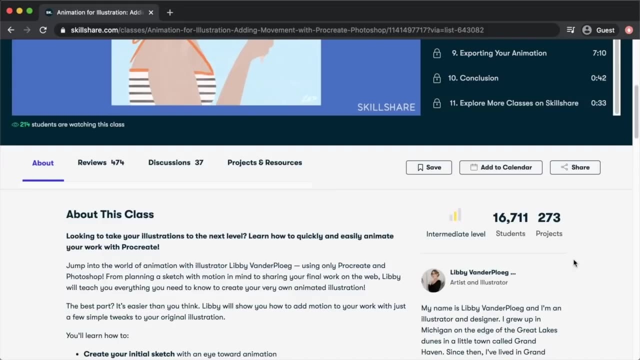 fit any schedule. For example, I myself have found high interest in the following class entitled Animation for Illustration, Adding Movement with Procreate and Photoshop by Libby van der Plog. Since I animate some of my videos, this class made it easier for a mathematical guy like myself to tap into the world of animation in 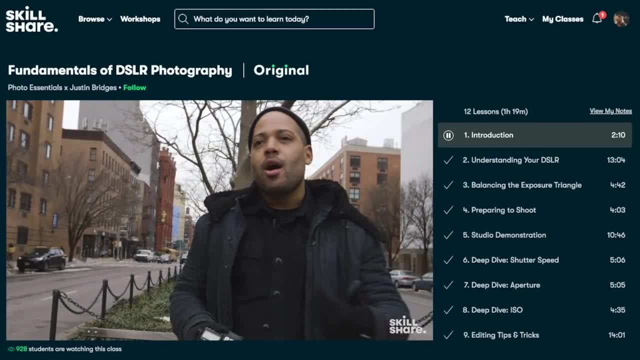 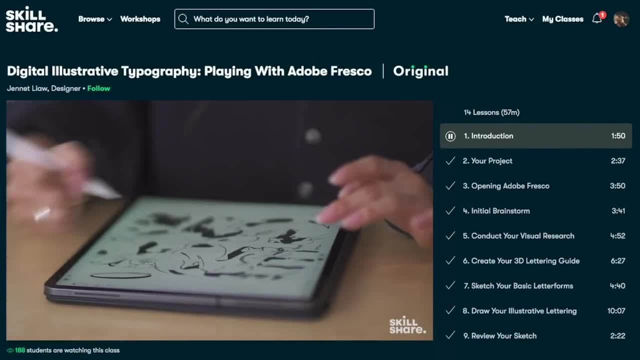 a smooth way. Skillshare is organized specifically for learning and you won't have to deal with any ads, and it's less than ten dollars a day. If you're interested in learning more about animation, you can subscribe to my channel by clicking the link in the description below. 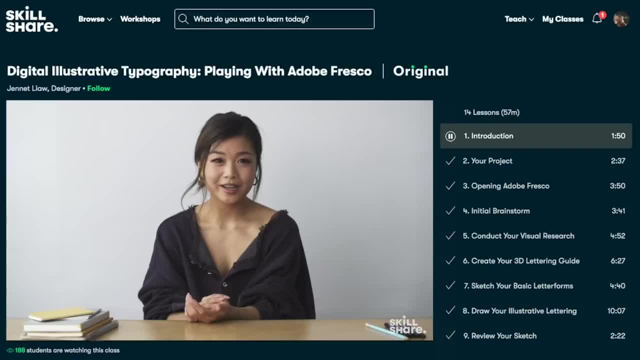 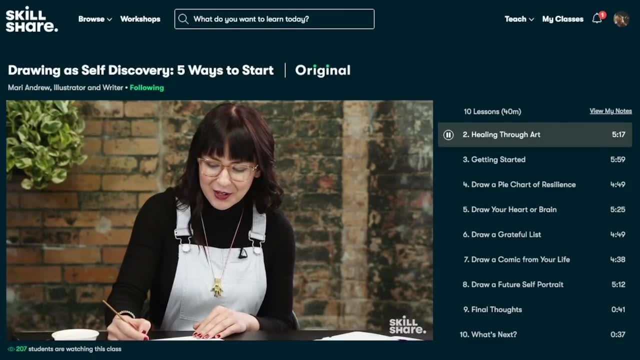 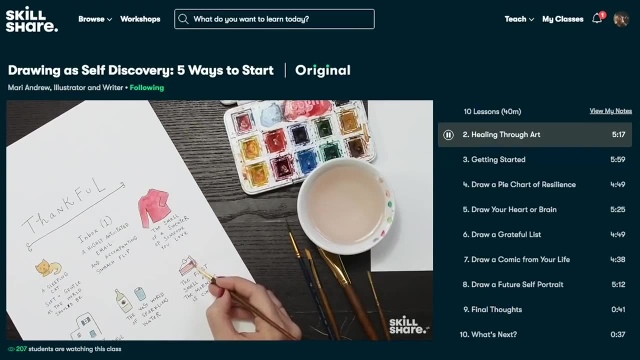 Time is a very valuable asset and, no matter what 2021 brings, you can spend it creating something meaningful with Skillshare's online classes. The first 1000 of my subscribers to click the link in the description below will get a free trial of premium membership, so you can explore. 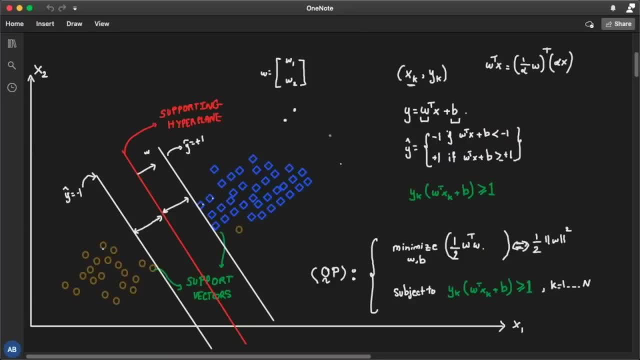 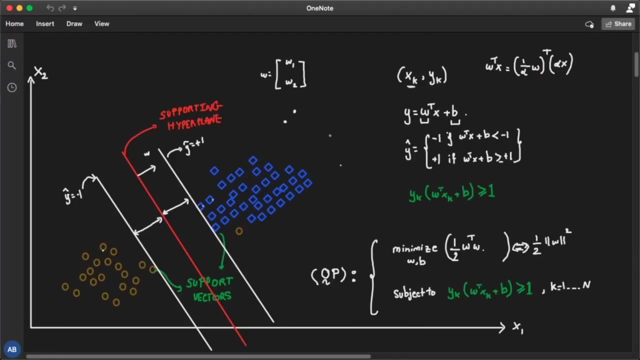 your creativity with Skillshare. So in this one we're going to introduce you to a very powerful machine learning model, that is, the SVM, or the support vector machine, along with its different linear variants. That is, we're going to introduce what a hard margin SVM is and its corresponding 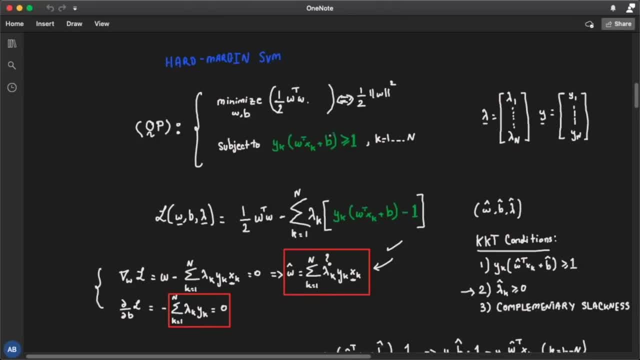 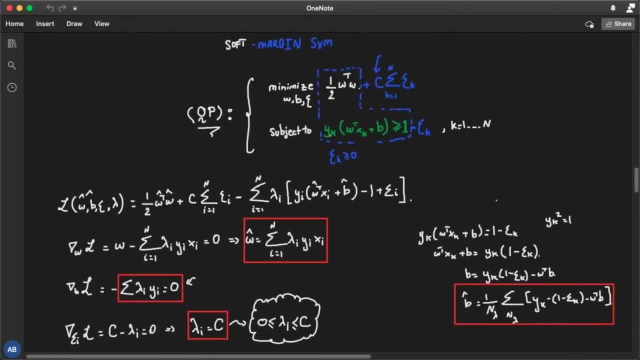 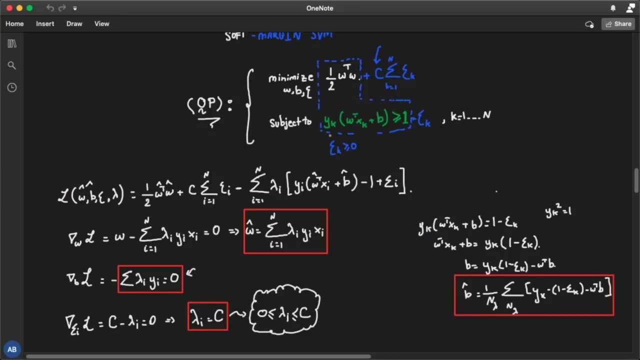 convex optimization formulation. We're going to see how to solve it using KKT conditions and the Lagrangian. We're also going to show you the soft margin: SVM, along with its convex optimization formulation, and using the same approach, we're going to solve this problem. A python implementation of 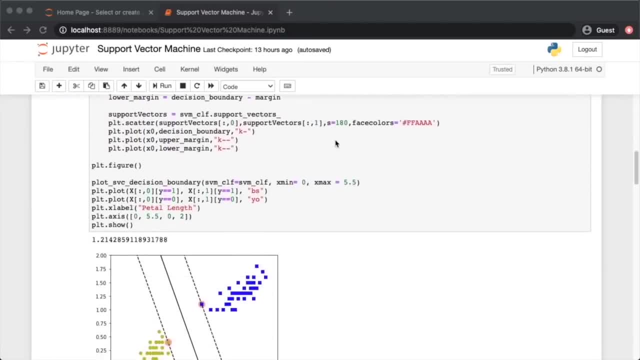 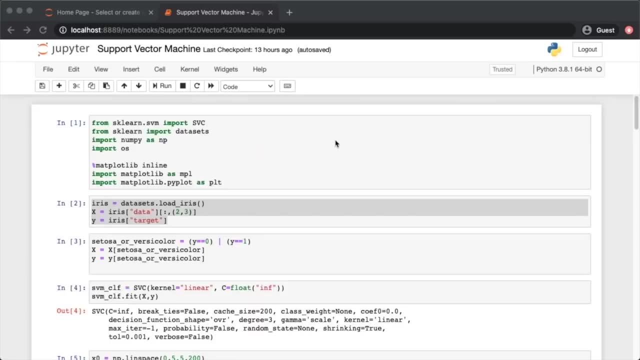 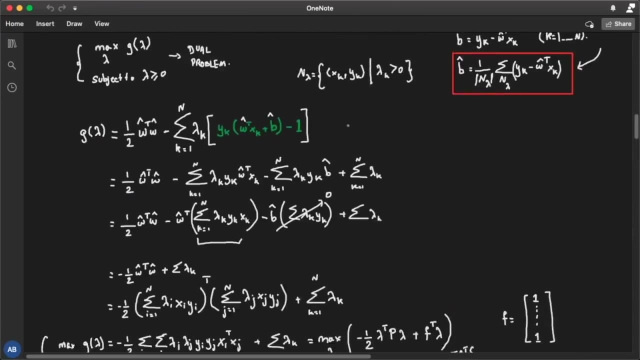 both soft and hard margin SVMs is going to be given along the way for presentation purposes, and in the next lecture we'll be dealing with the non-linear type SVM. So without further ado, let's get started. One of the most powerful and easy to understand. 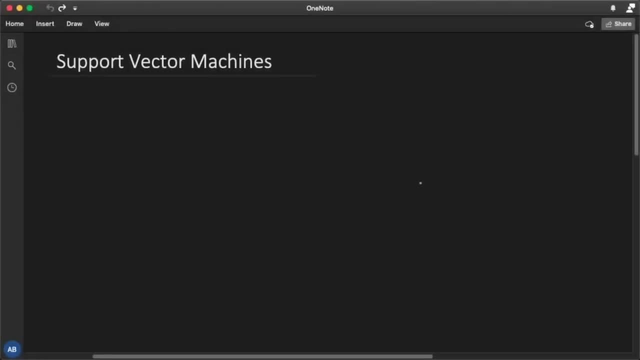 models in machine learning is the SVM or the support vector machine. Not only is it capable of performing linear and non-linear classification, but it is also capable of regression and even outlier detection. It is probably one of the most popular models in machine learning and it's really very interesting and mathematically a nice topic on its own. 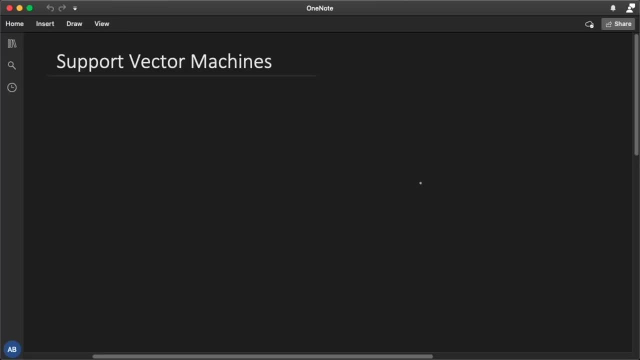 So in this lecture we'll be modeling support vector machines. we'll show how to formulate a convex optimization problem that will lead us to different types of support vector machines, such as the soft margin, the hard margin and even the non-linear. 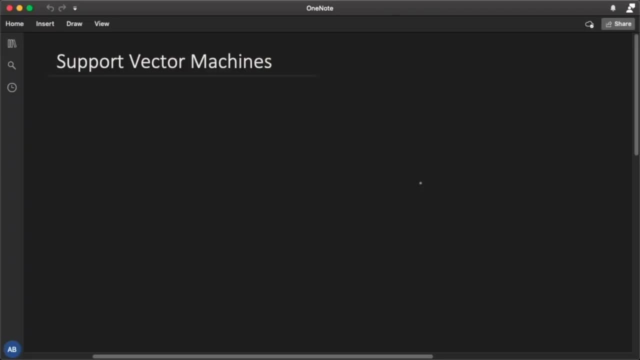 So soft and hard are both linear SVM classifiers. We'll be also tapping upon non-linear SVMs, such as the ones that utilize kernel methods, and we'll be seeing why. we can, you know, use kernels to generalize the notion of linear SVMs to non-linear ones, thanks to a very important theorem, that is Mercer's theorem. 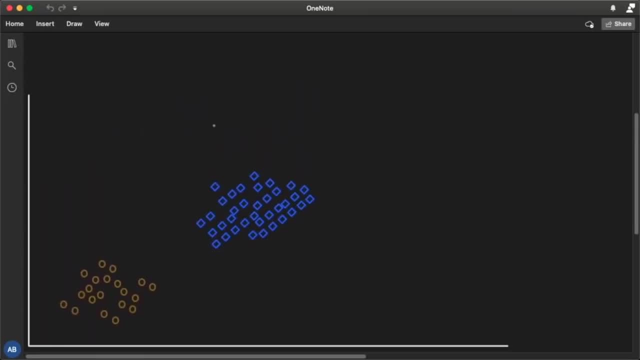 So we'll be starting off by a given dataset, the one we're going to talk about today, which is the one we're going to talk about today. So we'll be starting off by a given dataset, the one we're going to talk about today, which is the one we're going to talk about today. 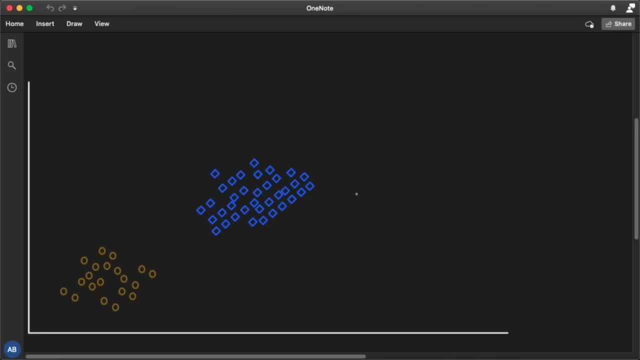 that we see over here. So let's say I've got two features that are x1 and x2.. And my interest here is to perform classification right. So I'm given this dataset, though the circles are classified as maybe zero and the squares as one. So the fundamental idea behind SVMs is: 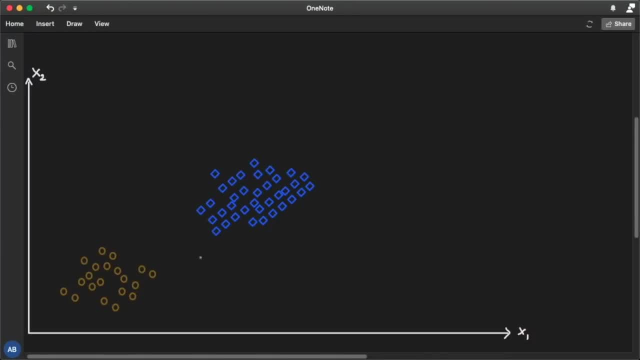 to fit a line or, in higher dimension, a plane or hyperplanes that separate or properly separate those two datasets. So many questions arise, naturally arise here. The first, that is: is my dataset linearly separable? Are they? is there any outliers in my dataset? All those effects. 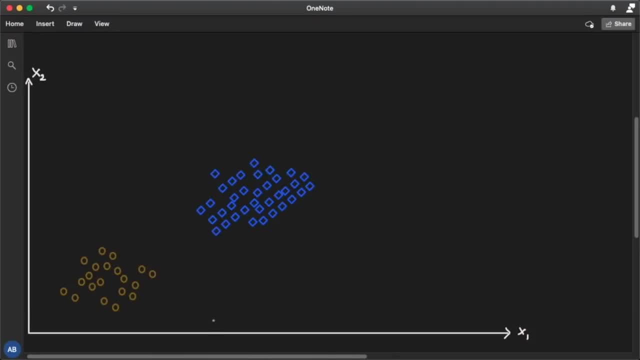 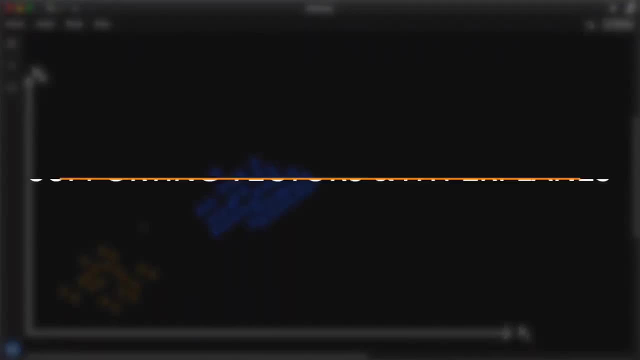 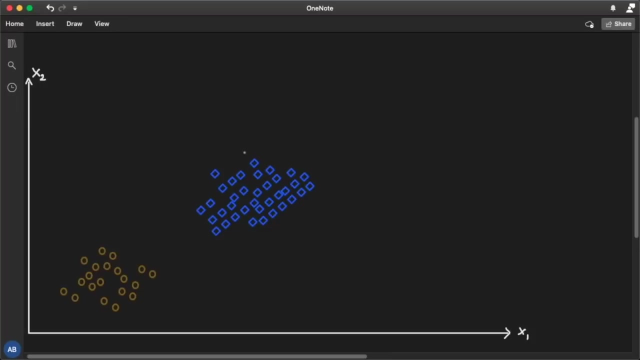 will affect the performance of, you know, finding the optimal plane that separates both datasets. okay, So, naively speaking, what someone could do is, you know, tweak around to find a really good line right to separate both datasets. So one might choose the following line, which is: 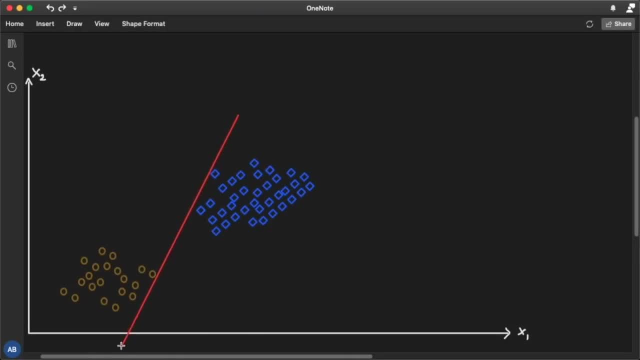 probably a good choice- The following red line and say: oh okay, I found this line- that is a heuristic line- right, Because there's no mathematical explanation why we chose it right. But, as you can see, this line is supporting the support vectors. let's put it that way. So what are support? 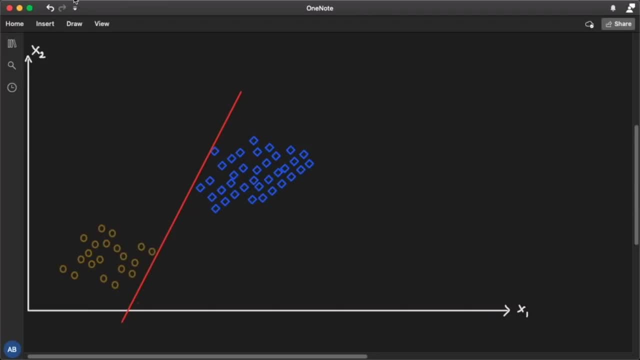 vectors. in that case there are instances. I'm going to highlight them over here. So this instance right here is a support vector as well as this one. So those are both support vectors belonging to different datasets. And why is that? It's because if we center a hyperplane, that 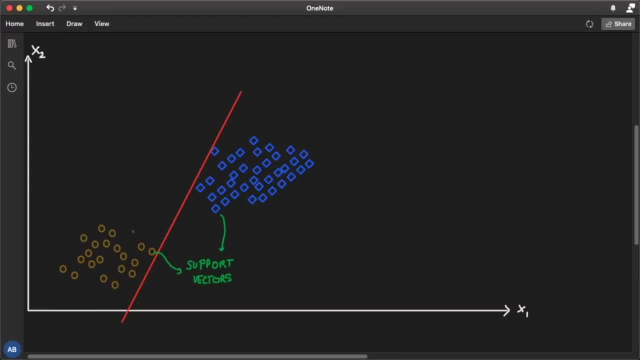 you know, falls in the middle between both datasets. well, those two vectors are on the edge of the street right. So if I were to, you know, put a line on the edge of the street right. So if I were to, you know, put a line on the edge of the street right. So if I were to 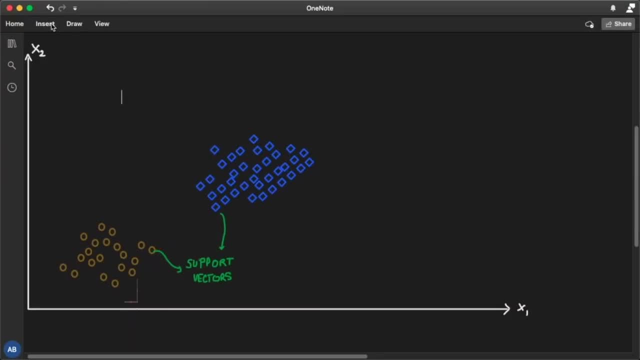 you know, remove this line and say I'll insert this one over here And another one over here, right? It's as if those two vectors are are points where those two lines pass to separate both datasets. So all I need is those two points to separate those two datasets. 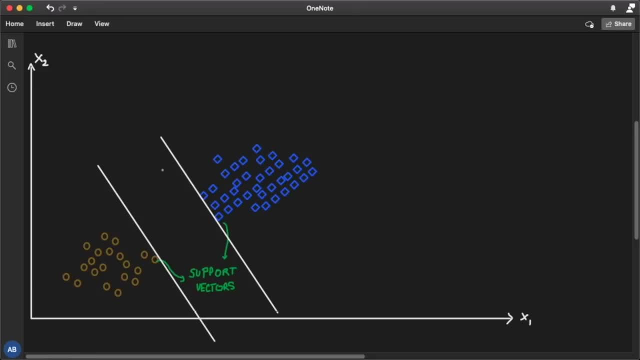 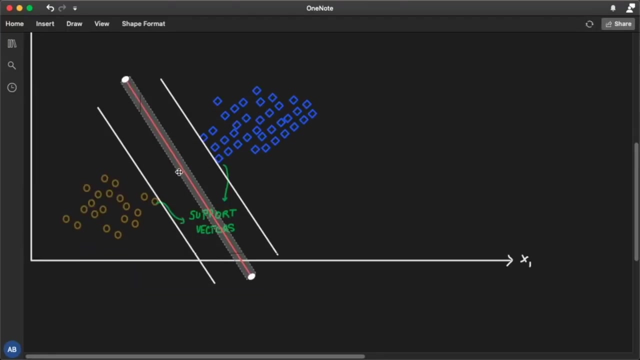 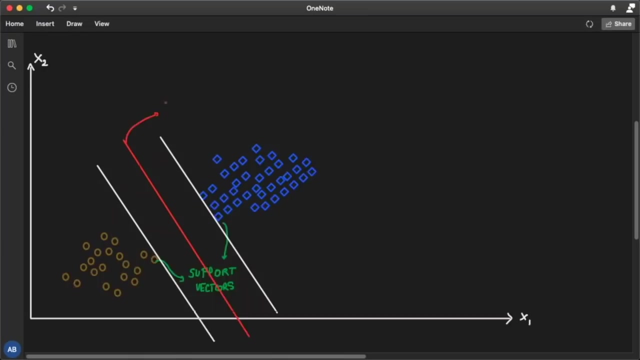 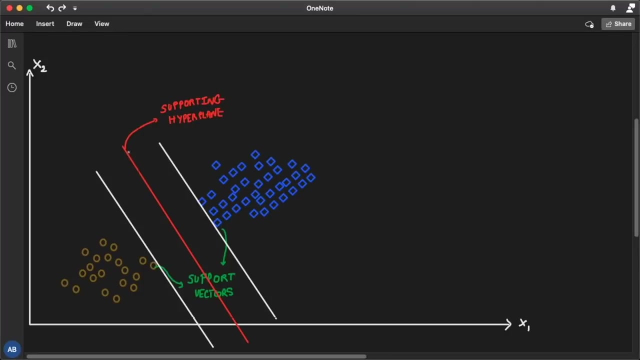 Okay. So in that case, what SVM or the hard SVM would do is pass a line in the middle of those two support vectors, Okay, And this hyperplane or line would then be called the support, the supporting hyperplane. Okay, So now the question is the following: How could I find this supporting? 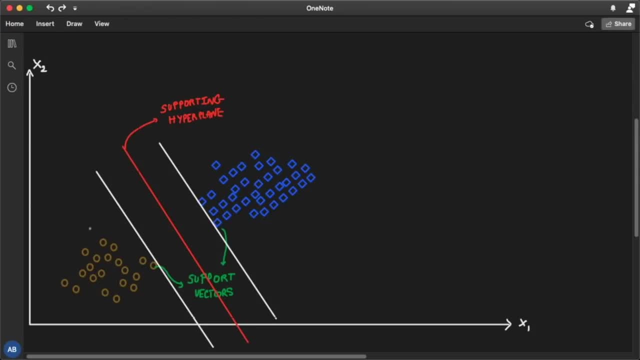 hyperplane, given my training set, that is, both datasets and their corresponding classes. Well, um, I did explain this in one of my convex optimization application lectures, which I'll be leaving down in the description section below, And I'll repeat the derivation. 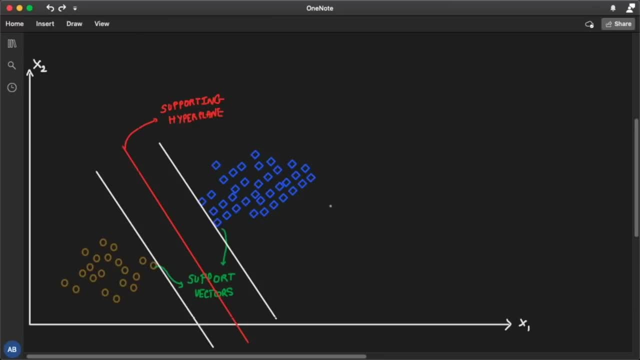 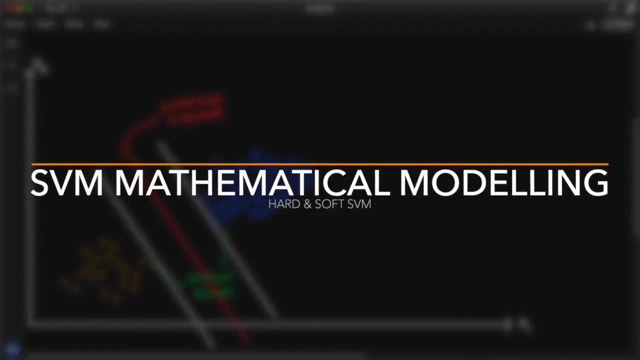 over here because I want to also extend it to non-linear SVMs. In the convex optimization application lecture, we were only restricted to linear and hard margin SVMs. Okay, So over here what we're given. instances right Of the form X. 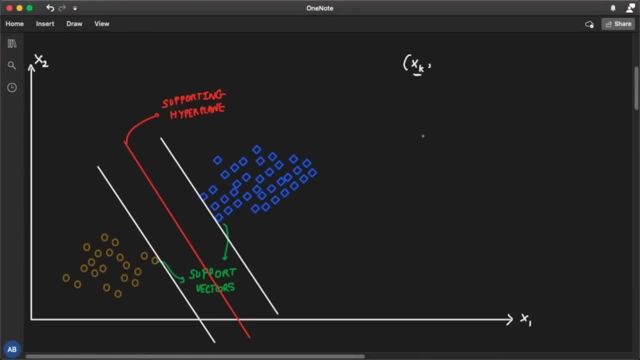 K and their, which are vectors containing points X1 and X2 in this particular case, and their target values or their corresponding classes, YK. So if XK belongs to the circle class, my YK is zero, else it is one right. Our aim is to find a hyperplane right That is of the form Y, equal W transpose. 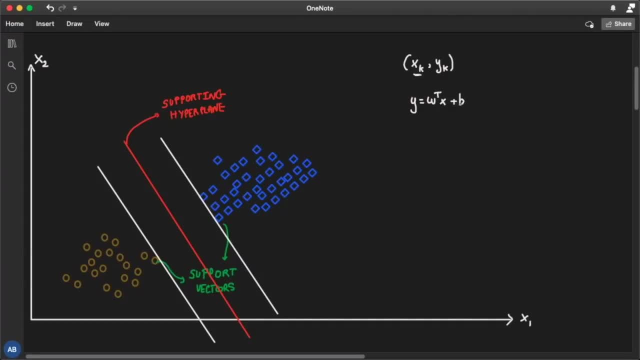 X plus B, right. Our aim is to find W and B, so that for each X I want to evaluate its corresponding class Y. If it lines on top of the line, we say that we are in the square class, else we are in the circle class, right. So in other words, if we say that my Y hat is zero, if 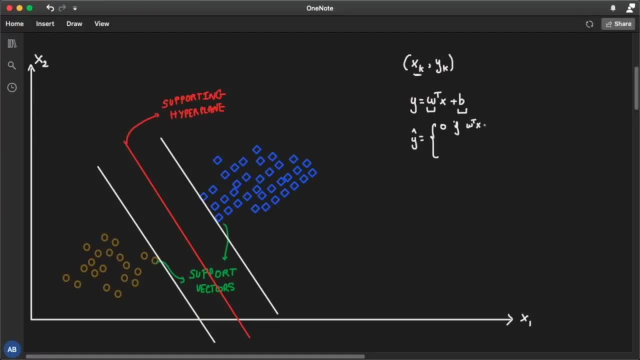 we say that W transpose X plus B is negative, or instead of zero, we can assign a minus one and a plus one. If point X lies on top of the hyperplane, W transpose X plus B. right, So I have a W transpose. I don't have a K, I'm just going to write it down. It's going to be a two. And then we'll write down the W transpose X plus B as negative or instead of zero we can assign a minus one And a plus one if point X lies on top of the hyperplane. W transpose X plus B right. 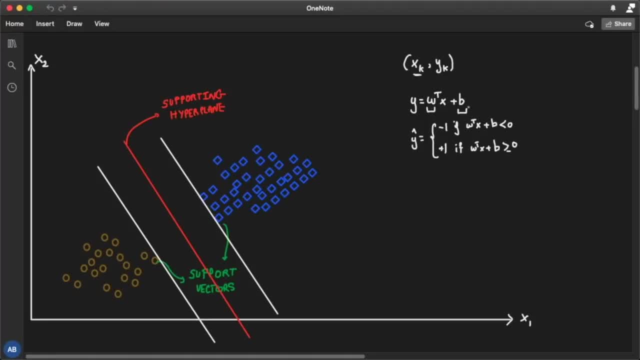 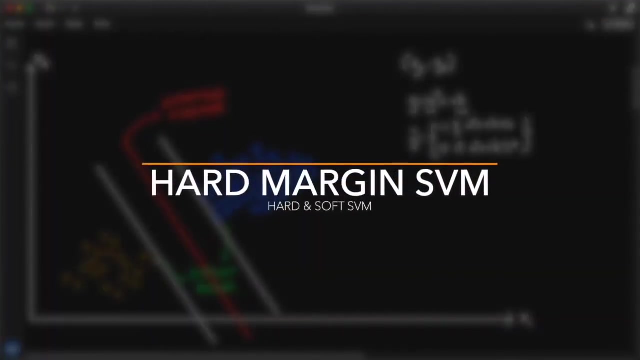 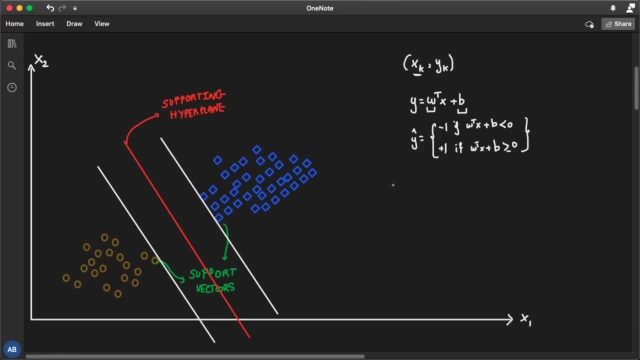 As you can see over here, our aim is to find W and B with the following constraint right. So those two equations could be seen as constraints. Now, replacing both constraints using one single equation, we can see that if I denote by: 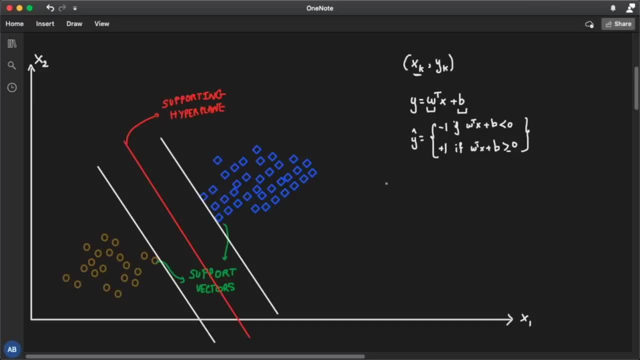 so let's say I'm given N samples or N, the number of instances is N, So the number of squares plus the number of circles is N. Then, and also referring to the Kth instance as XK, YK, then the first equation satisfies. 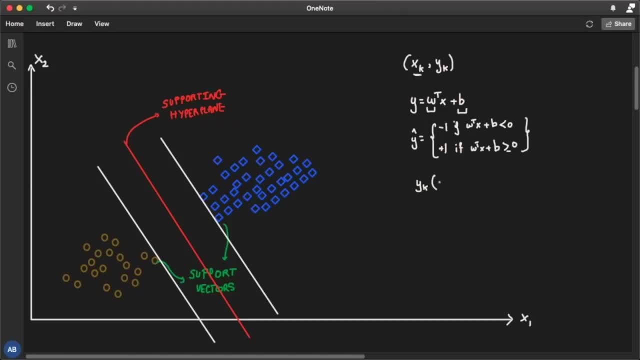 YK multiplied by W. transpose XK plus B. Since this guy is negative and so is this guy, then this guy multiplied by this guy is positive. This is for the first case, But this is also true for the second case, because YK is positive and so is W. transpose X plus B. 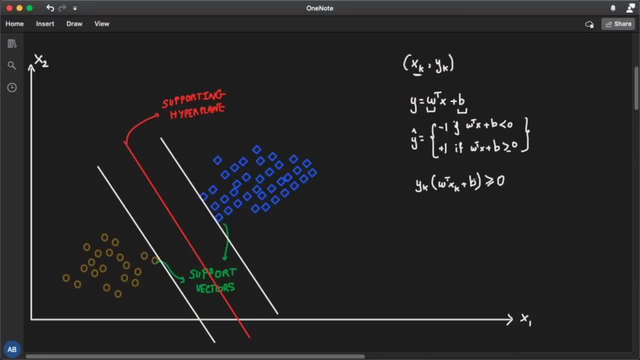 So this guy is a constraint, right, And actually it is the only constraint if we were to solve a hard margin linear SVM problem. okay, So what are we doing here? We are optimizing a certain cost function subject to this particular constraint. 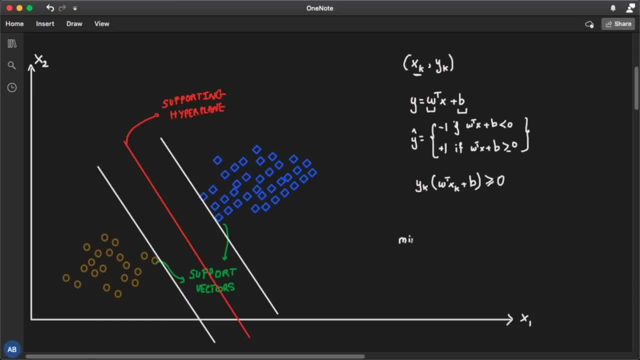 So I'm trying to minimize a certain cost and we'll see what it is just about a bit. So this optimization is going on with respect to W and B, because those are the two quantities that define the hyperplane. W is the gradient right. 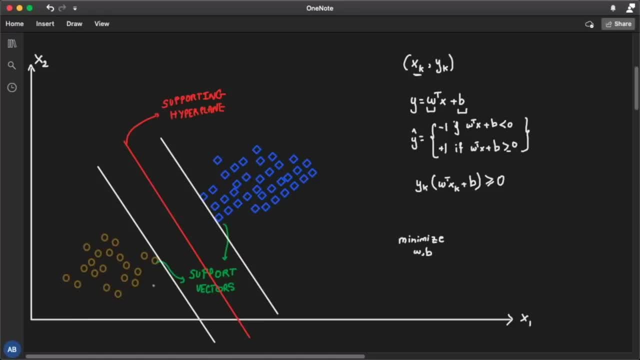 And B is an offset. If B is zero, then this line would be passing through the origin right. So we're minimizing a certain cost, and I'll state what it is just about now. And Y subject to this constraint over here. 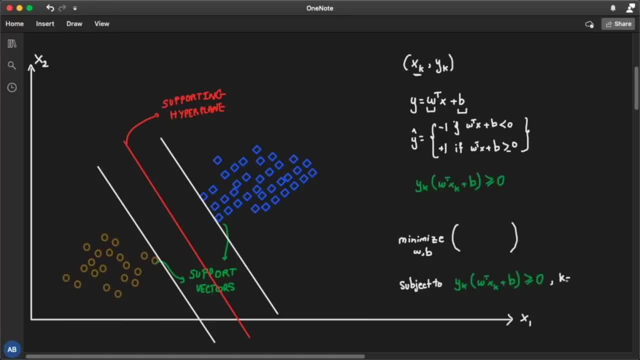 And this guy applies for K, going from one down to N. So for all my training instances. Now, what am I trying to minimize here? Of course I'm minimizing functions of W and slash or B, Right, Okay. so what is an appropriate decision or cost function? 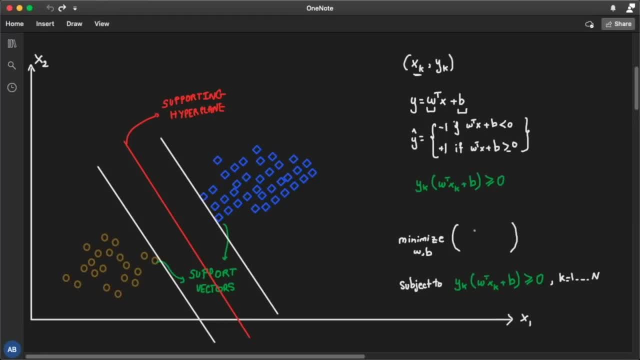 that I need to minimize. that seems suitable over here. well, let's take a look at the gradient for a bit. we said that the gradient W, it's the one that defines, it's the vector that defines the direction of the plane. right then, it seems natural to include W in. 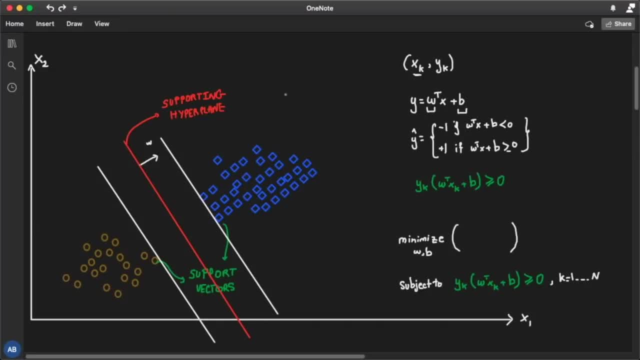 our cost function. now, let's say, our optimal W, without loss of generality, is W 1 and W 2 in this particular case. right then again, bear in mind that W is a direction vector. it doesn't, its magnitude doesn't hold any information right. the magnitude of W is only going to. you know, just amplify W, but it's not going. 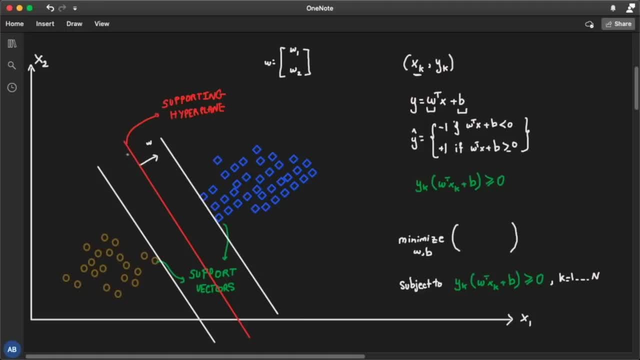 to change. you know the the sense of this line, that is, if my line looks like this: right. so if I divide, if I come here and look at the objective function, Y hat right. If I divide my W by an alpha, then my Xs are going to be multiplied by an alpha. 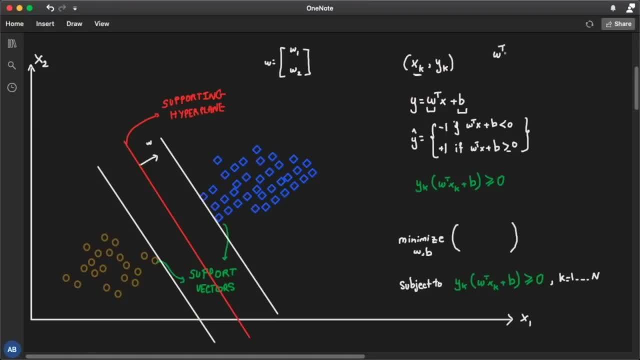 Look at it that way. So W transpose X is equal to one over alpha W transpose multiplied by alpha X. Now the larger alpha is, you can see that my alpha Xs increase. So let's say alpha is two. then I divided my gradient or slope. 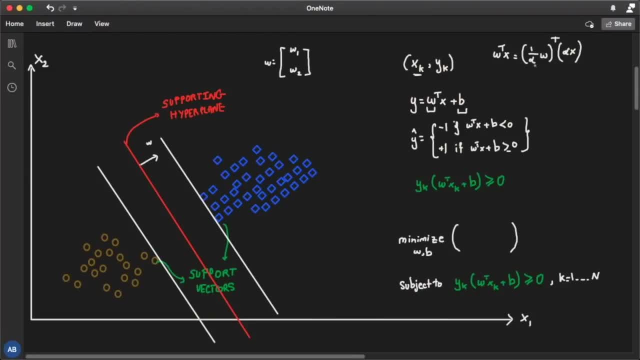 I divided my gradient vector by alpha. then my instances are multiplied by alpha. Let's say alpha is two, then we get instead of X we get two X. So my margin increases, right Margin? is this distance over here, right? 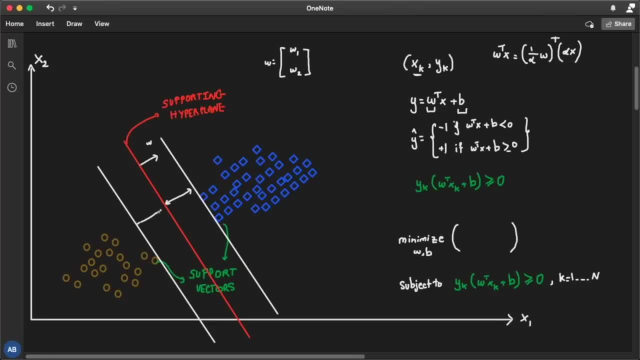 This is the margin. Symmetrically it's also this distance over here. So if I multiply my instances Xs by two, then this point would be here, And this point would be here, And this point would be somewhere here. 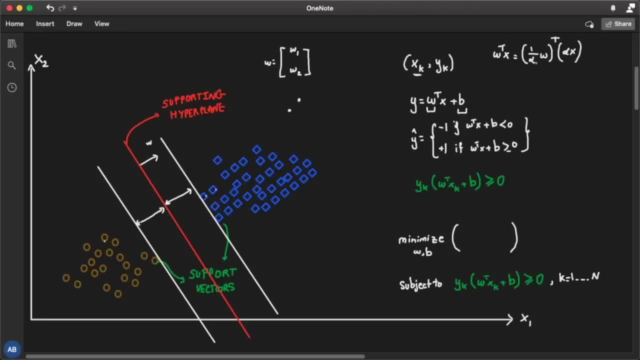 So we're increasing the margin. Thus the constraint here is to the thing here is to minimize the magnitude of W. that is we're interested in minimizing. W transpose W. Okay, And usually in references you find a half over here. That's because W transpose W is the Frobenius norm. 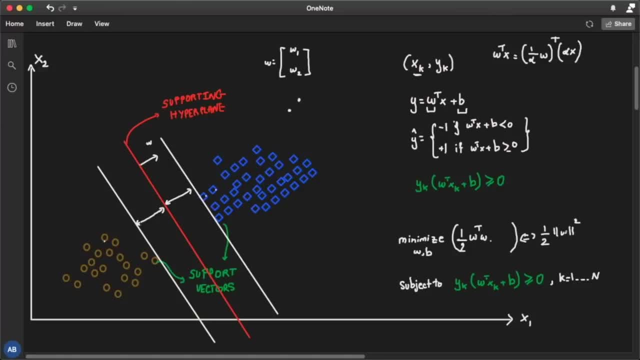 of W Squarer and thus, when taking the gradient of this cost with respect to w those two, this two vanishes or cancels out this two. right and okay. so that's what we have to say about the cost function in case of the hard margin linear svm. one last thing over here is that this problem is still loose. 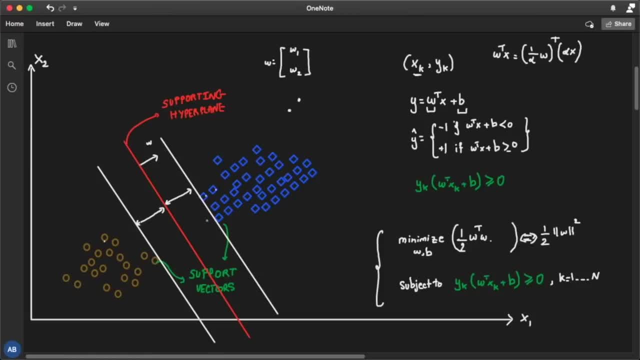 and why is that? it's because we're not, you know, we're not- taking this margin into account. okay, right here i'm saying okay. so if my, if you're giving me an xk along with its class, then i say it's zero. i say it's positive when my y hat is one and it's negative when my y hat is. 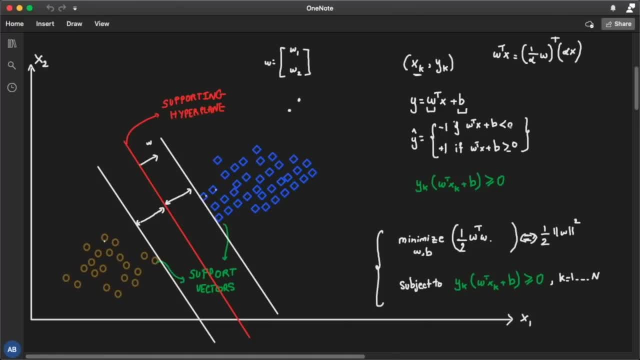 minus one. well, we're not leaving any margin. that's that's. that's the thing over here. we're not leaving any margin. um, a proper way of doing that is saying that, without loss of generality, that this line over here or this support vector over here is the one where y hat is minus one, and this guy over here is y hat is plus one. 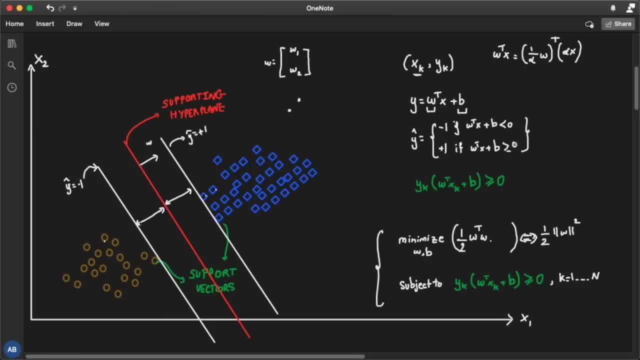 if we're not leaving any margin. that's, that's the thing over here: we're not leaving any margin. if we were to leave the problem as is, there's no margin because it's zero. so a proper way of taking this into account is by modifying those zeros into the margin values. that is minus one. 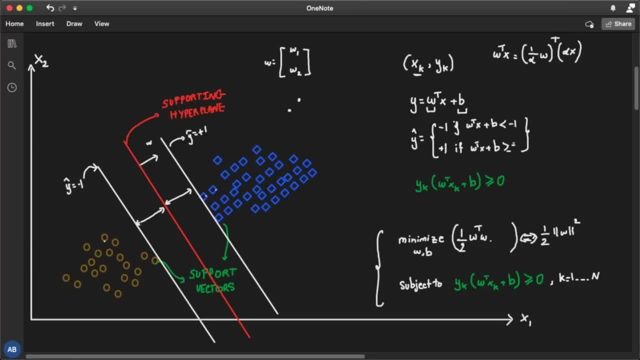 and plus one respectively. so i'm not going to classify only when w transpose: x plus b is negative. no, this is even stronger when it's less than minus one, so when it's below the support vector and not the supporting hyperplane, okay. likewise, i'm going to say that my x is belongs to class plus one when. 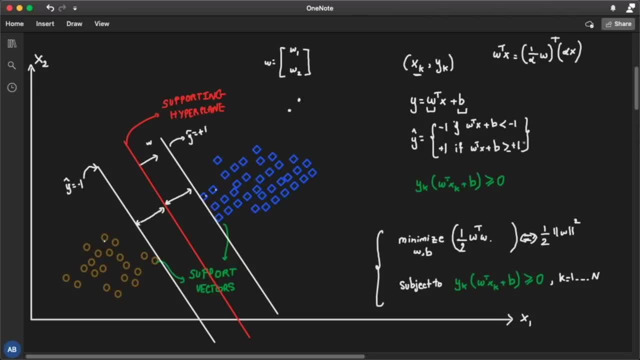 w transpose x plus b is not only greater than zero, but greater than plus one. that is the upper supporting hyperplane supporting hyperplane. okay, so in that case, multiplying y hat by w transpose x plus b is not only positive but greater than one right. it's greater than one in both cases. so this is the problem: i have to optimize and 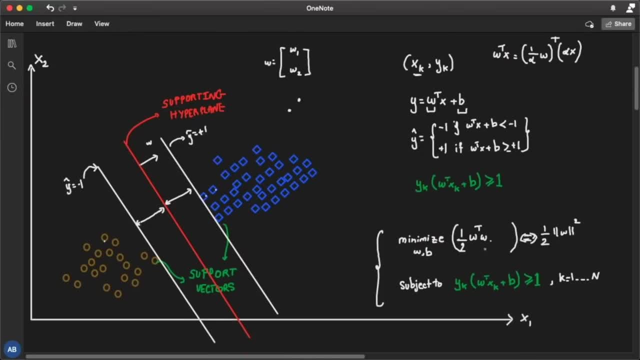 since this problem is convex. why is it convex? so if you were following my convex optimization lectures, you can easily recognize that this optimization problem is a quadratic program. why? because the cost is quadratic in w and the constraints are linear in w and b, and thus this is a qp quadratic program. okay, and so we can solve it easily using this optimization problem. 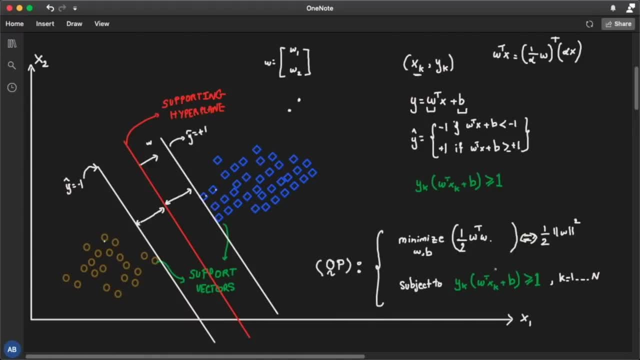 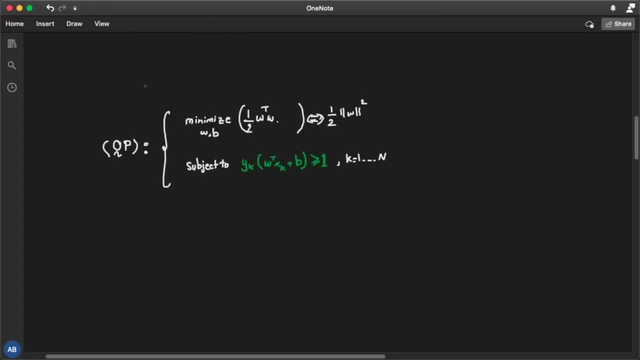 we're going to use the lagrangian function. so this is the problem we have. and note that this is a hard margin problem. why is it hard? is that because i'm classifying without accepting any outliers we're going to see just in a few moments from now? 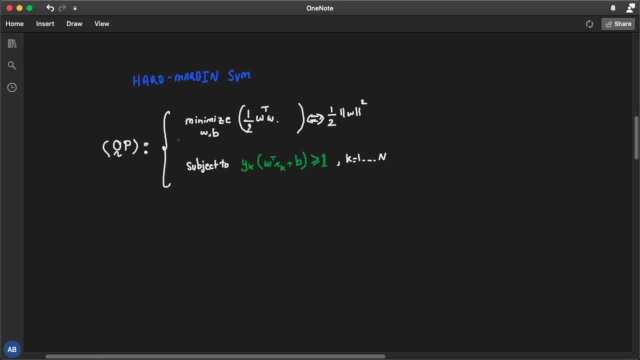 that there is also another modified version or softer version of this problem that accepts outliers. i'll explain it just in a few moments from now. okay, now let's focus here and try to see how to derive w and b. okay, um, i'm also going to leave down in the description a link for my 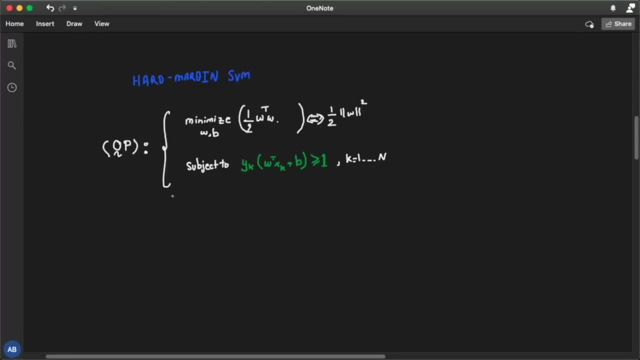 convex optimization lecture on quadratic programs. i really urge you to watch this lecture before the following derivations. okay, so before proceeding, i'm going to write down the lagrangian function of this problem, that is, a function of the variables, and the lagrangian vector, lambda. so w is also vector and lambda. over here is a. 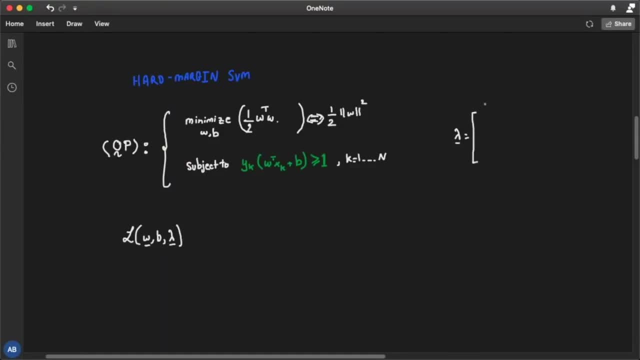 a vector containing all the Lagrangian multipliers associated with the constraints, lambda one down to lambda n, right. so the Lagrangian function, if you're following my convex optimization lectures, is nothing other than the cost function. half w transpose w and since we're minimizing, 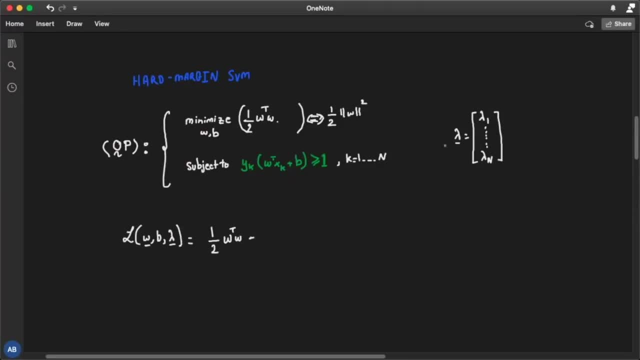 we're going to have a minus lambda k multiplied by the kth constraint, when positive, that is, I'm going to get the one on the left hand side. it's a minus one. so I'm going to multiply lambda k, lambda k with the kth constraint when one is on the left hand side, so the constraint is positive. 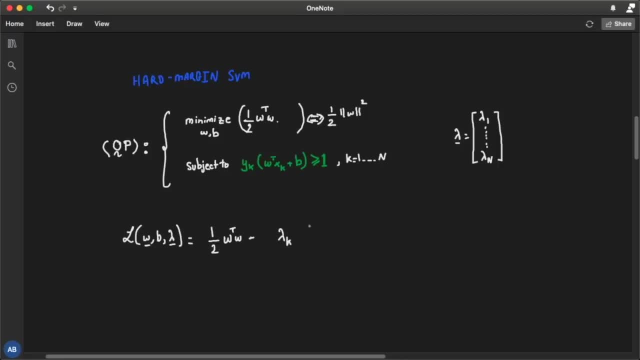 and hence I'm going to get a yk into w, transpose xk plus b minus one right, and don't forget that we're going to sum over all such weighted terms. okay, now, what you probably know from high school is that, using basic calculus, once you have a, 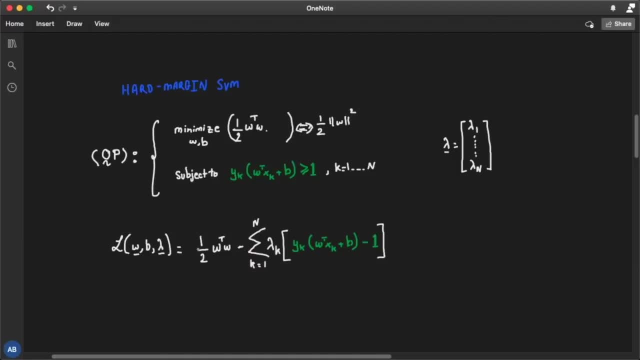 Lagrangian of the problem, then it suffices, and it suffices to take the partial derivatives of the Lagrangian with respect to the unknowns w, b and lambda. set them to zero. You get a system of equations in w, b and lambdas. 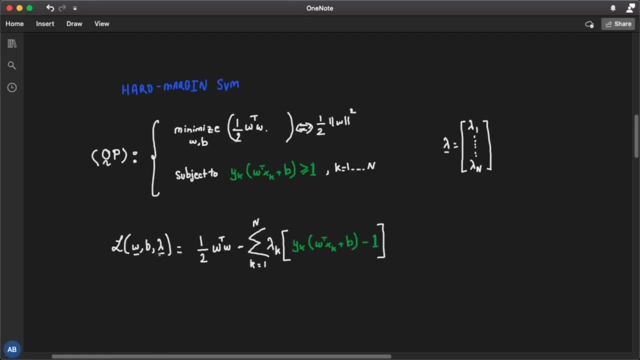 and you solve for those unknowns right. However, this method only applies to equality constraints. That is when I have a problem with equality constraints, But fortunately, under some regularity conditions which we have over here, we can also follow the same approach. 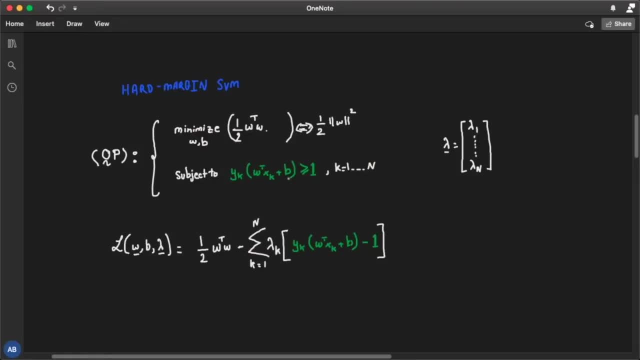 even when we have inequality constraints. And these regularity conditions are the so-called KKT conditions, that is, the Caruso conditions or Pushkin-Tucker conditions. And what are they? That is, if you solve the problem as if we have any equality constraints. 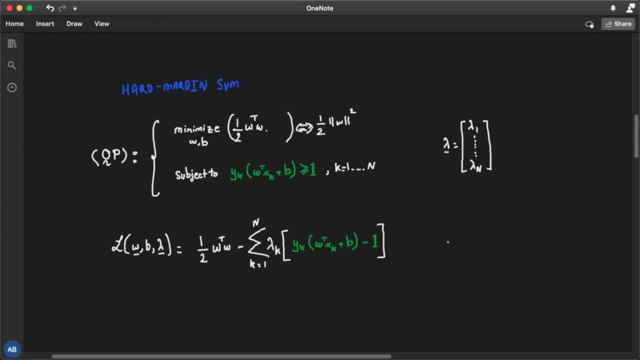 given that the solution- let's denote it as w hat, b hat and lambda hat- satisfy the KKT conditions. I also have a lecture on KKT conditions and I'm going to talk a little bit more about that, So let's get started. 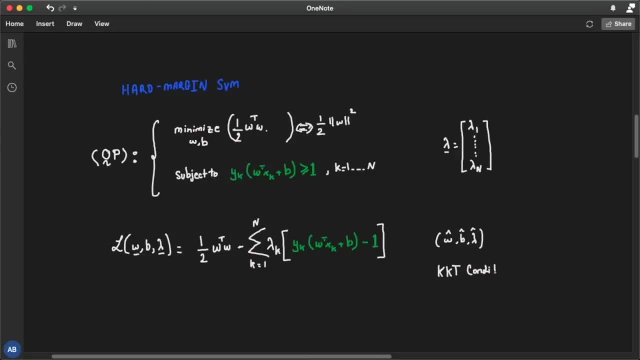 So what are the conditions that I'll be leaving down in the description section? So one we have to. the solution achieved by equality should respect the problem's constraint, That is, all yk's multiplied by w hat transpose. That is the solution. 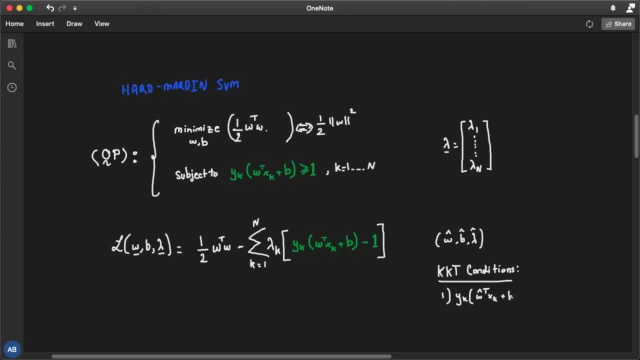 So one xk plus b hat should be greater than 1.. That's one. And two, all my lambda k hats should be positive. and three, we should have complementary slackness. And what is complementary slackness? It means that either 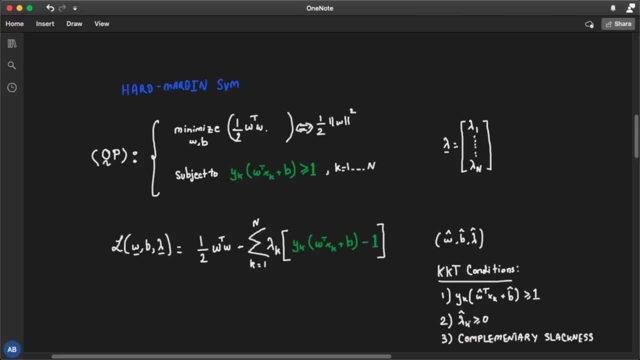 lambda k is zero or that is for the kth constraint. either lambda k is zero or the green term is zero. what does it mean that the green constraint is zero? it means that my kth instance lies on the boundary. what, what happens when this term is achieved with equality? it means that xk lies on. 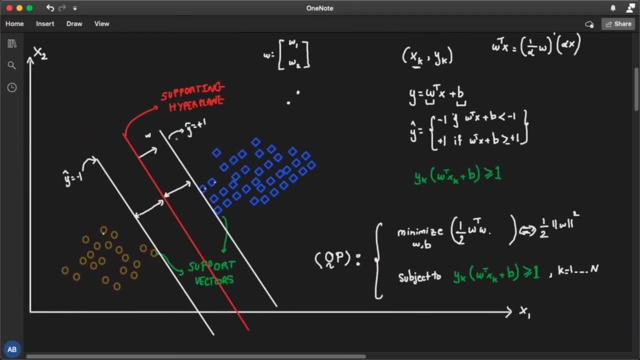 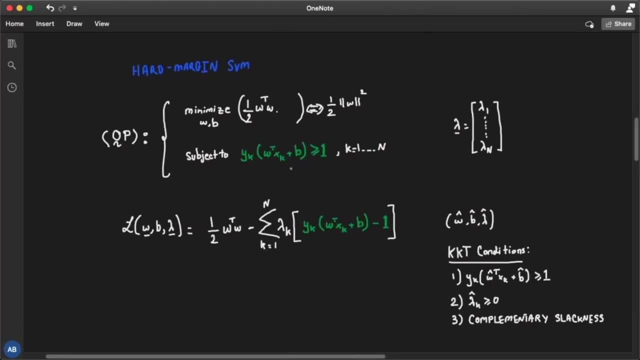 the on one of the margins right, either this line or this line, depending on the value of yk. okay, so kkt conditions give us necessary ones for a stationary solution, or point to be a solution for the constrained optimization problem. so after obtaining the solution, if you verify that, 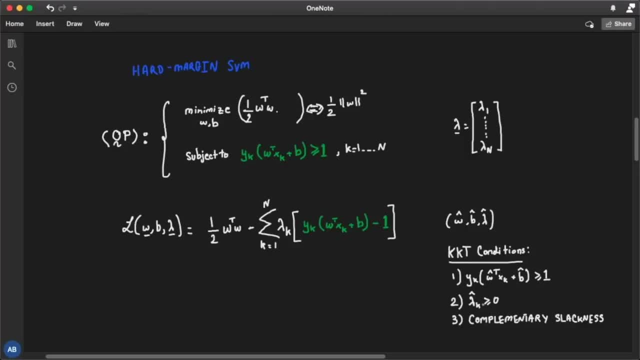 all three solutions are you achieve, that means your point is the optimal point and indeed in the svm this is the case. so let's first proceed by computing the gradient with respect to w. so nabla w of the lagrangian function. i'm going to omit, for sake of compact presentation, that l depends on w, b and lambda. so 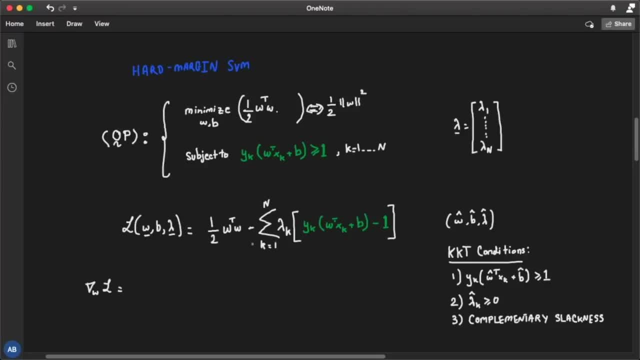 what happens when i take the gradient with respect to w. this term becomes so. when deriving, when applying a vector derivative on w, transpose w, we get a 2 w and this 2 will cancel out with this 2, leaving us with w. okay, now, over here, this term is linear. 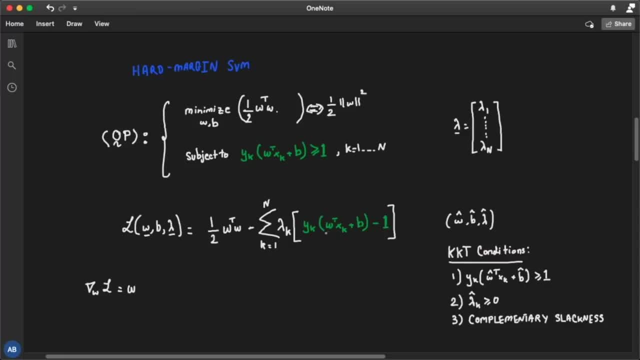 in terms of w, right. so what I'm going to to be left with is only this term, without the w, so as if you're deriving 2x, what's the derivative of 2x? x with respect to x, it's 2.. so what are the terms that are independent of w in this? 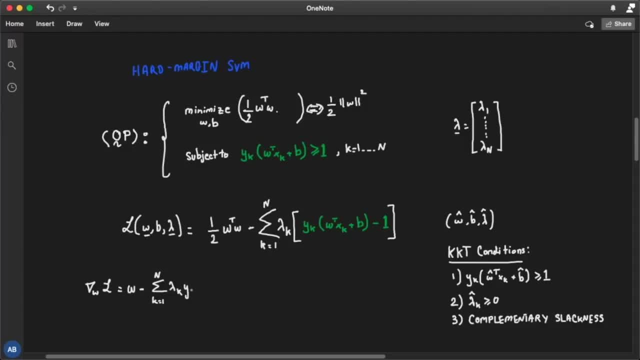 part over here it's lambda k, y, k, x, k. note that lambdas and y's are scalars and the x is a vector. okay, now let's apply the partial derivative with respect to the scalar quantity b. what do we get? we can see that the only term depending on b is the sum. on lambda k. 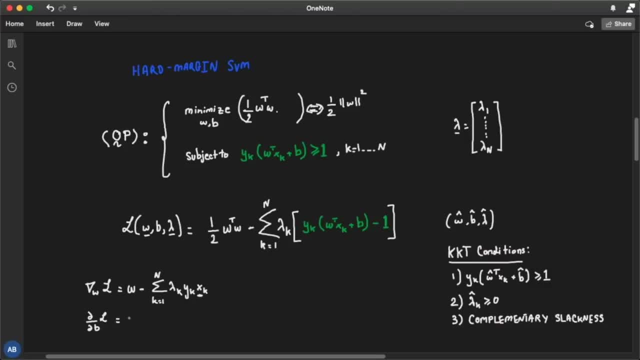 y k, and don't forget the minus over here. so we get minus sum lambda, k y k, right? so if i set both terms to zero to obtain the stationary points or point, we get that from the first order condition, the first equation. we get that. my solution of w. 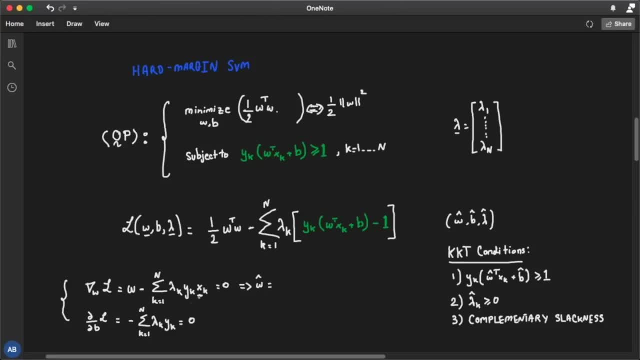 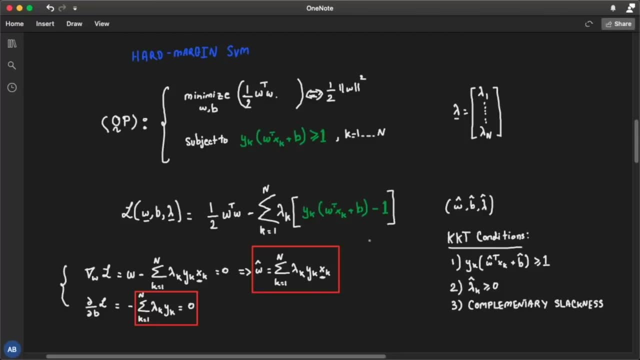 u takes the form of this guy over here. so i have both conditions w hat. that is this guy. i know my x's and y's. they're the given training set right, but i don't know the lambdas likewise over here. i get this condition over here, that is. 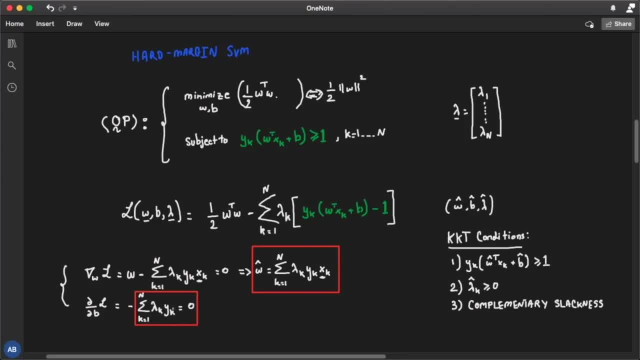 the scaling, the linear combination between lambda and y has to be zero. that is lambda vector and my y vector. if i stack all my instances y1 down to yn and one vector call it y, those two vectors should be orthogonal. that is lambda transpose y is 0. right now I have a closed form. 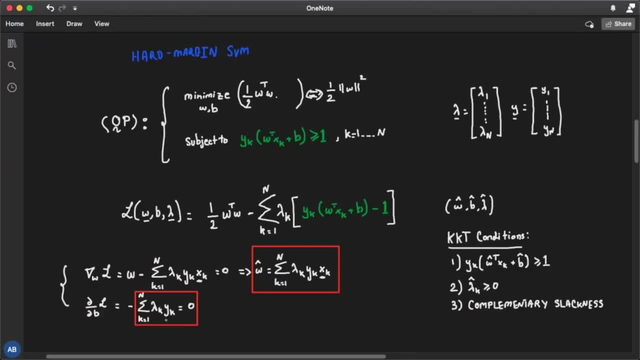 solution of W, but I don't have one for B. that's another problem. so we have two problems right now: what is my lambda and what is a closed form solution of B. okay, well, for B, don't forget that we have our good old friend, or friends, Karush and. 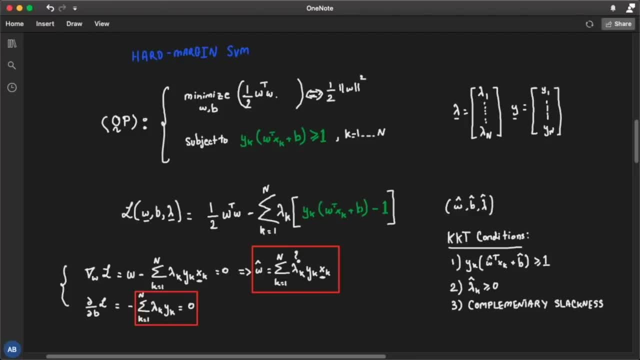 Khan and Tucker. they tell us that, okay, your solution has to respect all three lambda K. positive, no problem, I'll show you. I'll show you what I mean, why this is no problem, as well as the complementary slackness. we'll see this just in a few moments from now. but take a look at condition one. condition one: 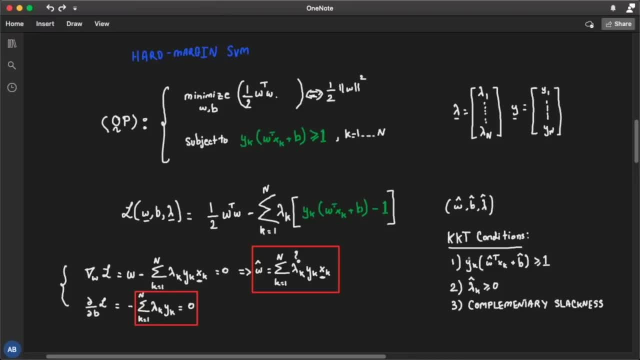 they tell us: okay, your solution is optimal as long as one, two and three are satisfied. now let's tighten one up. let's say that, okay, I'm going to solve my problem, but I'm going to solve it with equality. that is, y K into W half. 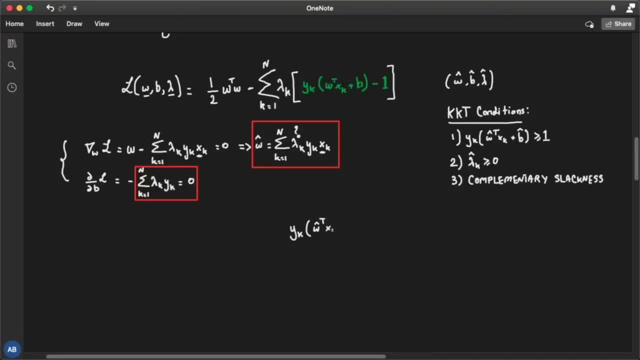 transpose xk plus B hat, which is what I'm looking for, is 1. what have I done here? I have tightened my inequality. it still satisfies the KKT, because the KKT tells me that it should it. it shouldn't be less than 1, it should be greater than. 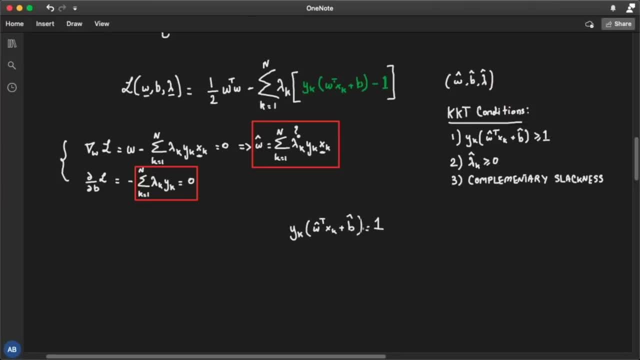 or equal. I'm going to take the extreme case, which is equal, just to find a closed-form solution of B hat. how is this helpful? Well, just express this equation in terms of B hat as a, I mean isolate B hat on one side. 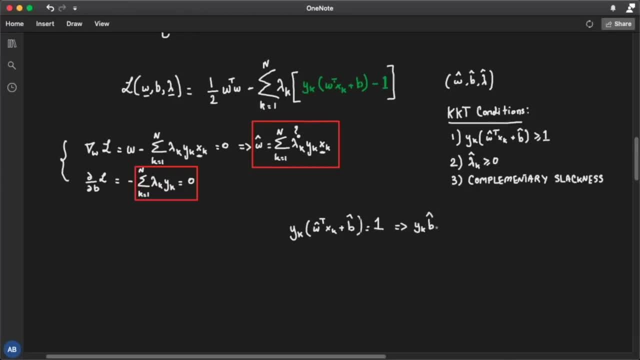 you're going to get that YKB hat is equal to one minus YKW hat. transpose XK right And there you go. So once you compute W hat, let's say you have computed W hat, you know your XKs and YKs, so you can compute B hat. 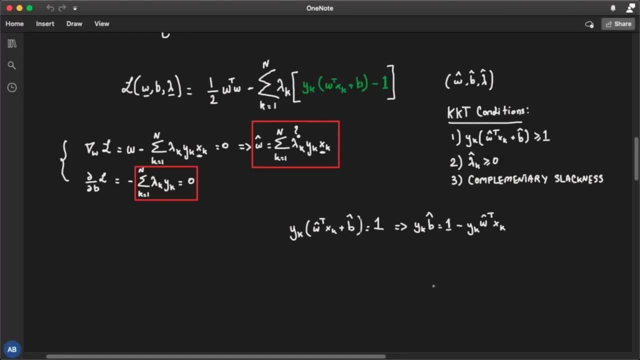 How Well to make use of all the training set. notice that this applies from K going from one to N. you can average both left and right-hand sides. That is taking the sum over YKB. YK is going from one to N. 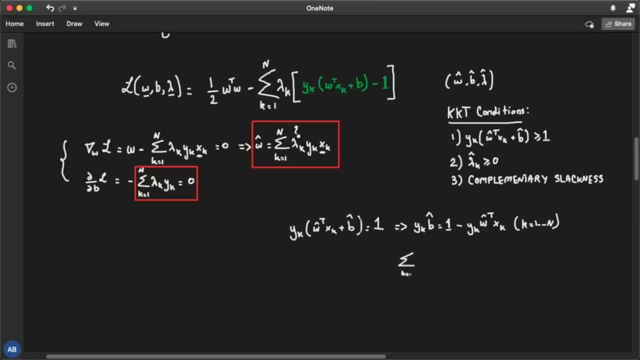 So over here you can go from K equal one to N YK, right. So one last thing over here is to notice that YK is either plus one or minus one. right Now to get rid of this YK over here. 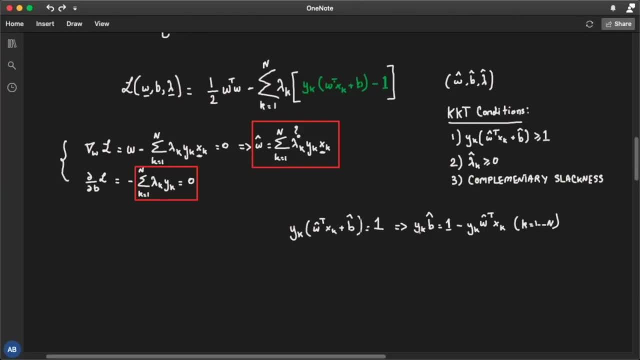 I'm not going to divide by. well, you could divide by YK. but if we multiply by YK on both sides, look what we get. So we get a YK square B hat is equal to YK minus YK square W hat, XK right. 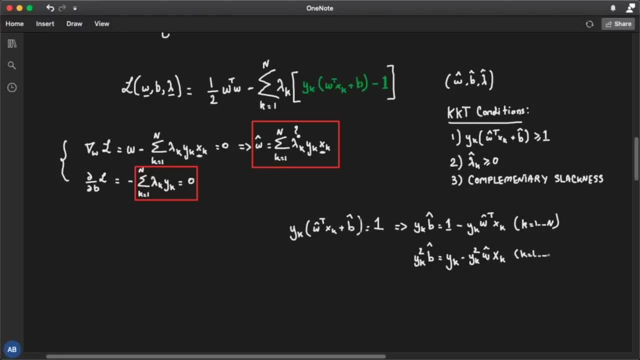 Same thing K, going from one down to N. Notice that YK square is nothing other than one, because YK is either plus one or minus one. So I get B hat. that is YK minus. I forgot a transpose here. W hat transpose XK. 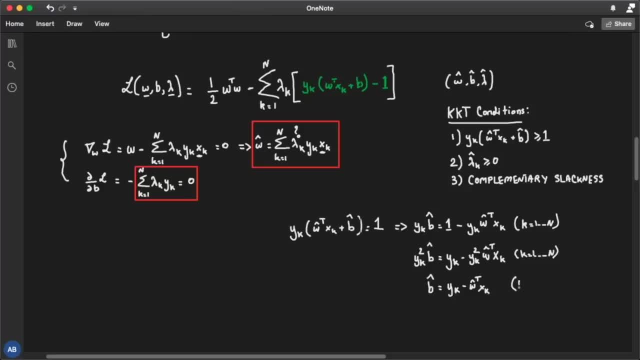 And this thing also applies for all K, going from one down to N. Now this gives you an estimate using only one training edge. Now this gives you an estimate using only one training edge. This gives you an estimate using only one training instance: XK, YK. 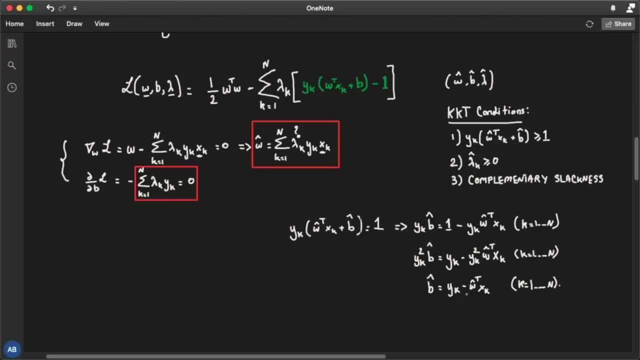 However, we can use this for all my training instances, right? So it's preferred to take an average over all such terms to robustify the quality of estimation of B hat. So for that, we're going to average over all such terms. 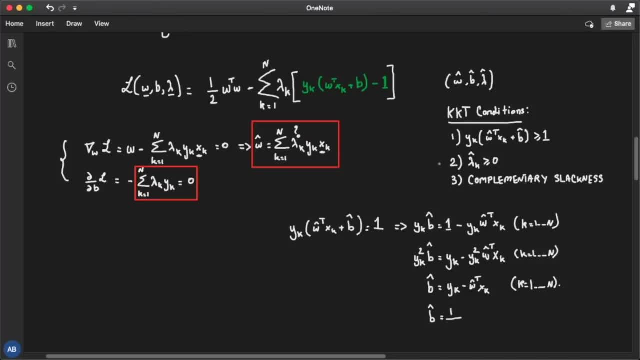 but that's where the second KKT condition comes from, right into play. we're not going to take all of them, from 1 to n. no, we're going to take the ones that give us a positive lambda k, okay. so if we denote by i don't know um, what do you want to call it? 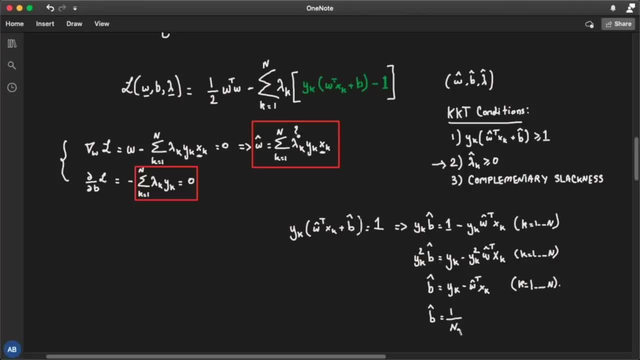 let's call it n subscript lambda. that is the number of elements or training instances. that correspond to a positive, positive lagrangian multiplier. we're going to average over all those terms. so n lambda, let's call n lambda this. i don't know the set, so this is the cardinality. 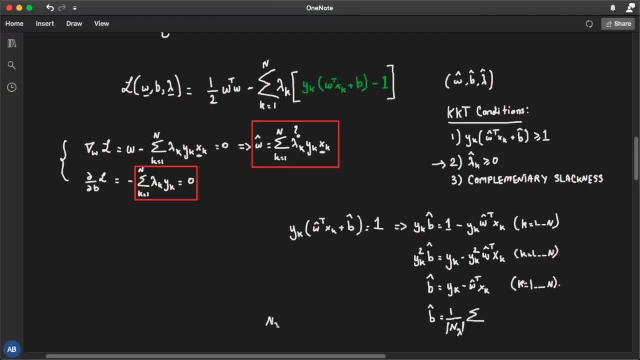 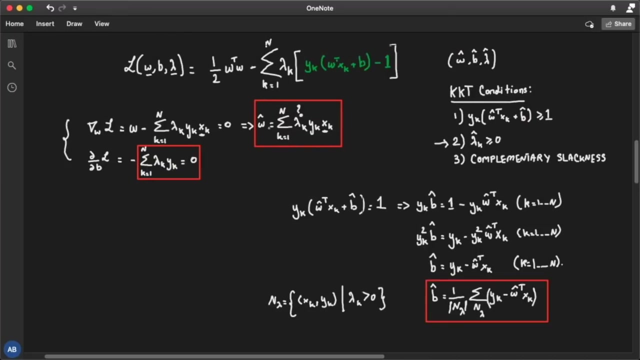 so let me write down n lambda. n lambda is the set of xk, xk, y, yk, such that lambda k is strictly positive, right, so over here i'm summing over such training instances. okay, good, okay. so now i have a closed form solution for b hat. i have a closed form solution for w hat, but 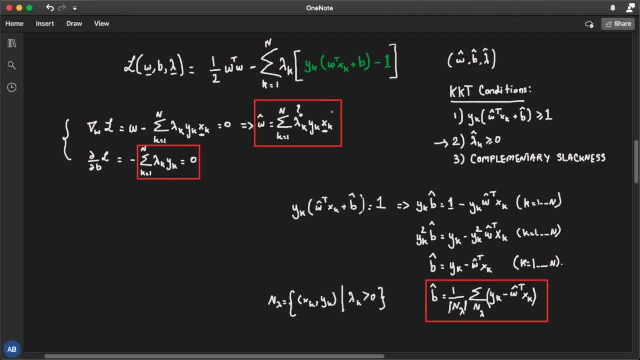 in order to compute w hat, i need the lambdas. and even more, in order to compute b hat, i need, i need w hat. so given lambda, i compute w, and given w, i compute b. so without the lambdas i can't do anything right. so how do i get my lambdas? well, if you've also been following my convex optimization, 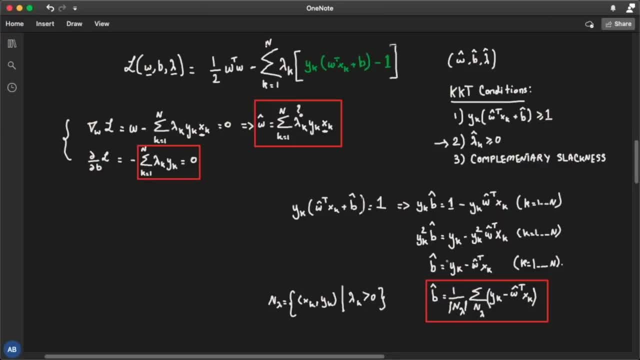 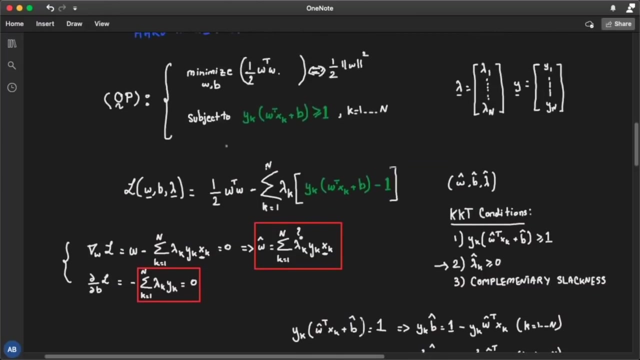 lectures, you'd see that we spent a lot of time talking about the duality concept and that for every primal optimization problem there exists only one optimization problem, and that is w hat and optimization problem. there exists a dual problem. there exists another problem that is more or less very related to the initial problem that we had, the primal one. okay, so 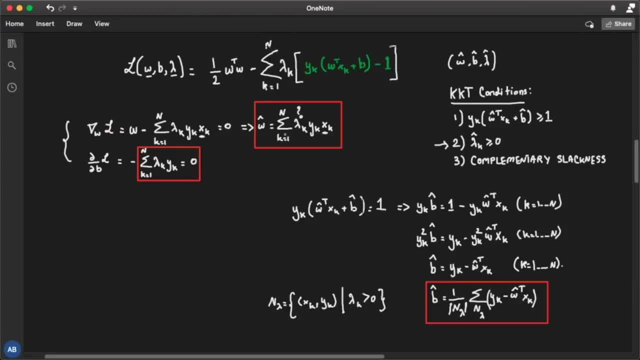 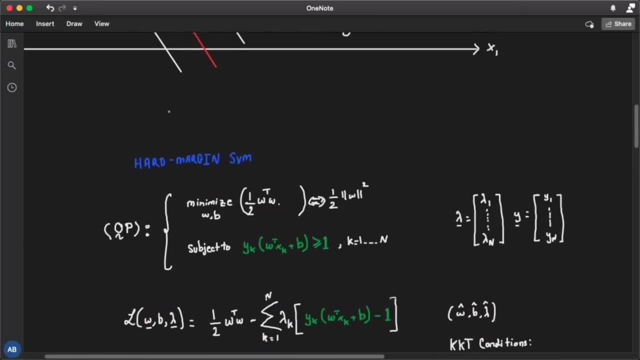 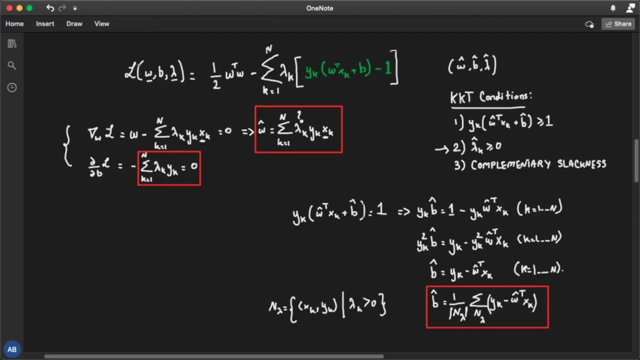 what is the dual problem? actually, the dual problem is the problem where, instead of minimizing the cost, instead of minimizing the cost, I maximize the Lagrangian function at w hat and b hat. so I'll be maximizing with respect to lambda. and actually this function has a name, it's called 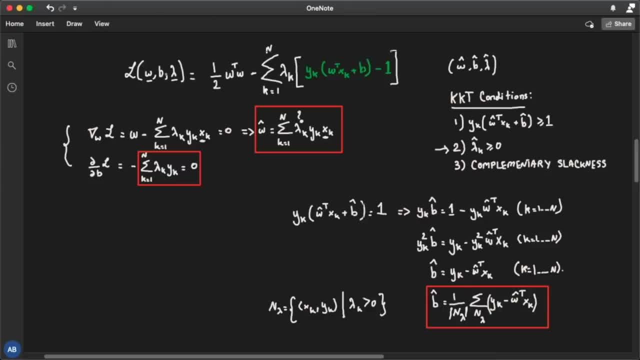 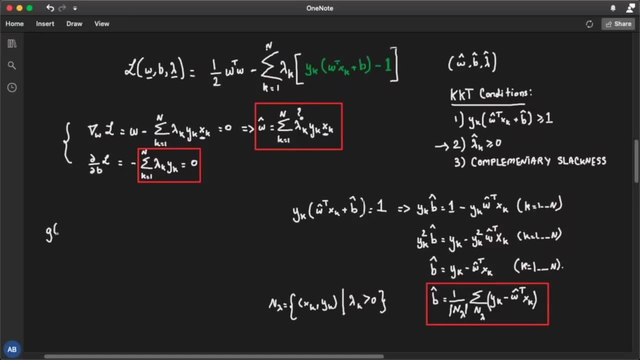 the dual function, the Lagrangian dual function, and in my lectures I denote it as g of lambda. so g of lambda is actually the infimum, but in this particular case it's the min on w and b of the Lagrangian function: l w, b and lambda. that is, l w hat, b hat and lambda is the unknown right here. 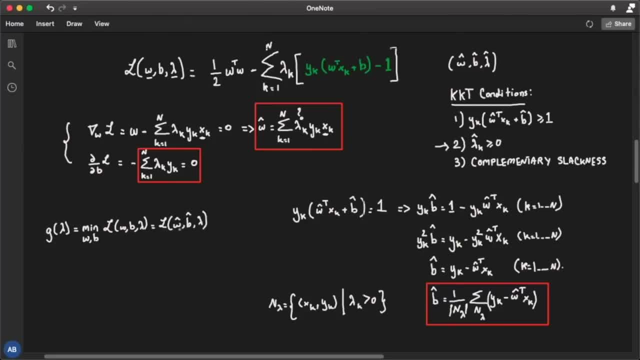 so let's find out this guy which is g of lambda. so after I found it, so after I find out an expression of g of lambda, my objective would be to maximize, over lambda, the function g of lambda subject to the second KKT condition. okay, okay, subject to positive lambdas. so this is actually referred to as the dual. 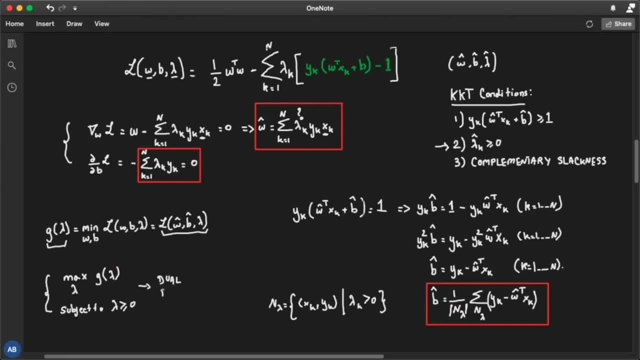 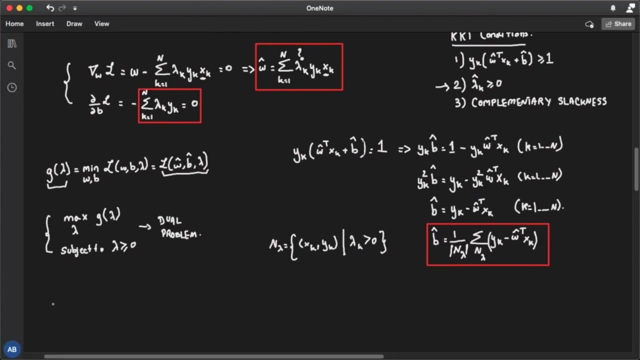 problem, and also under some conditions, the primal and dual have zero gap, duality gap which in this case is also conserved. okay, so let's find which is in this case satisfied. so let's write down an expression of g of lambda, right? so GF, lambda is the Lagrangian absolute value of the Lagrangian function. 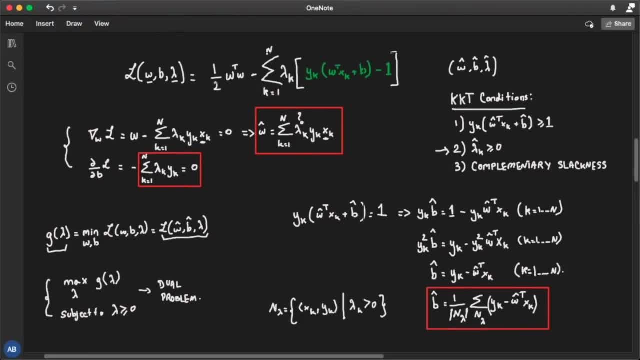 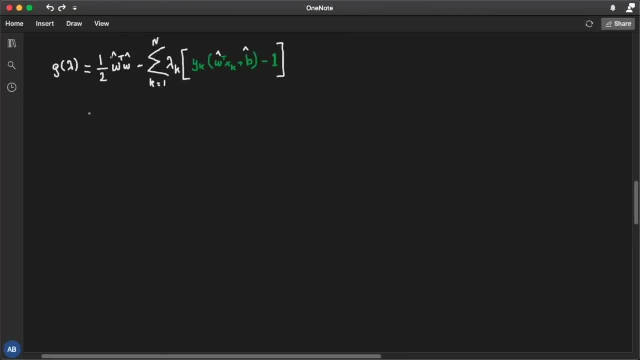 l w hat and b hat, so it's this guy at w hat and b hat, so it's this function. now let's expand this term over here. what we get is what we get is okay. so my w hat transpose times w is over here and let's expand this. we get three terms. that is the first one is lambda k. 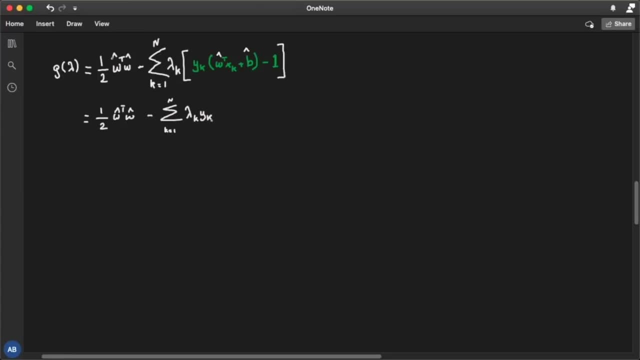 yk w hat transpose xk. the second one is lambda k yk b hat and the third one is plus a sum on lambda k right. okay, um, let's extract terms that do not depend on k outside those sums. so what we get is: w hat transpose goes outside, so k going from one to n: lambda k, yk, xk right, minus b hat into. 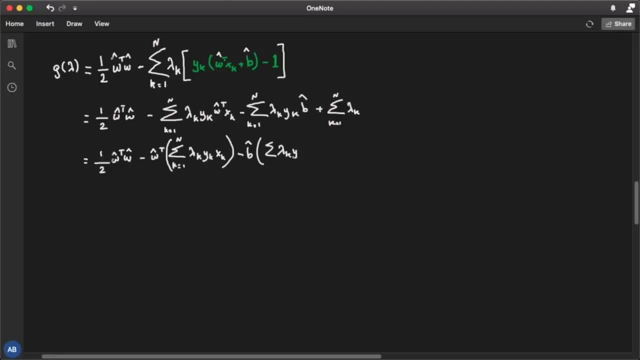 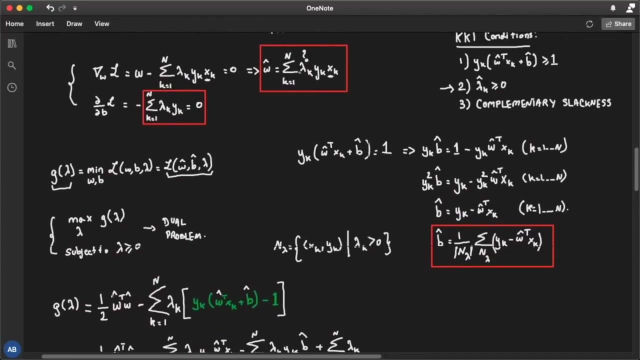 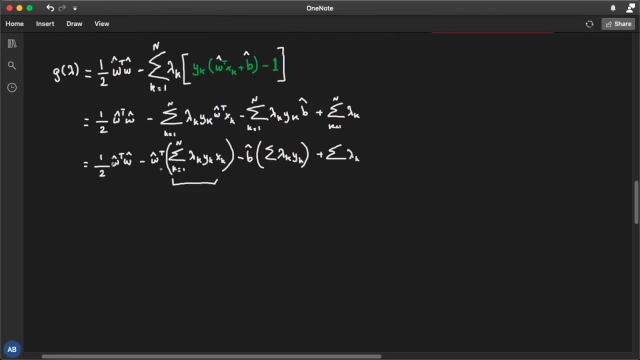 sum on lambda k? yk plus a sum on lambda k right now. what is this term over here? if we go up here, sum on lambda k yk, xk is w hat, so sum on lambda k yk, xk is w hat. so we have two terms: w hat, transpose w hat. so we've got a half minus a one. 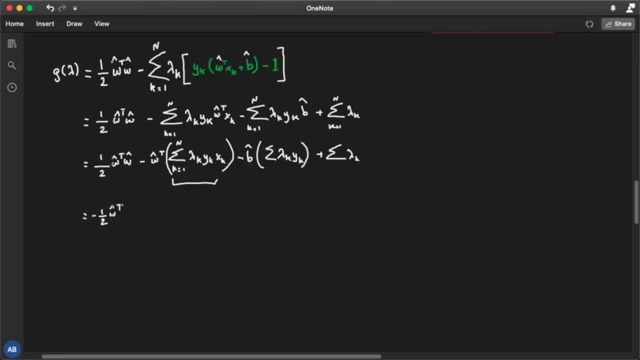 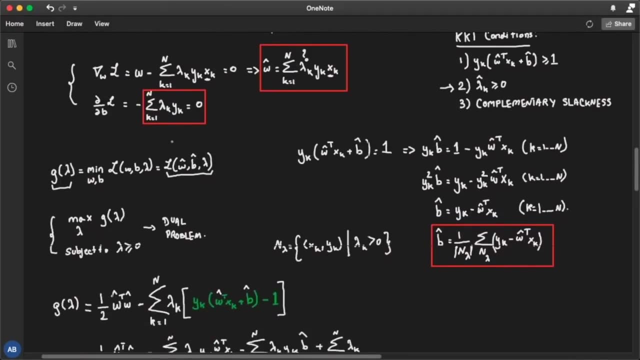 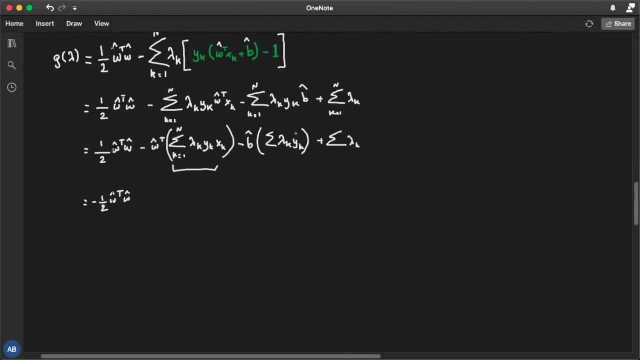 that's a minus half w hat, transpose w hat. and the third term, we have a sum on lambda k yk. well, we just saw in those first order conditions that this sum on lambda k yk is actually zero. so this guy over here is a zero and we're left with the sum on lambda k. well now, since my problem, 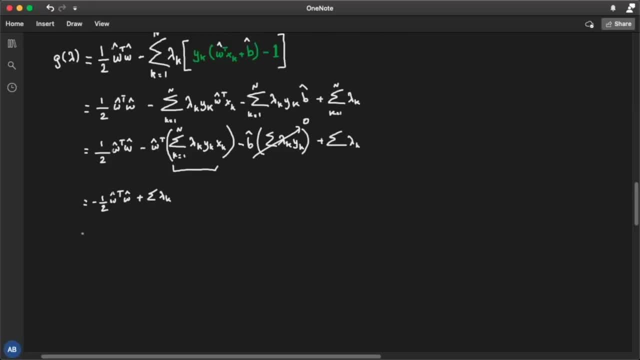 problem is to maximize g of lambda with respect to lambda. then i have to express my w hat again in terms of lambda. so i'm going to have two summations. well, since i have two summations, it's better to express each one in terms of different indices, because i'm going to multiply. 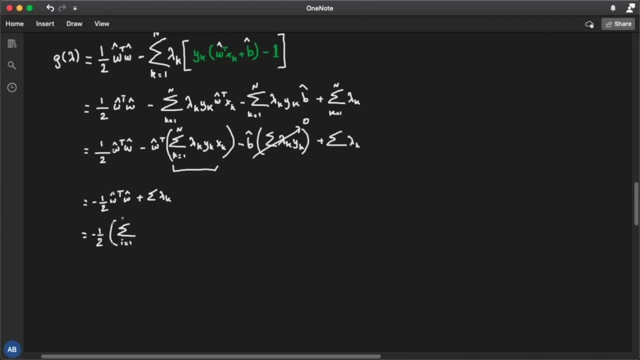 them with each other. so the first one runs on i, so lambda i, x, i, y, i. and the second one same thing, but it's running on j, right, so lambda j, x, j, y, j. then we've got a sum on lambda k. okay, let's multiply both summations to get a minus half. 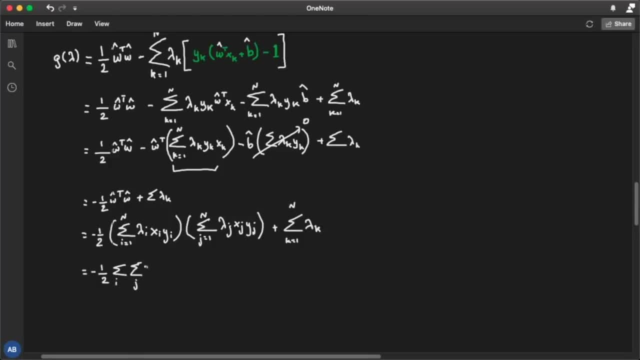 and a double sum on i and j. lambda i, lambda, j are scalars, y, i, y, j are scalars and an x i transpose. oh, i forgot to transpose over here. so x, i transpose, x, j, plus this sum over here. on lambda k: this is my g of lambda expressed in summation form, subject to: 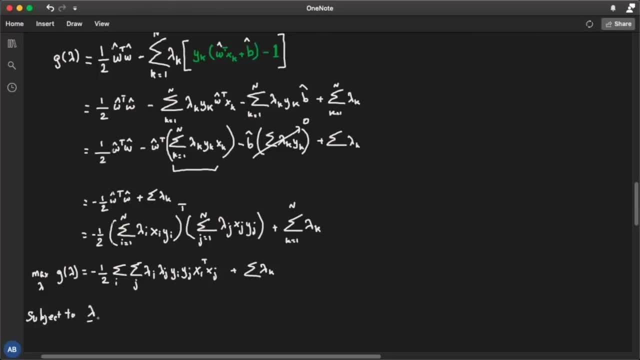 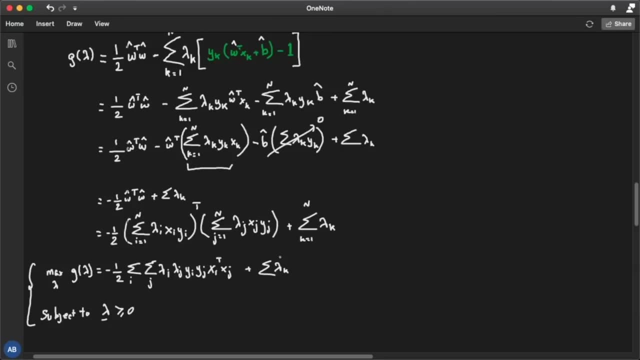 lambda positive, okay, entry wise. so we're not going to solve this problem over here in terms of lambda, because it's an easy problem. i can assure you that. um, and the way you can see it is that this guy is actually a quadratic program. is it convex? well, we have to express it in matrix form so that we can discuss that further. 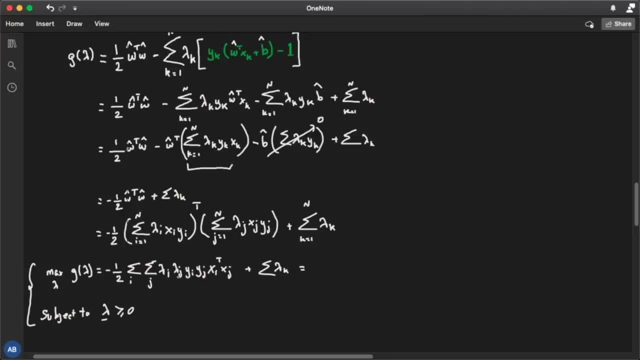 so what i'm going to do here is that we could notice that, since we're maximizing in terms of lambda, then i'm going to do a matrix form, and i'm going to do a matrix form, and i'm going to do a matrix form and i'm going to express the maximization term as follows: so we get a: 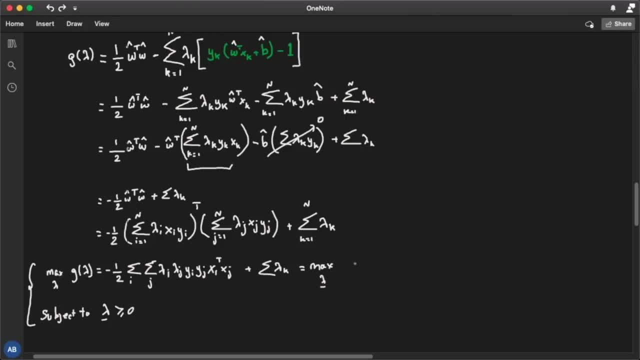 lambda transpose. well, we have a minus half, so we're actually maximizing a minus half lambda, since we have a double sum, the quadratic term over here. so it's a lambda transpose p, lambda plus. we have this linear sum over here could be expressed as f transpose lambda. let's start with the easier term, which is the linear part. so since this guy is a sum on, 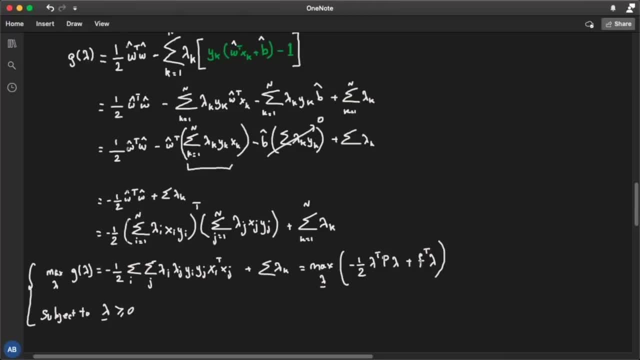 lambda. the coefficients of the lambdas are all one, so my f should be a vector loaded with all ones, right? okay, that's my f. what about my p? well, my p is a matrix, where it's i, j. let's see lambda i, lambda j multiplied by this term, so it's this term over here, so it's a y, i. 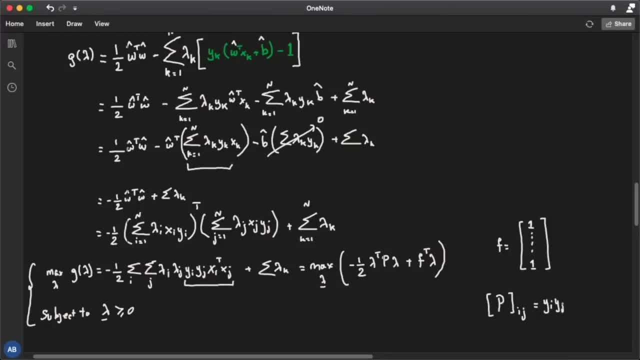 y, j right, multiplied by an x i transpose x, j, correct? okay, now let's take a, let's zoom in on this matrix and let's verify: is it symmetric? well, what is p, j, i? it is y, j, y i. x j transpose x i. well, y, j, y, i is y i, y, j, no problem, and x, j. 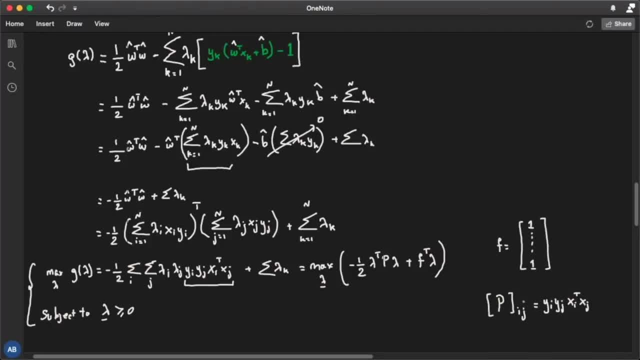 transpose x i is the same as x i transpose x j. so p i j is p j i. hence p is a symmetric matrix. okay, and the second important question is that is it. is it positive, semi-definitive? well, actually yes, it is, because you can express p. 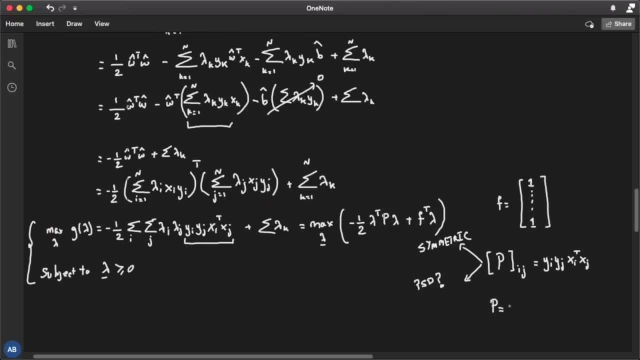 as a product of two matrices, non-zero matrices. and what are they? well, it's u. transpose u where u looks like this: u is a the m by n matrix that you know. in its first column we've got a y1 x1, y1 scalar x1. 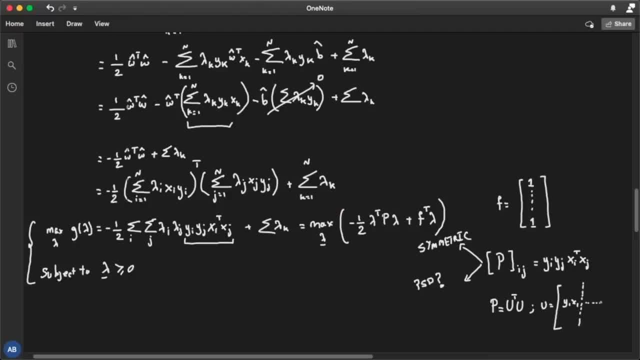 vector down till the last column, we've got a, yn, xn right. so since this matrix is in the form u transpose u, then it is positive, semi-definite. why is that? well, using the definition of positive, semi-definite matrices, for every vector, z and r, you have to prove that z transpose p, z is positive. 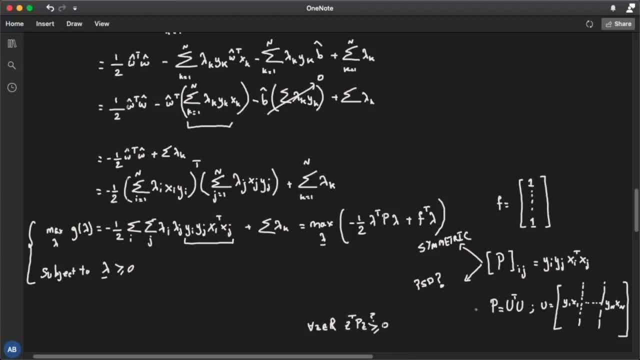 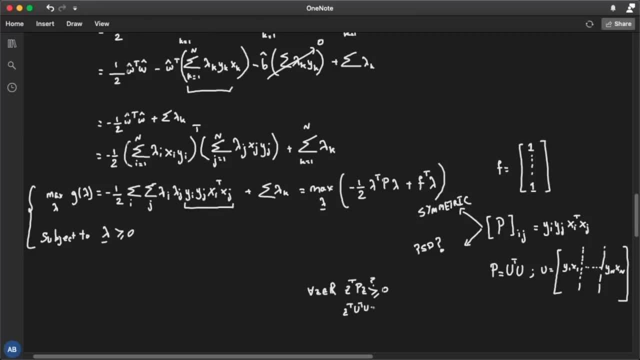 is that the case over here? well, let's plug in instead of p a: u, transpose u. we get a z. transpose u, transpose u, transpose u z. that is, u z transpose into u z. right, that is the Frobenius norm on u z, which is always: 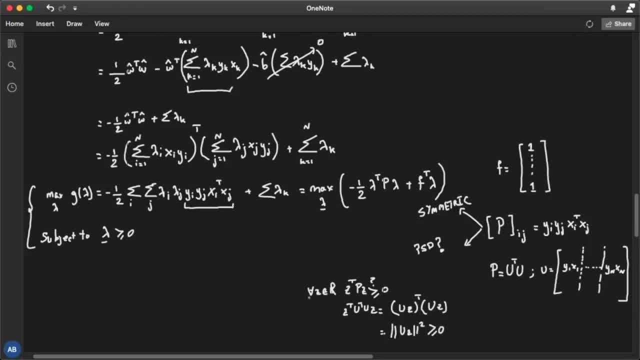 positive. so for any z, this quantity z transpose p. z is non-negative and hence p is positive, semi-definite. hence this problem over here is a quadratic and convex optimization problem which you can easily solve right. this problem is easily solved. you can easily write down the Lagrangian function of this problem. you can solve it easily. 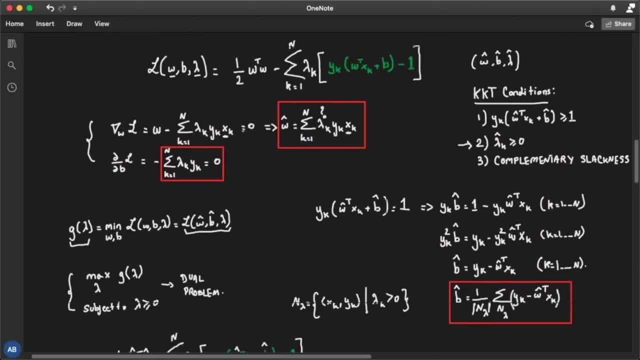 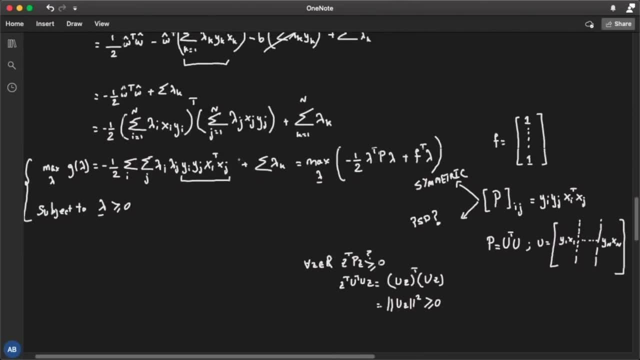 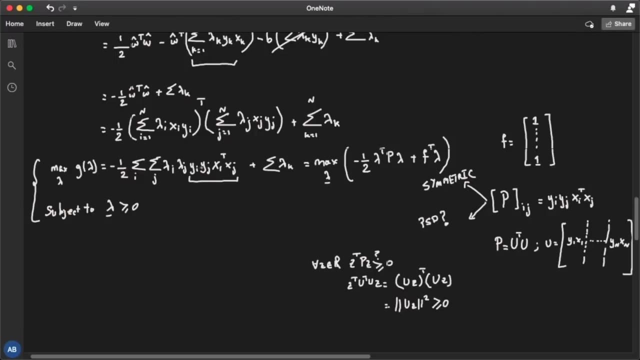 using the same recipes that we presented over here and hence, after you solve now. if you have problems solving this problem, you can kindly leave a comment down in the comment section below, and maybe you're stuck on a step. I can further assist you. maybe you want me to conduct another lecture presenting how to solve the dual problem of the SVM. no problem, I can prepare such a lecture and if not, well, you get your lambdas and once you have your lambdas from this dual problem, you go back here and you solve it using the BVM problem. 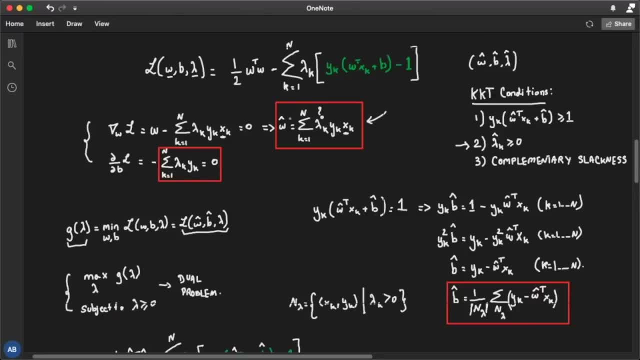 you stick them inside this equation over here. you have your w hat. that's done. you get your w hat and after you have your w hat, you go back down here, you stick it inside this equation over here and you get your b hat. and that's when you realize that you performed a hard margin: svm okay. 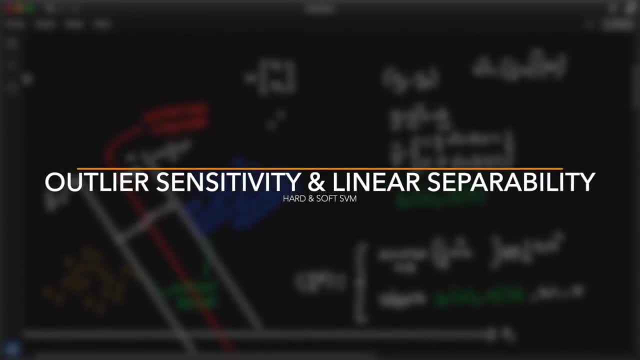 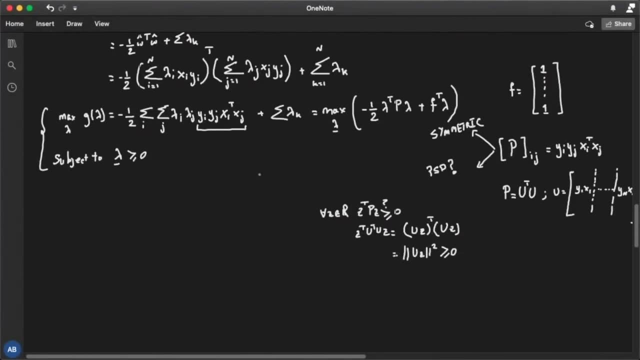 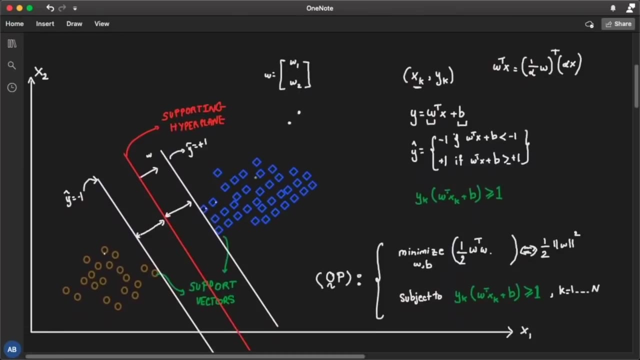 so that's how you formulate a hard margin svm problem and that's how you solve it. and that's when you notice that sometimes it works but sometimes it doesn't. and why is that? because sometimes, or most of the time, you have outliers in your data and a hard margin svm is 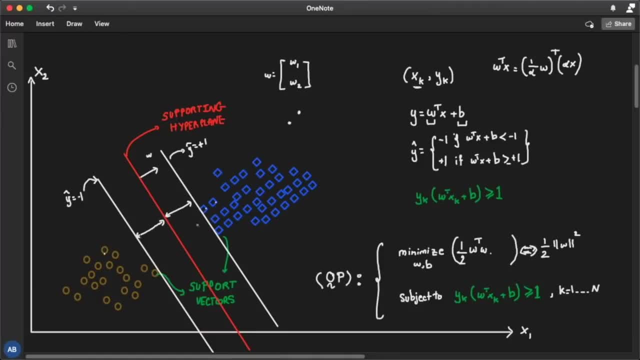 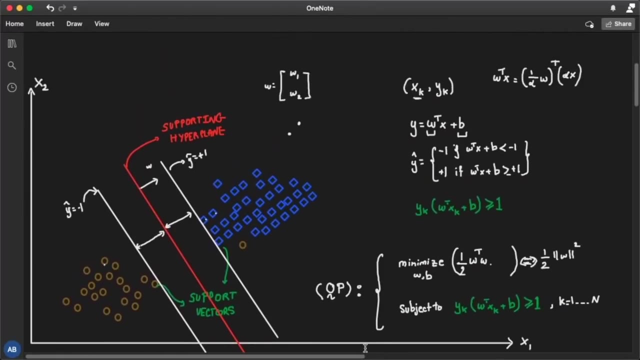 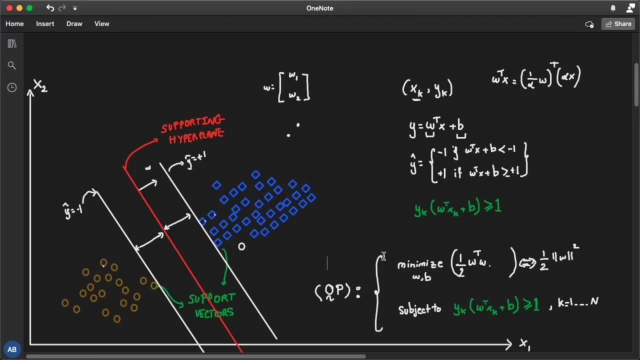 really sensitive to these kind of problems. so without. so let me show you what i mean. so, instead of let's say, let's say i've got one of those circle points right over here, right? so the first question is: well, is my data linearly separable? well, if it weren't for this annoying point right here, then yes. but this point is: 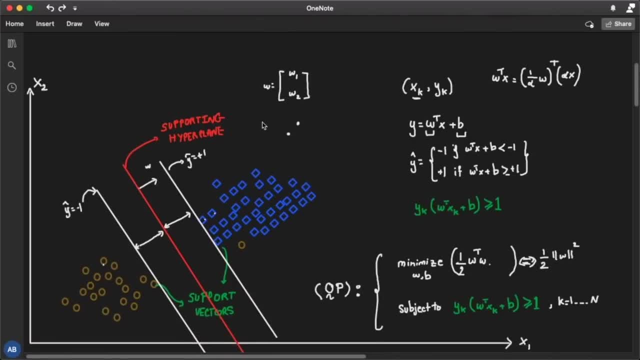 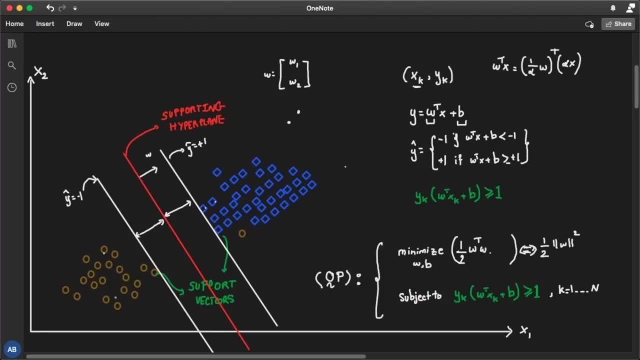 really annoying. that's what we call in statistics, an outlier. it's an annoying point and it's not an outlier. it's an outlier, it's an outlier, it's an outlier, annoying point. it's a point that you know. it's an, it's a, it's a misfit, it doesn't belong where. 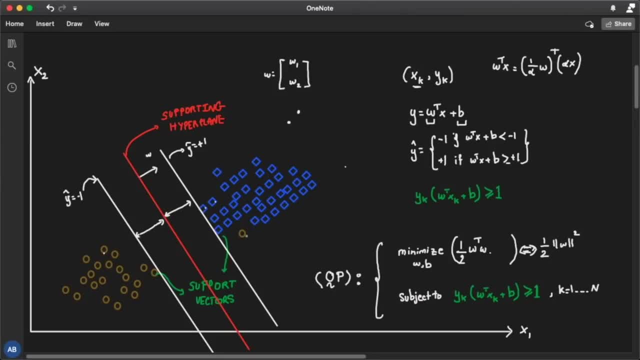 it actually belongs, okay. and that's where you have to start saying, hmm, should i take a hard decision over here or should i loosen things up? and what we mean by loosening over here is, you know, instead of placing this line over here to separate my data, what could i, you know? 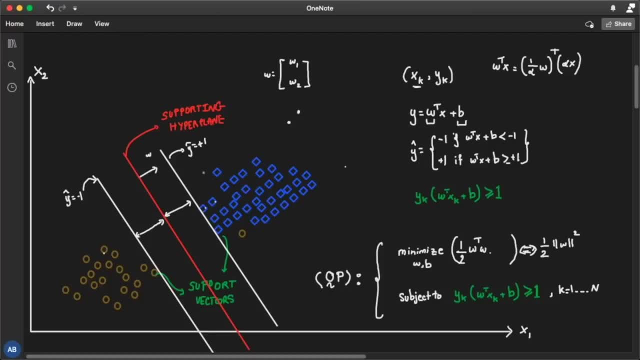 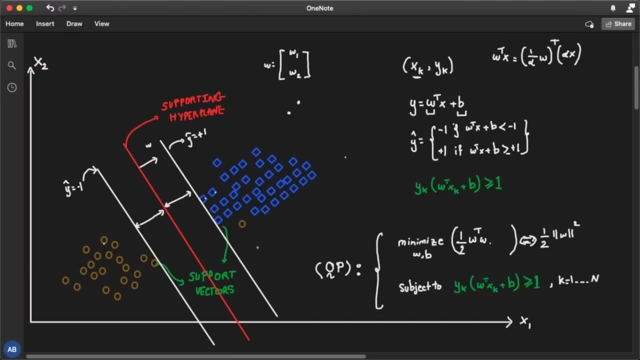 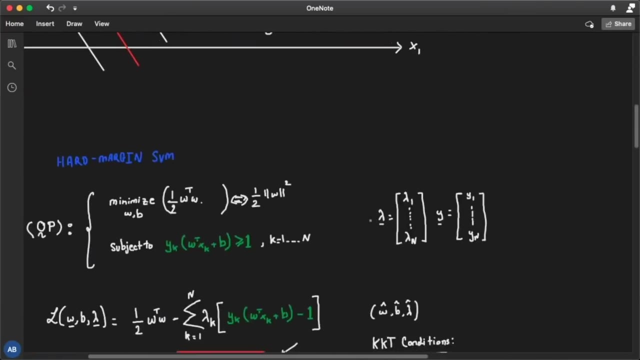 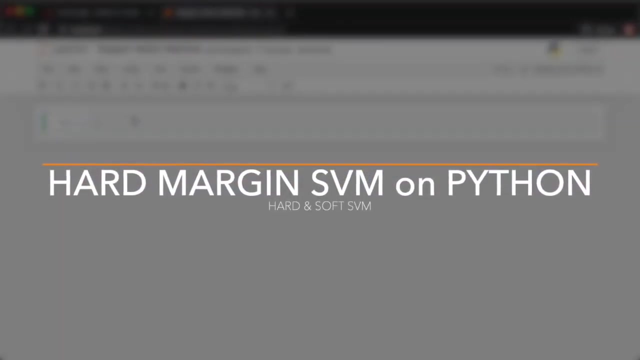 just cheat a little bit and put it over here. maybe just stick it over here. well, that's a really smart approach and that's when you can formulate another problem over here, reflecting this softness. okay, now, before now, before we get into the soft margin. linear svm. 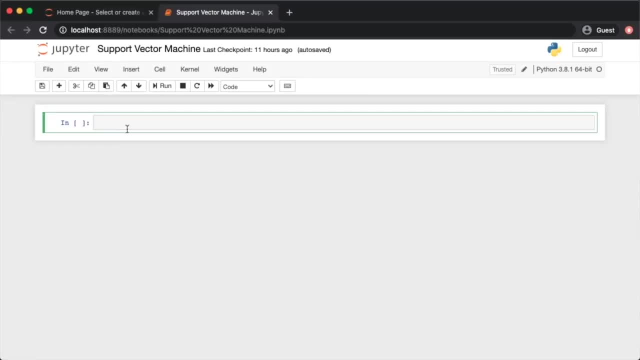 it's worth spending some time to see how to get svm up and running on your jupyter notebook on python, okay. so for that let's import the dedicated, the dedicated libraries or modules. so we need the svm classifier, svc from sk learn. i'm also going to import some data sets. 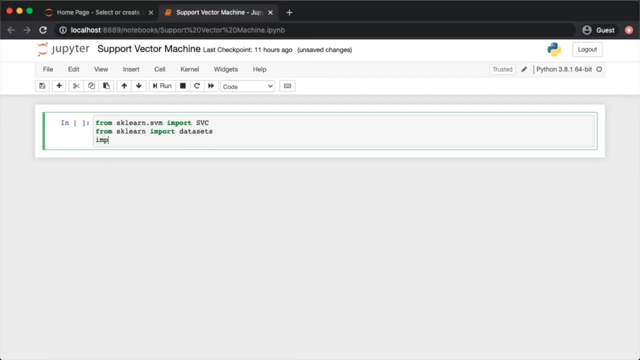 i'm going to be needing the numpy and for plotting i'll use the matplotlib in line and we'll import matplotlib as mpl and from matplotlib i'll be needing the piplot. okay, so this is a percentage, not a dollar sign. okay, so now let's import the iris data set. 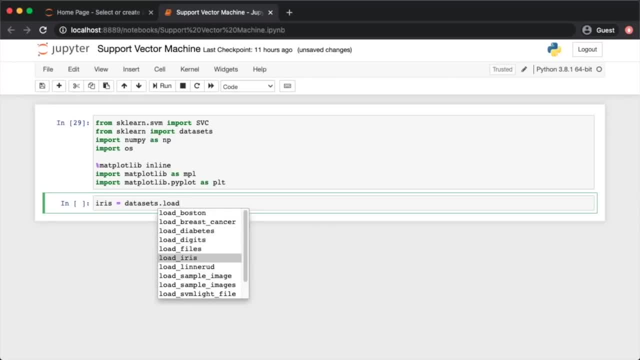 that is achieved from load underscore iris as such, and my training dataset would be irese as such. as such, because my training dataset would be iris as such- more Messing- and as such, my training dataset would be iris as such- more Messing data. let me see how this looks like X. so we need the length and the width, so the 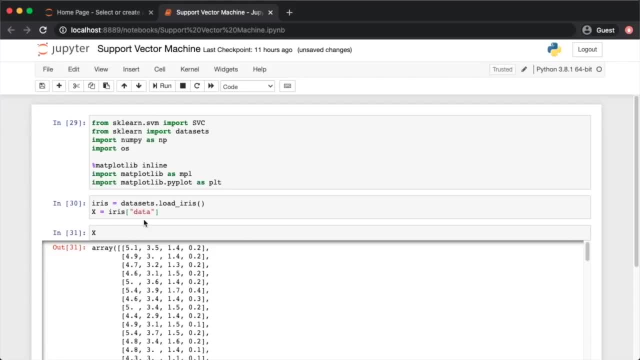 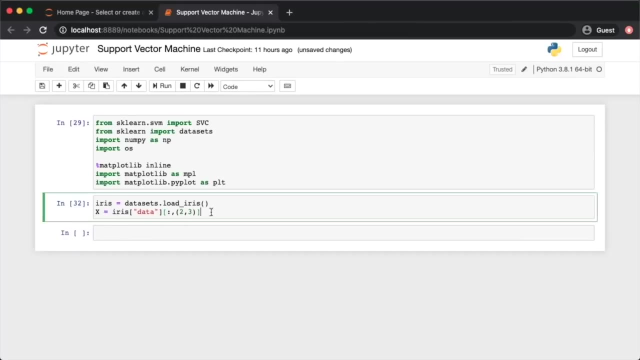 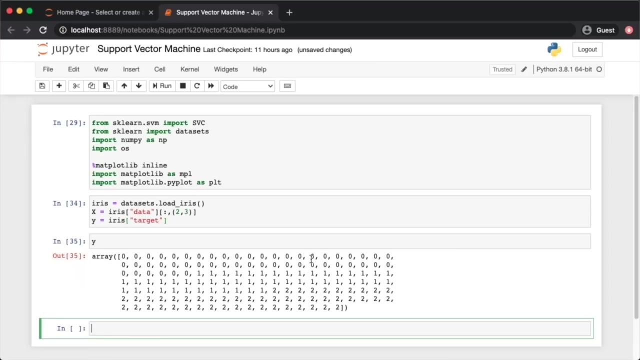 first and second columns are length, petal length and petal width respectively, so I can extract them as such, right? okay, and I will be extracting the target values, the Y's. okay, this is my Y's now, as you can see, I have three classes. I'm 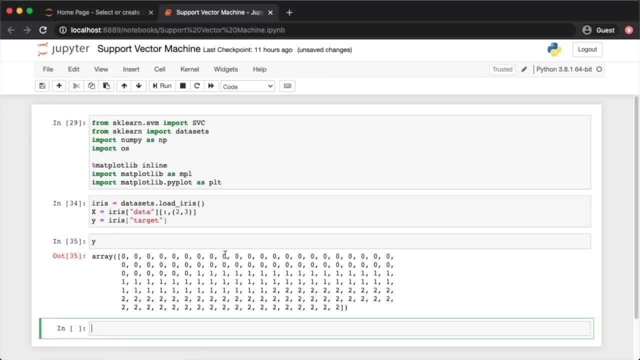 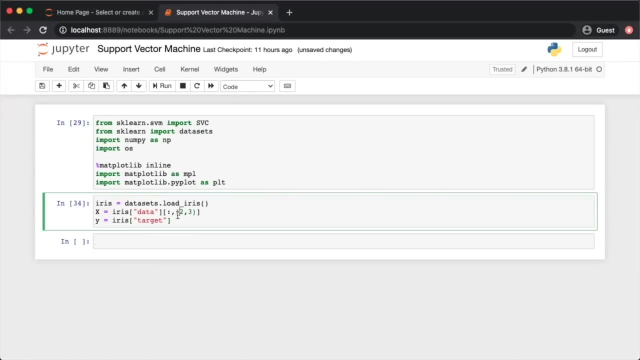 only going to be interested with binary classifications, that is, I'll pick the Y's that are either 0 or 1, and that could be achieved as follows: so 0 is setosa and 1 is versicolor. so Y equals 0 or Y equal. 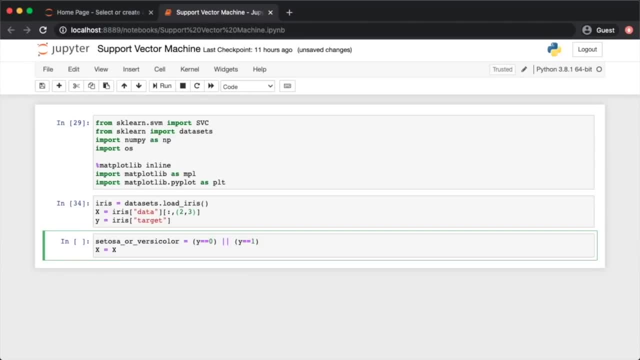 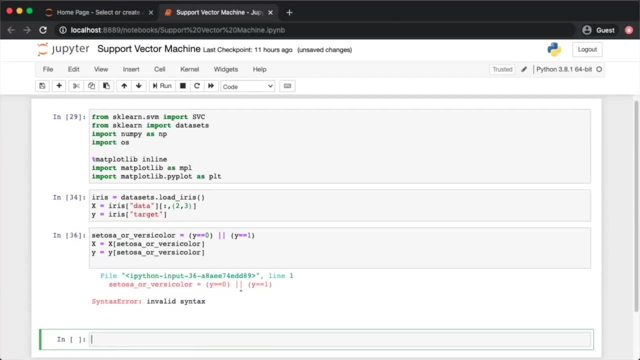 to 1, I'll extract the X's that correspond to those indices and their associated target, as well as their associated target values. oh, so this is not C++. so this is not C++ and I need one pipeline as such. okay, now let's define an svm classifier using the SVC. I'll 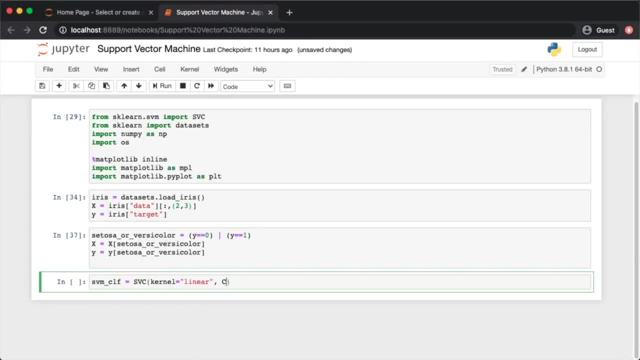 a kernel that is linear, and we'll specify the C hyperparameter, which we'll be seeing in just a while from now. when we talk about the soft margin, for the hard margin we set it to infinity. okay, so let's fit Y versus X, and there you go. 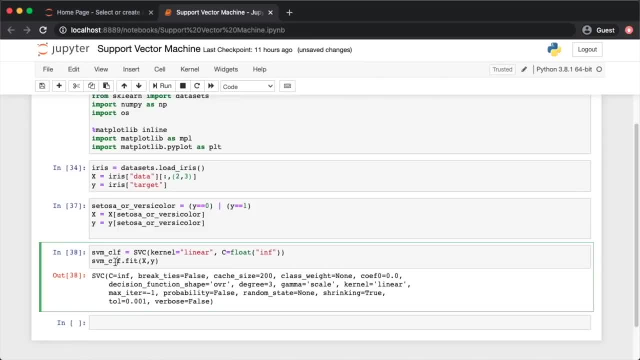 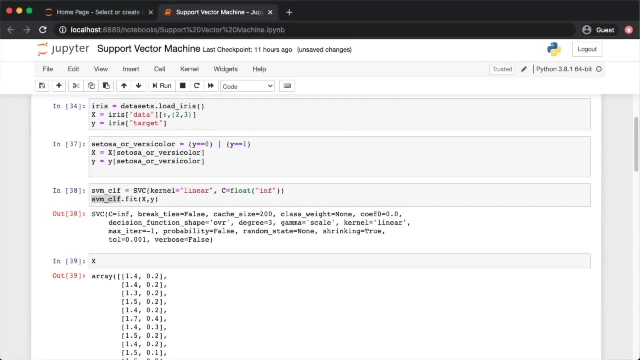 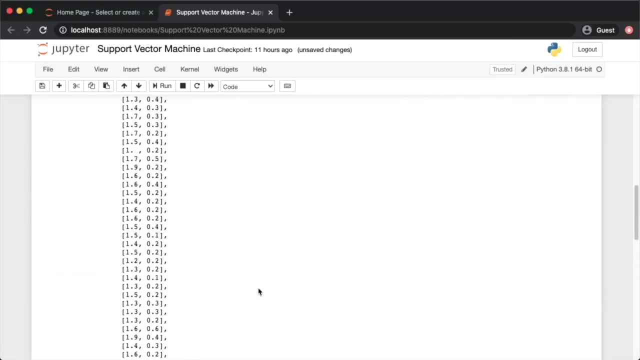 we have our SVM ready and the SVM underscore classifier, or CLF. okay, no, so now let's define an X 0 or an X axis. so let me see the range of my X's. so one point four, zero point two, four point five, no more than five and no less than. 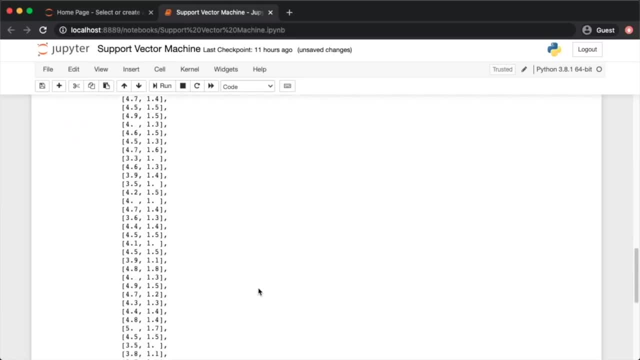 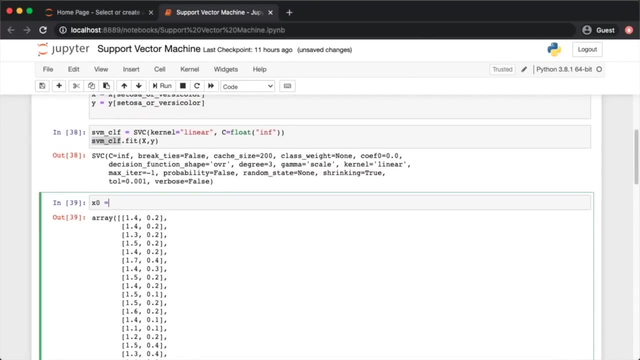 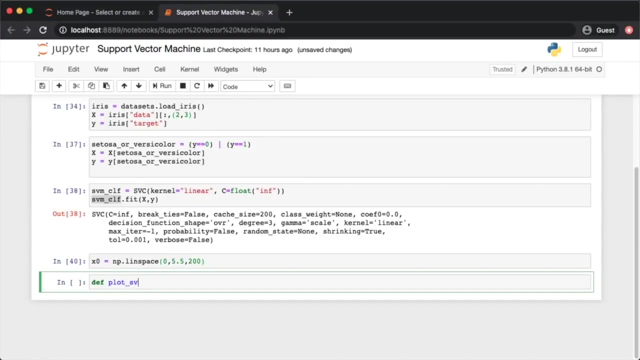 zero, right, is there a five? yeah, there's a five here, so I'll go for five point five as max. so let me define an X axis that is X: 0, going from zero to five point five, and I'll take two hundred points. now let's define a function that will plot my decision. 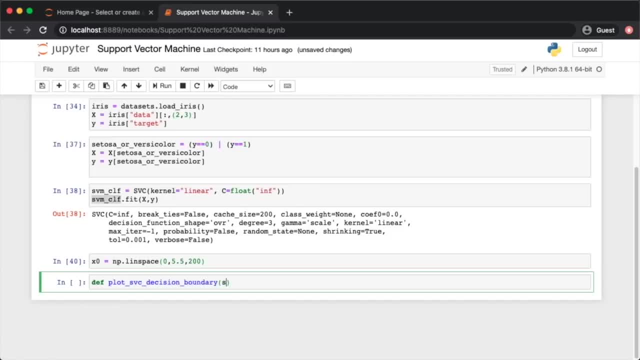 boundaries. okay, I'll pass it the SVM classifier as well as Xmin and Xmax. okay, so my W is actually stored in SVM, underscore CRF dot coefficient as such and my B is the intercept. now, at the decision, I'm going to have to plot the W transpose X plus B. okay, so. 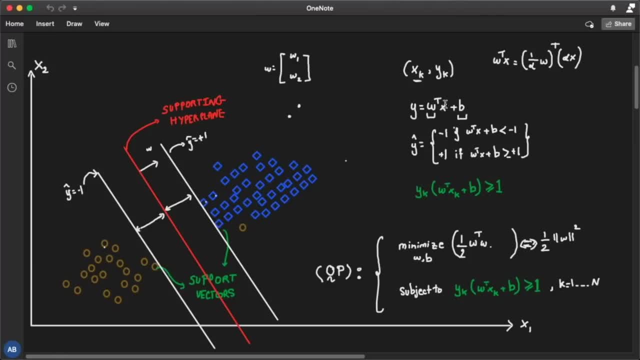 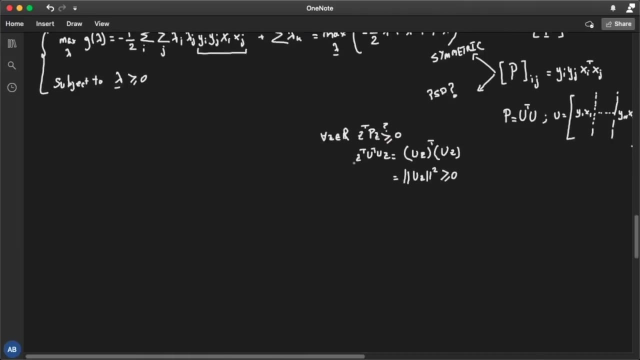 since I'm dealing here with two features, right? so X is X 1, X 2 and W is W 1, W 2, then this guy could be written in this particular case as: so if I start my indices as such, let me go down here. 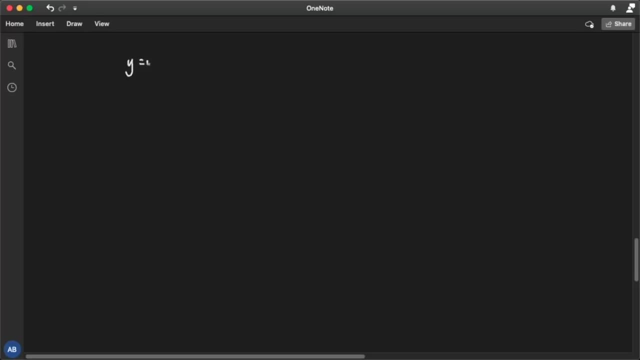 to make me some space. so if my Y is W, transpose X plus B and my W is W 0, W 1 and my X is also X is 0 X 1 and I can express this as W 0 X 0 plus W, 1, X 1 plus B and add the decision boundary: this guy is 0, so I'm 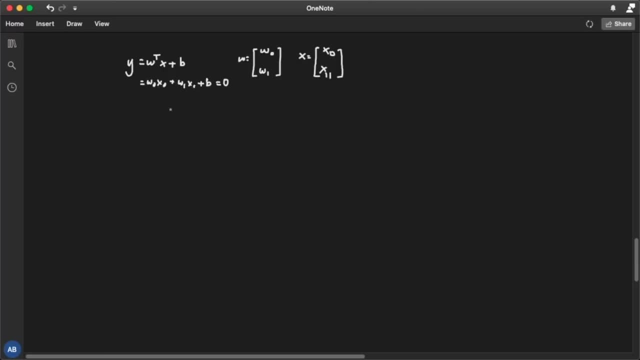 going to express X 1 as a function of X 0. how can I do that? well, that's easy. W 1 X 1 is minus W 0 X 0 minus B. right then, I divide by W 1 X 1 plus B and I: 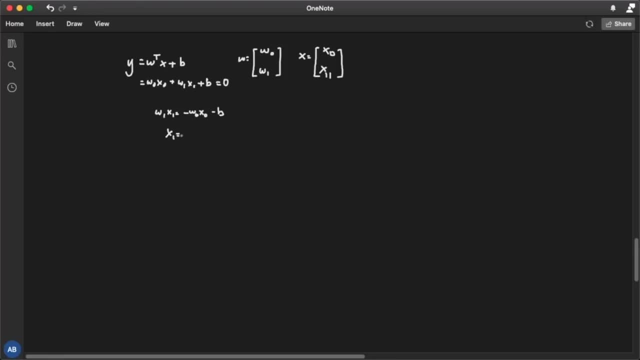 divide by W 1 X 1 minus B, right, then I divide by W 1 X 1 minus B: right, then I get an X 1 that is minus W 0 over W 1 X 0 minus 1 over W 1 B. so I need this. 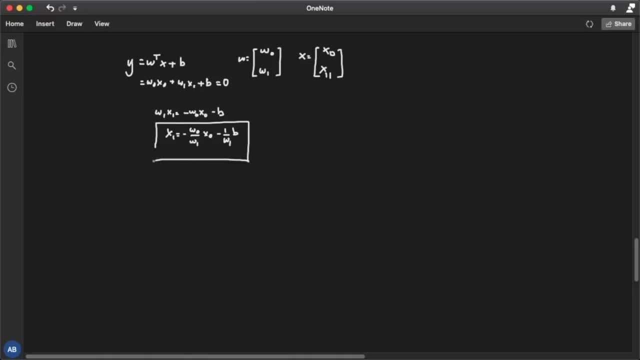 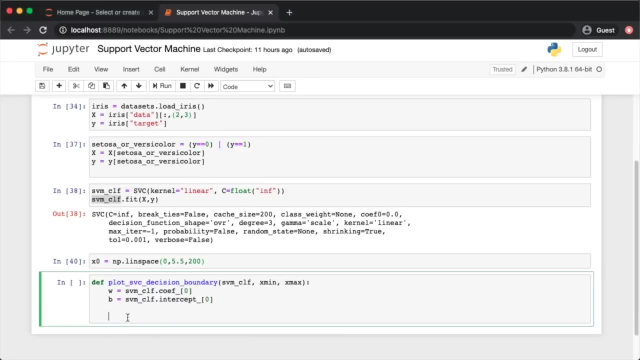 equation over here, right here. so that's what I need to you know generate. so, given what I need to you know, generate. so, given my X min and X max, I'll generate another X zero going from X min, X max. take 200 points. 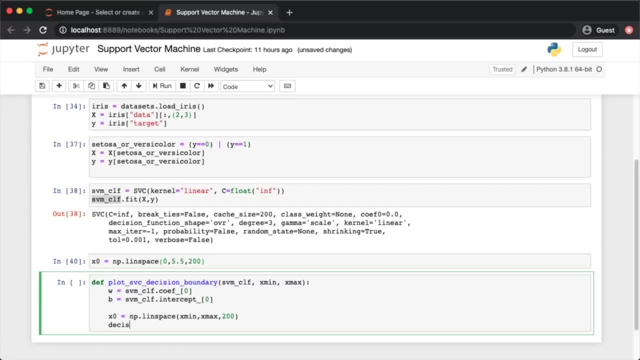 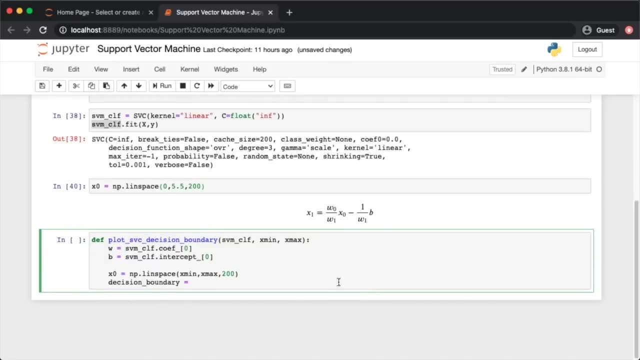 And then I'll get my decision boundary right, Which follows the following equation: So it is minus W, zero over W, one times X, zero. minus B over W, one right. And well, what is my margin over here? That's a good question. 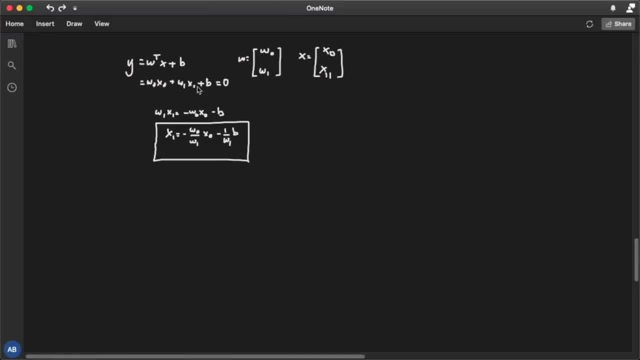 Well, it is, when it is when the same term is instead of zero, it's evaluated as one. So it's when W zero, X zero plus W one, X one plus B is one right. So expressing X- one is a function of everything else. 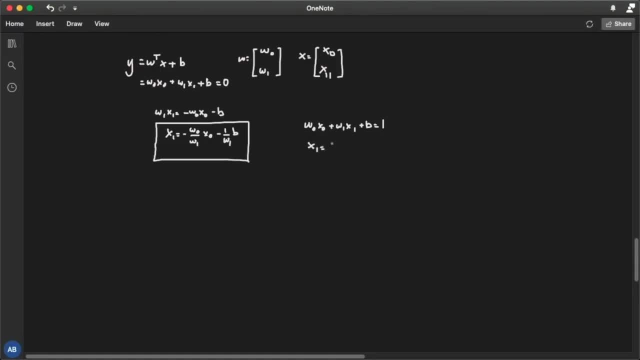 We get that X one is one over W one right Minus W zero over W one. X zero minus one over W one, B. So it's the same term plus a one over W one in case we're on the upper margin And it's a minus one over W one when we're on the bottom. 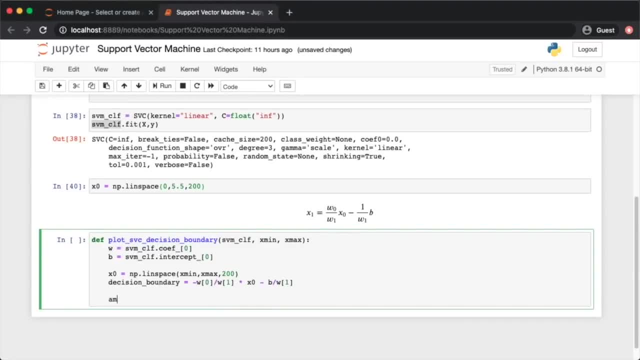 when we're on the bottom margin. So let's take this margin, That is the additional term, one over W one, So one over W one, and define the upper and lower margin. So upper margin is the decision boundary plus the margin and the lower margin is the decision boundary. 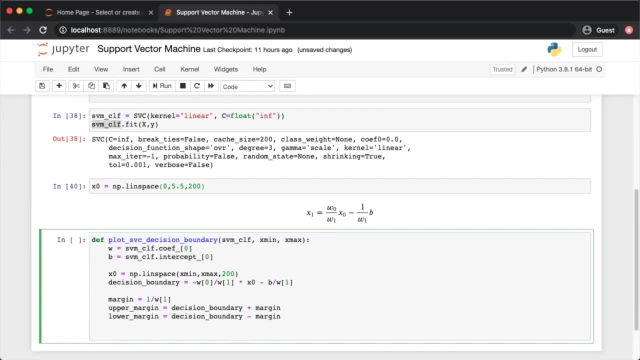 minus that margin. right Now let's take the support vectors that are SVM, underscore, CLF, dot support vectors- right. Let's plot a scatter plot containing the support vectors first component versus the second component, And let's specify some fancy face colors. 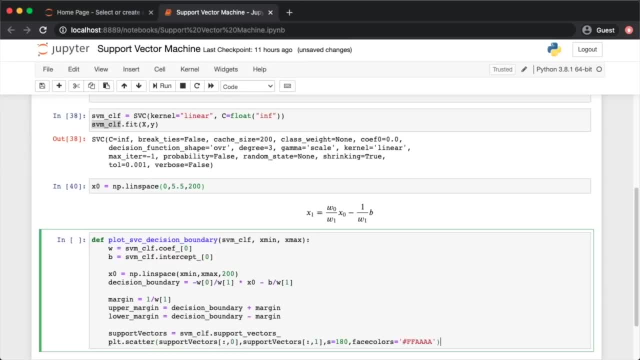 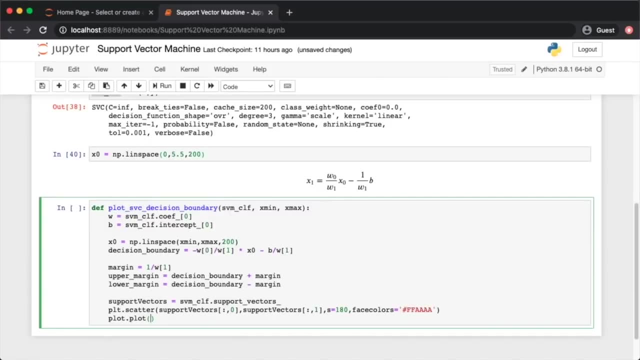 So let's enter the following hexadecimal color code. Now let's plot in the three Boundary lines. The first one is the decision boundary. I'll plot it in black. The second one is the upper margin. I'll plot it in dashed black. 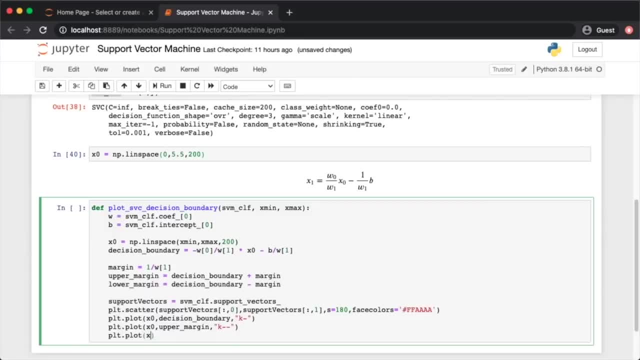 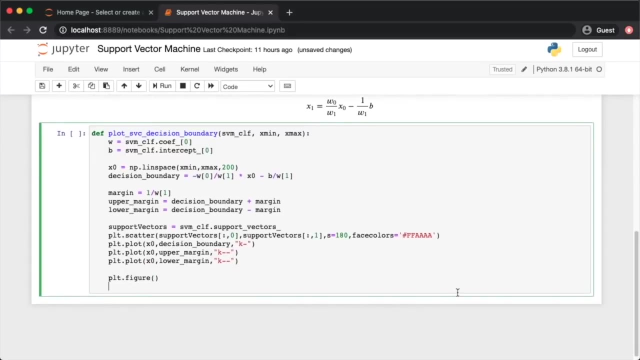 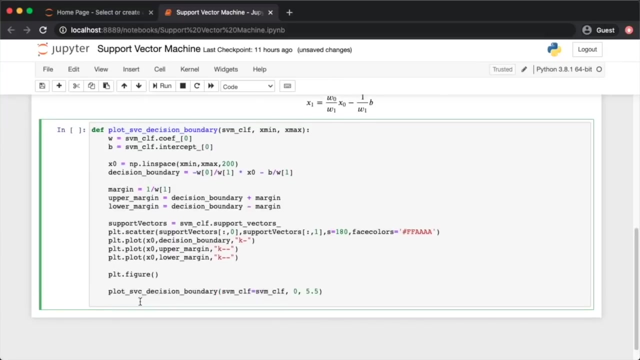 And the last one is the lower margin That I'll also plot in dashed black. We'll open a figure And on that figure I will call this function right, Pass it my classifier and my X min and X max. So X min is zero, X max is 5.5.. 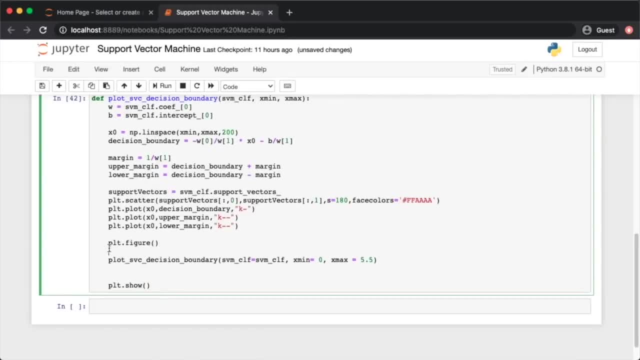 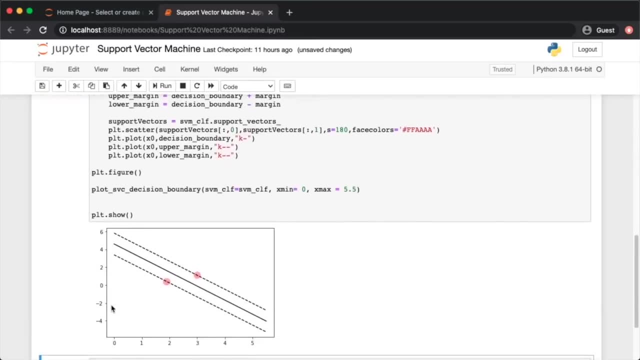 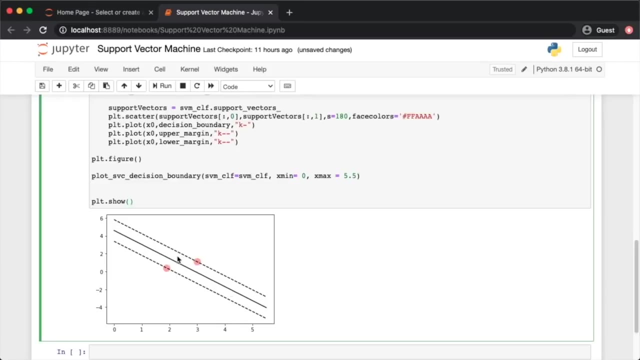 Let me see how the figure looks like. Oh, I'm still in setup. You should be careful when indenting as such. Okay, So that's what I'm plotting right now. I'm plotting the decision boundary, the lower and upper margins. 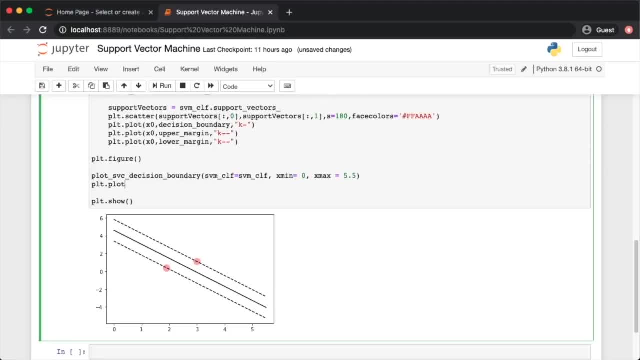 Now let's plot the data set. So the ones for one, two, three, four, five, Y equals one, I'll plot in this color, And the ones for Y equals zero, I will plot in another color, So in yellow circles, and the first one in blue squares. 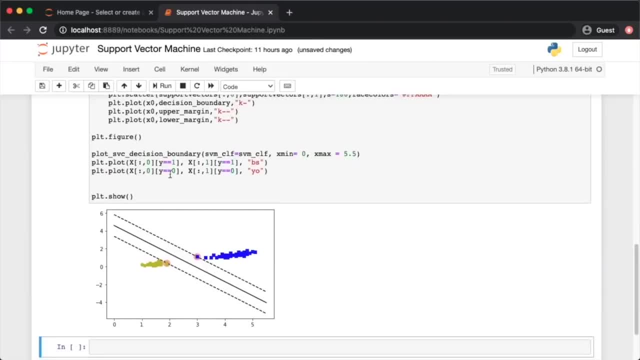 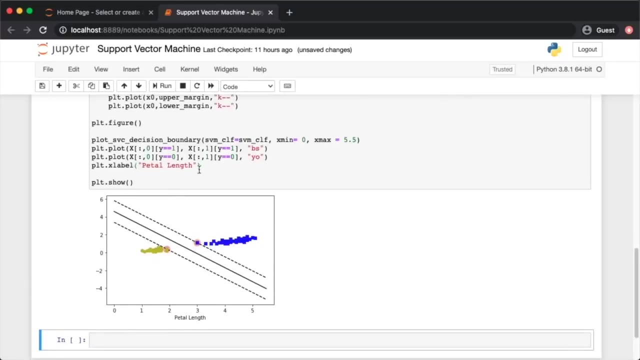 Let's see how the plot looks like. Okay, Not bad. And let's give an X label, call it petal length As such, and let's limit our access to zero- X min and X max Y min, And I'll also add the parameter with the max value. 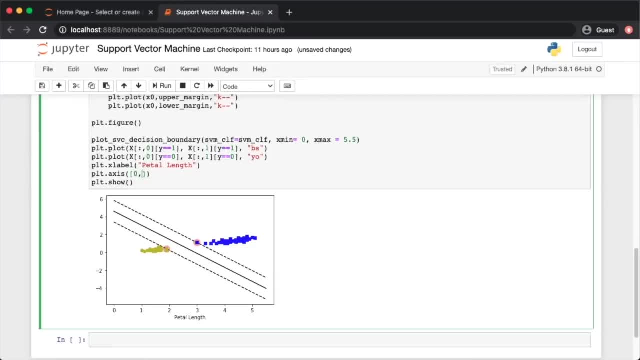 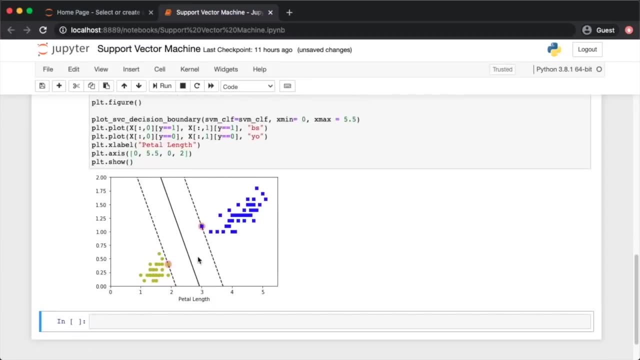 Only the max value is equal to zero, Or the max value of the input, And that's it. So the first thing we're going to do is to set this value, Okay, and Y max. and there you go. so, as you can see, SVM grabs the support vectors, passes. 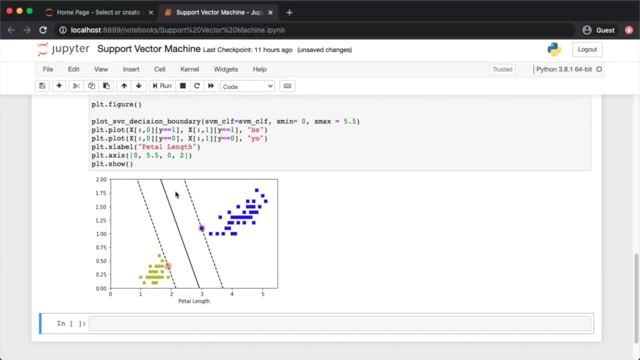 the margin boundaries and then fits in the decision boundary, so so that any arriving point is tested, whether it lies on top or on the bottom of this decision boundary. if it's on the top, it's a blue square. if it's on the bottom, it's a. 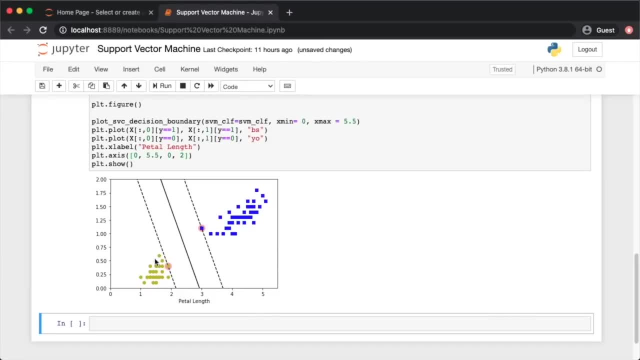 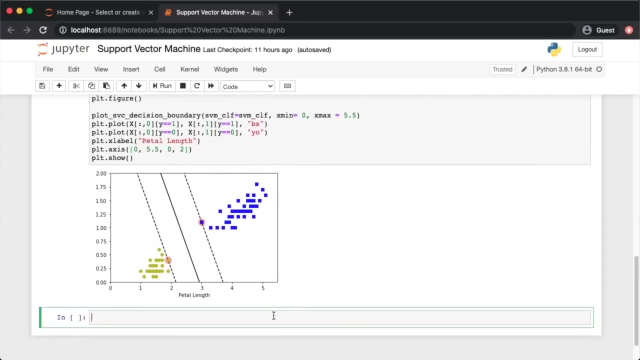 yellow circle. okay, okay. now let's see what happens when I add some outliers to my data. let's say I've got two outliers. say the first point is 3.4, 1.3 and the second one is 3.1 point two, zero point eight, and they're both classified as yellow circles. that 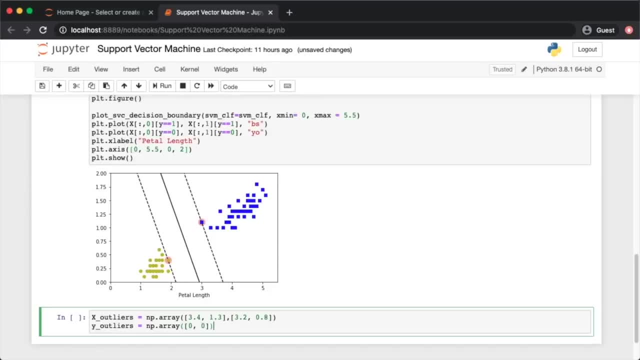 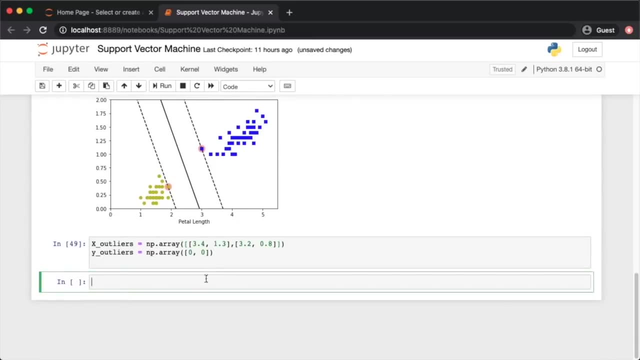 are class zero, okay, okay. so don't forget the double brackets in the first one, because it's a matrix. okay now, XO one is the data set containing the first outlayer. so we're going to concatenate on top of my original data set this outlier along the zero axis and it's corresponding y O one is using the same. 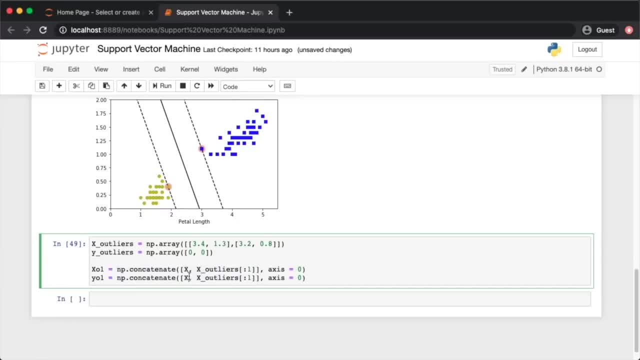 thing, copy paste it here. why over here? and why over here? and XO two is the one containing the second outlayer as such. Okay, Now let's create a classifier on the first dataset. Actually, let's see how the datasets look like. 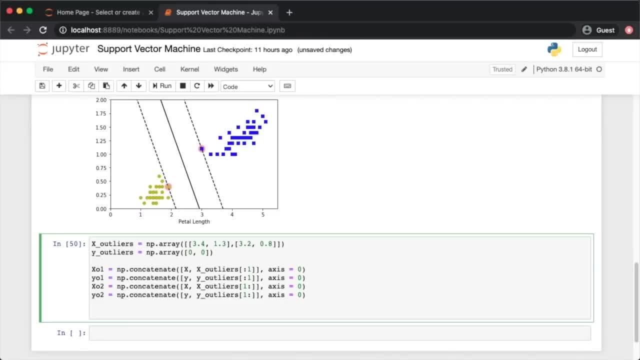 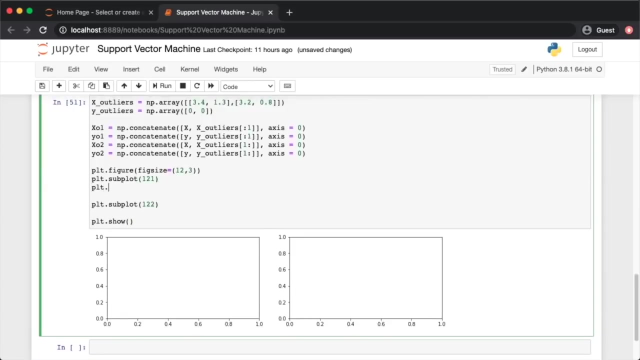 So I'm going to open a figure with the following figure size And in the first subplot, call it 121.. Second subplot, call it 122.. Let me show the subplot. Okay, In the first subplot I'm going to plot X01,. 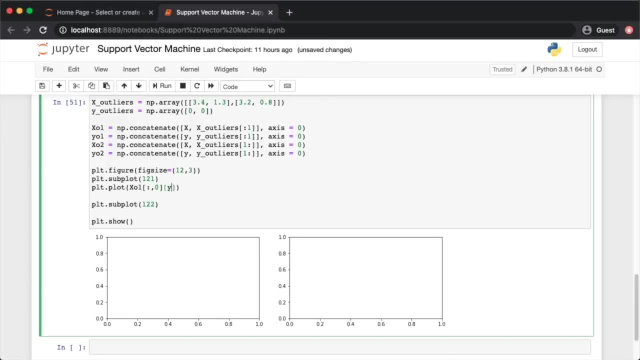 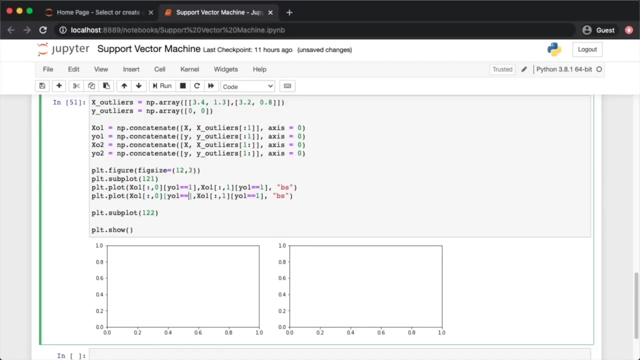 where Y01 is 1.. X01.. So that's the first class and blue squares. And likewise the second class and yellow circles. Okay, As you can see, here's my outlayer. Well, let's stick in an arrow over here saying this is an outlayer. 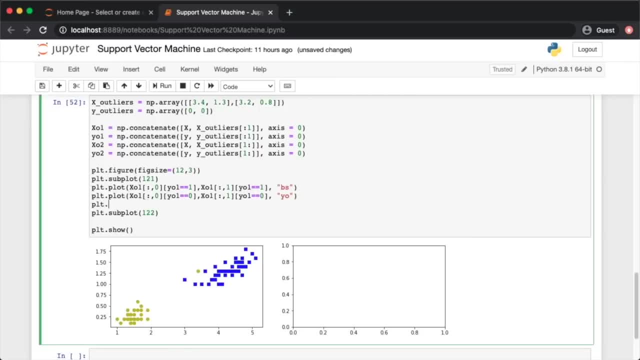 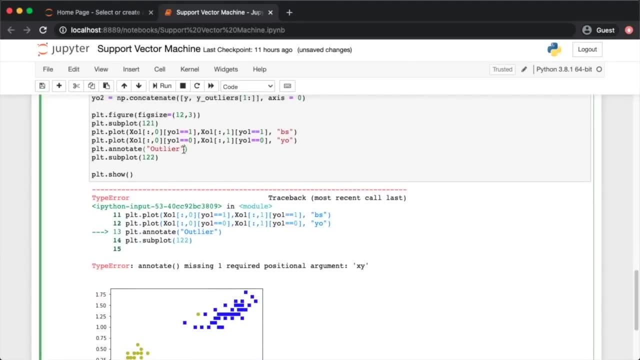 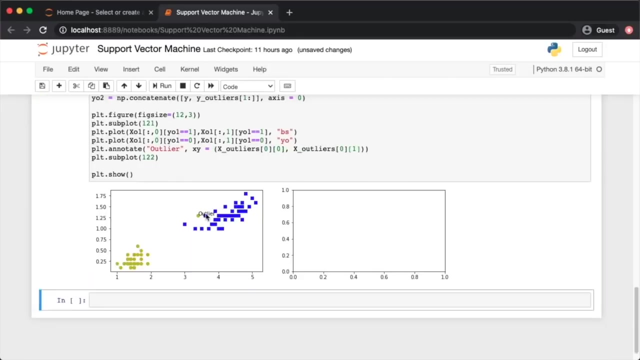 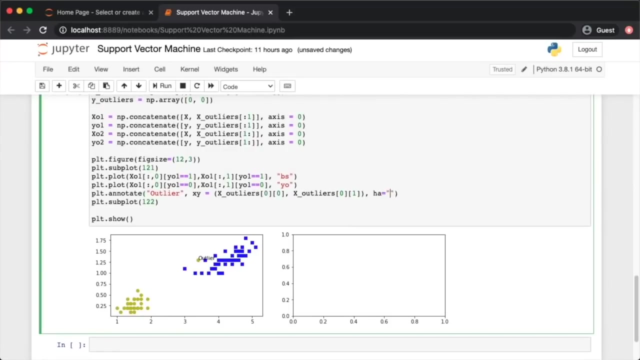 Okay, So the way you can do this is using the annotate function of plot. Say: this is an outlayer. Okay, It's missing some arguments that are the XY that should be pointing on the first outlayer as such. Okay, So let's fix this by including a center. 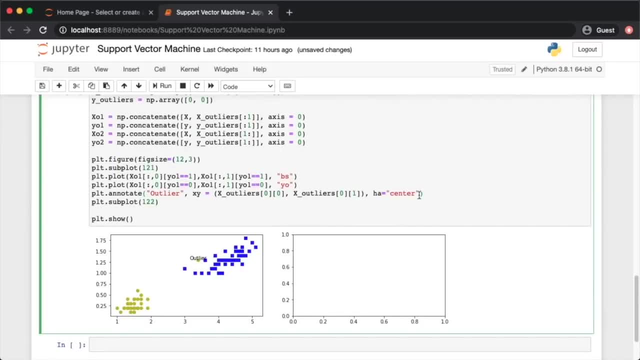 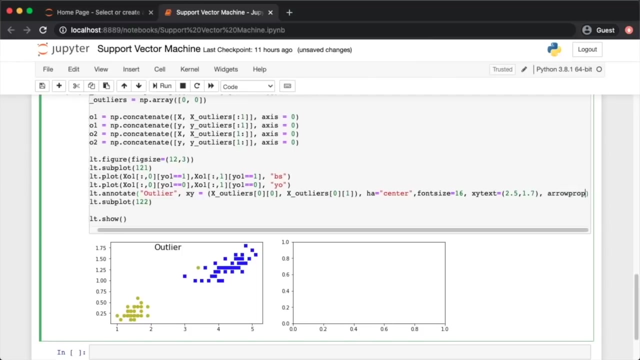 Okay, Let's increase the font size, Say 16.. Okay, Now let's indicate that it is a text with the following coordinates: Okay, Now let's put in an arrow Arrow props. It's a dictionary containing the color which we will color as black. 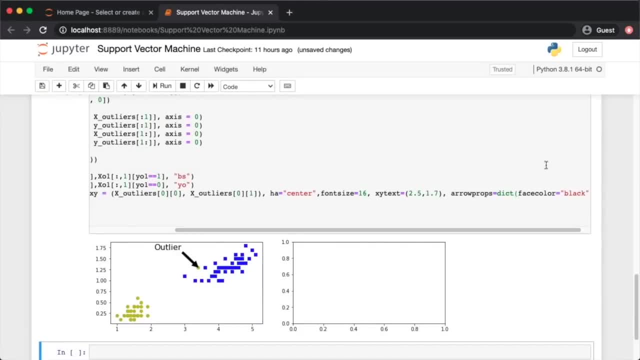 Okay, Let's shrink it because it's too. Okay, Okay, Okay, Okay, Okay, Okay. I think the minimum is 0.1.. Okay, That's good. Now let's limit our axis to I don't know plot axis. 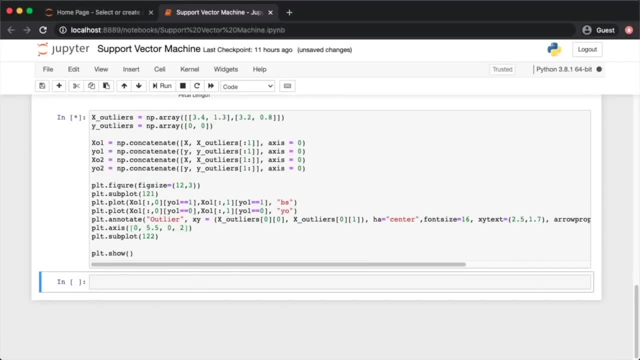 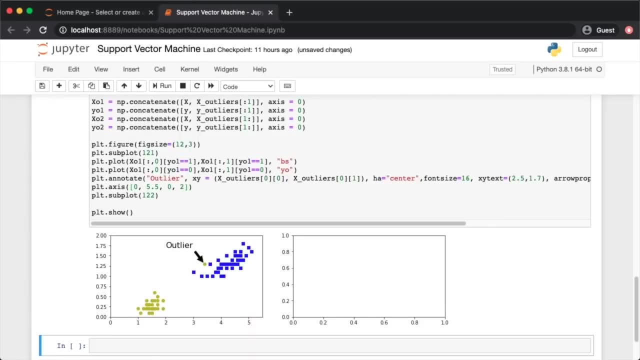 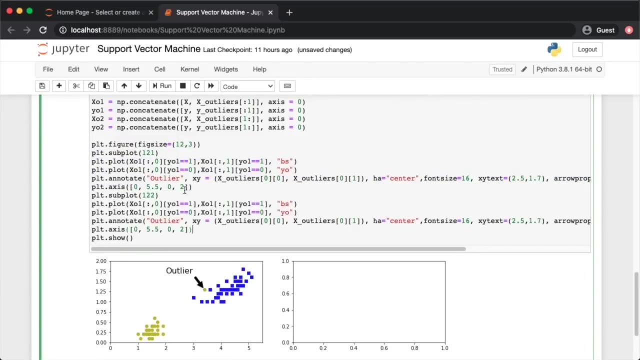 So x min, x max, y min and y max. Looks good, Looks good Now. I'll do the same thing for the second data set. So I'll copy paste just what I have over here: Instead of 0.1, I have an 0.2. 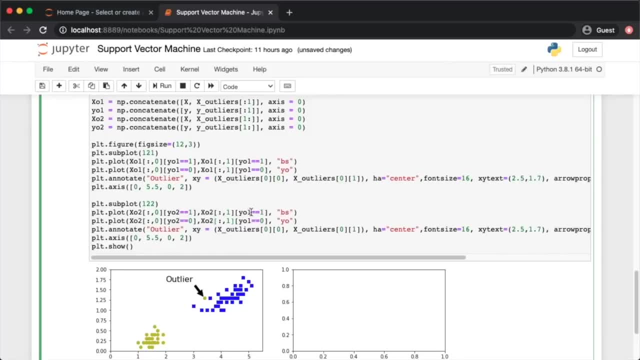 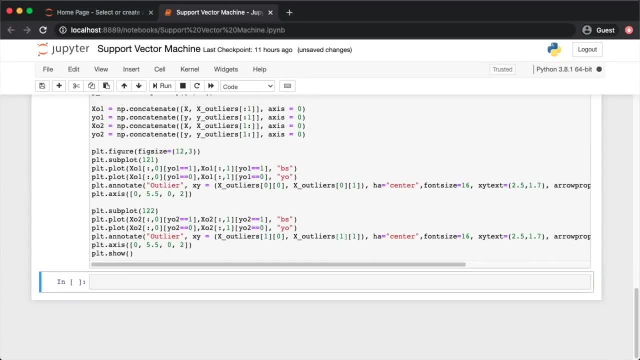 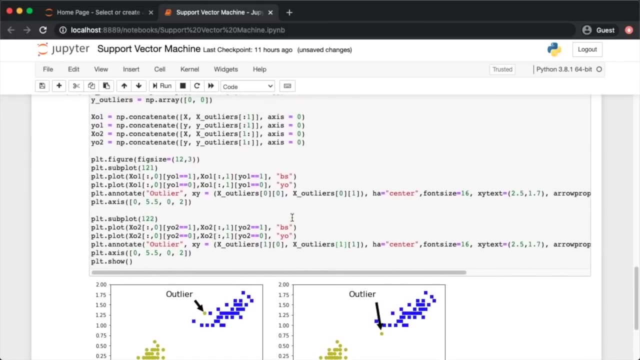 Right And over here it's a 1.. It's the second out layer. Okay, Okay, Looks good. Now all I have to do is run SVM here and here, So I have my. ah, I still didn't okay. 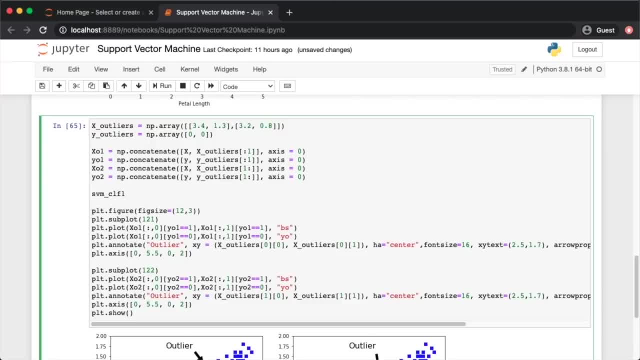 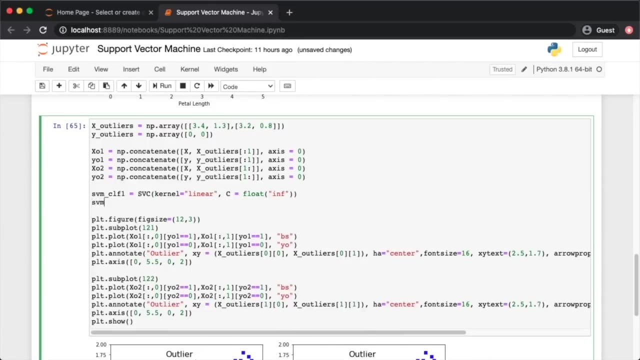 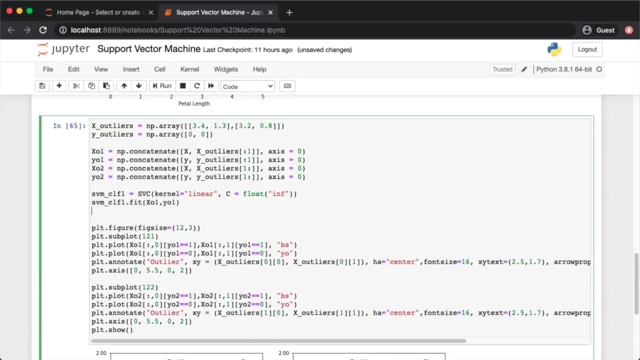 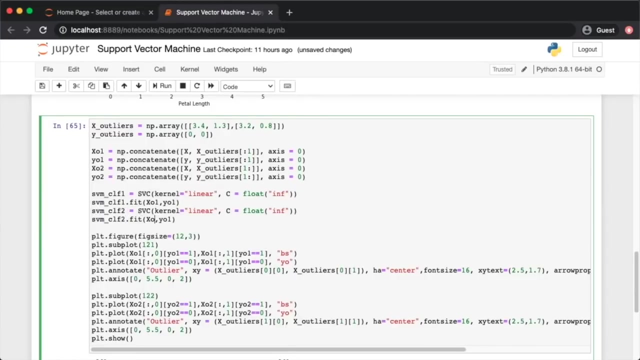 So let's create an SVM classifier 1 on the using SVC linear kernel. Pass it the C, that is infinity, It's hard kernel- And fit y 0, 1 versus x 0, 1.. Likewise, I'll create a classifier, call it 2, on the second data set as such. 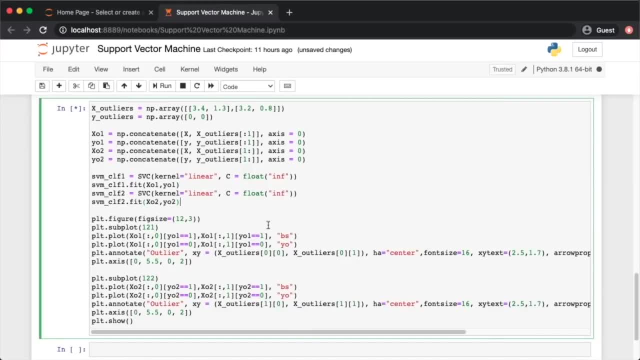 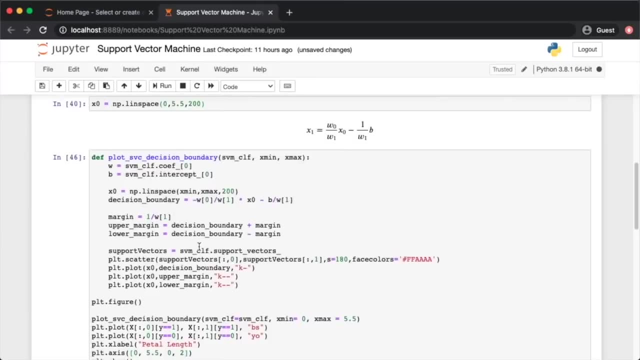 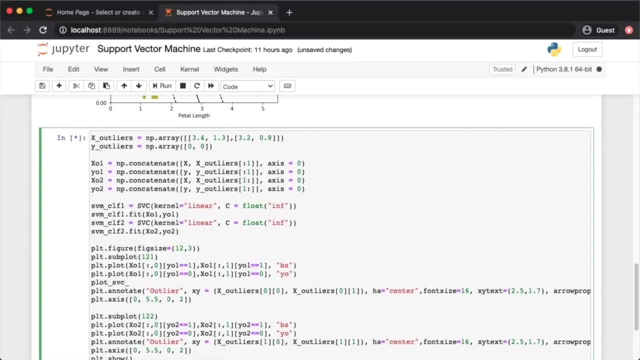 Right Now, just over here, I will call the function that we wrote over here to plot the decision boundaries. Right, So, plot SVC score decision boundary. I'll pass it the classifier, which in this case it's CLF1, passing it x min and x max. 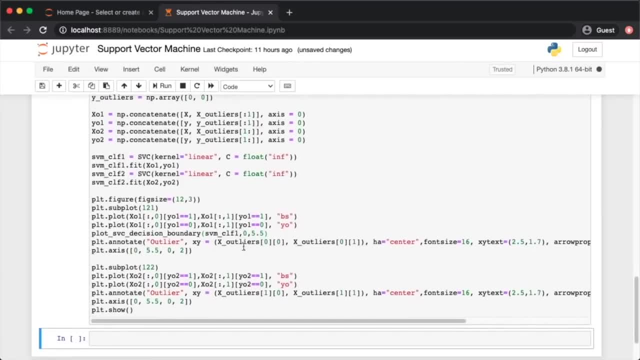 And, as you can see, it's taking a lot of time because, because of the floating point, precision. So right here, instead of infinity, I threw in x max. So right here, instead of infinity, I threw in x max. So right here, instead of infinity, I threw in x max. 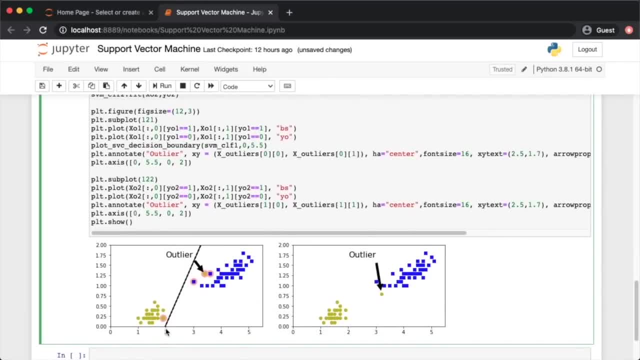 So, right here, instead of infinity, I threw in a large number and it's working And, as you can see, we don't have margins right here, because SVM failed on this dataset And the reason why is because this dataset is not linearly separable. 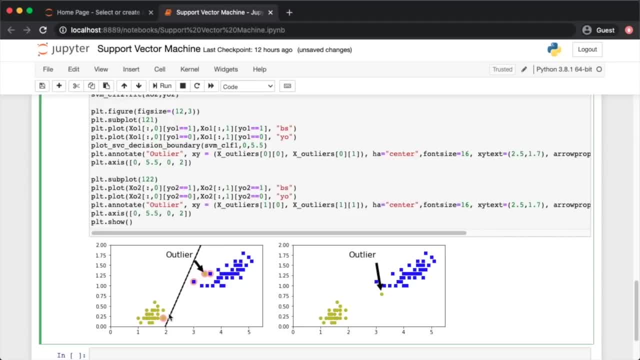 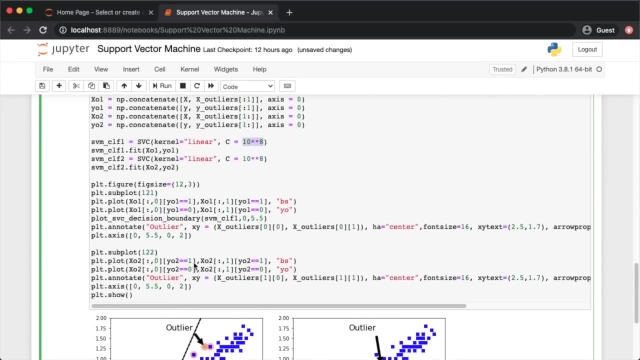 And the reason why is because this dataset is not linearly separable. As you can see, we don't have any, you know, margin. Actually, the margin is zero, Actually, the margin is zero. Let's try to, you know, print the margin together. 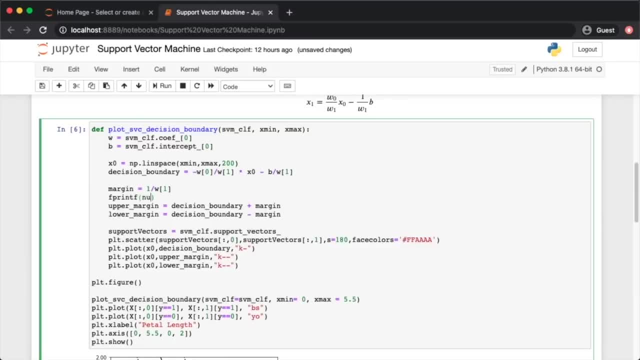 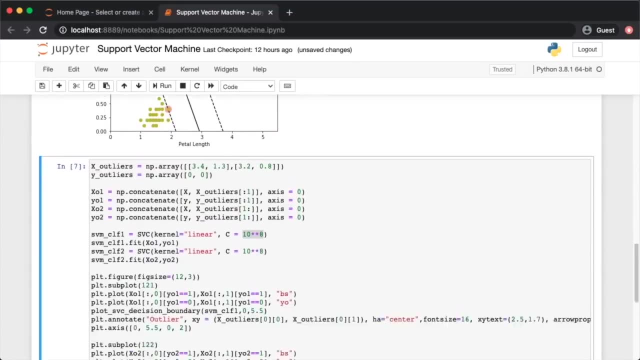 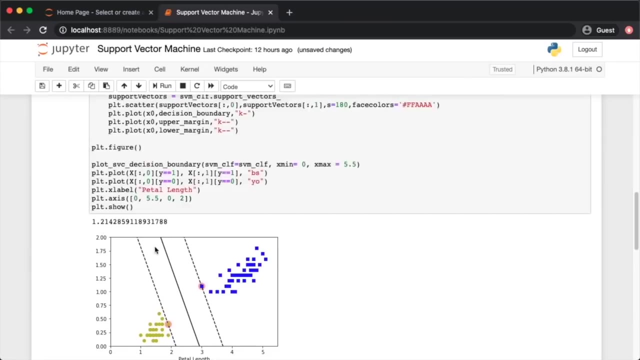 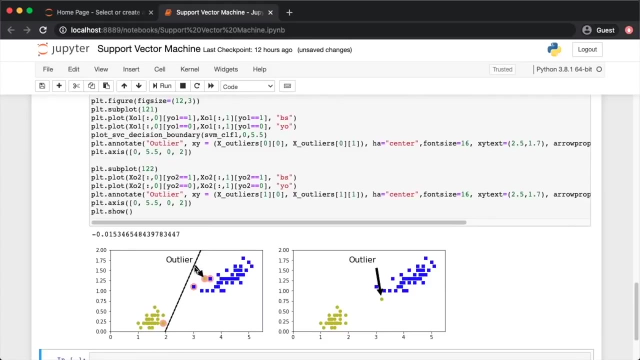 Well, you just kind of run through it: margin, so STR margin. actually it's a print like this: okay, there you go. the margin is really small as compared to the previous case. okay, so really small. that is, the margin is actually on the upper and lower margins are actually on the decision boundary and the way we can see that is to zoom. 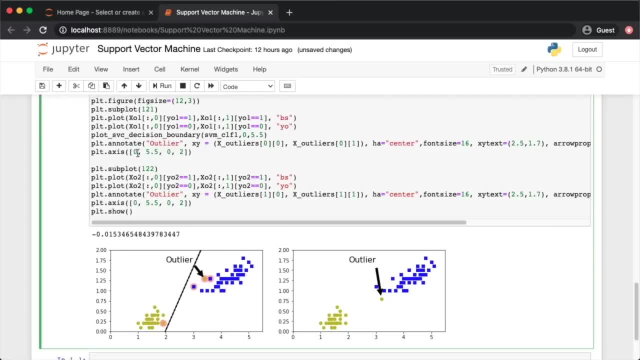 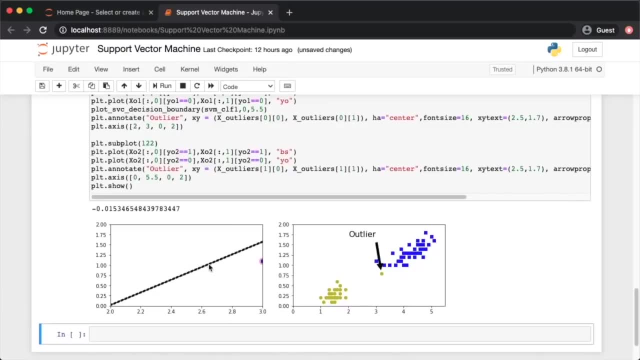 in over here. you can do this by limiting the x-axis, let's say between two and three. as you can see, they're over there. okay. let's limit, let's say, the y and x, the y values- um, i don't know- between 0.5 and 0.5. 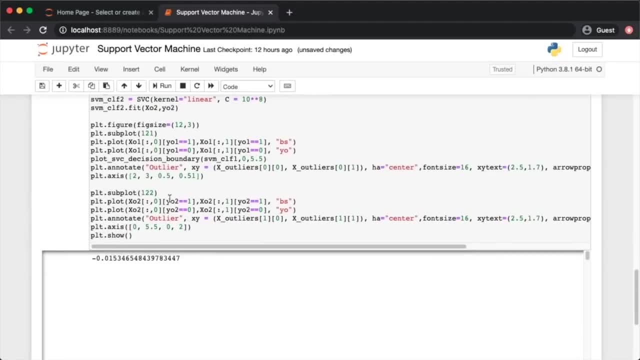 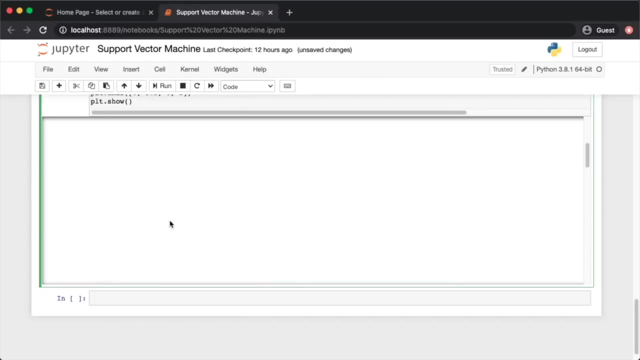 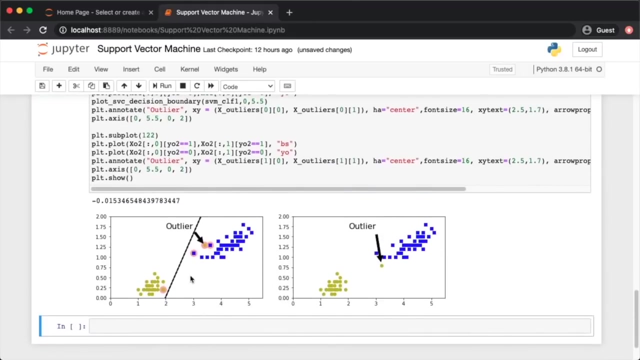 1. um, oops, so let's say between 0.5 and 0.6. nah, it's not working. ah, it's over here. so there you go, okay. um, okay, let's return those values as they were. there you go, okay. so the margin is zero. we couldn't. 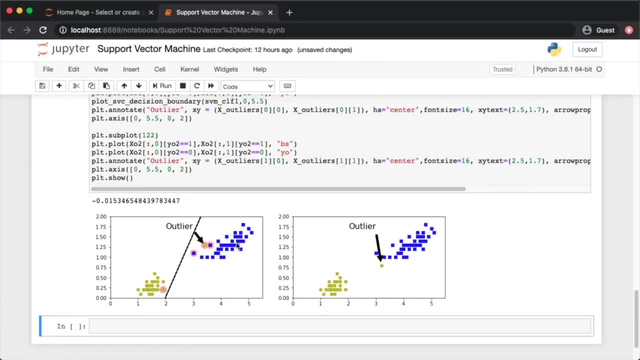 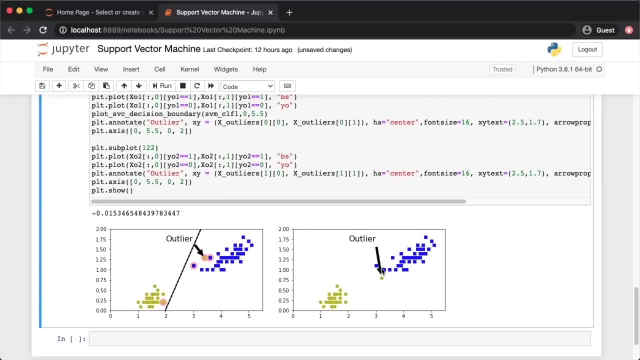 find the margin of 0.5 and 0.6, so let's return those values as they were. there you go. okay, so the margin is zero. we couldn't find a proper margin to linearly separate both data sets, so that's where it fails, however, over in this case, actually let me. the arrow here is aligning on the 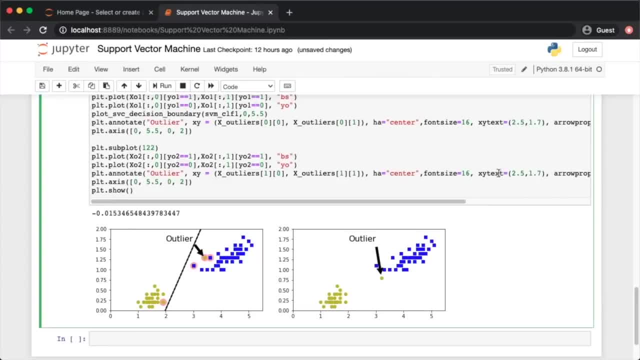 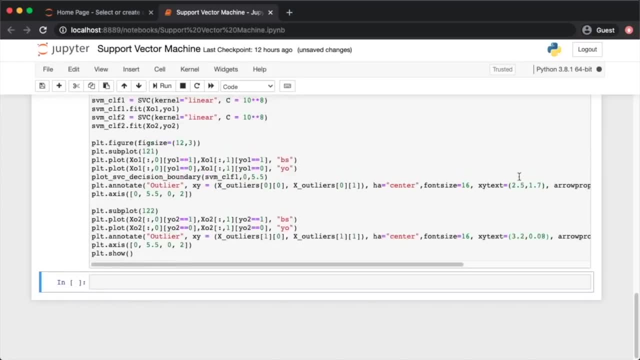 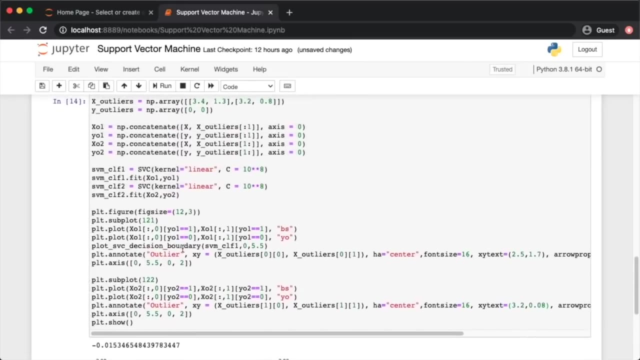 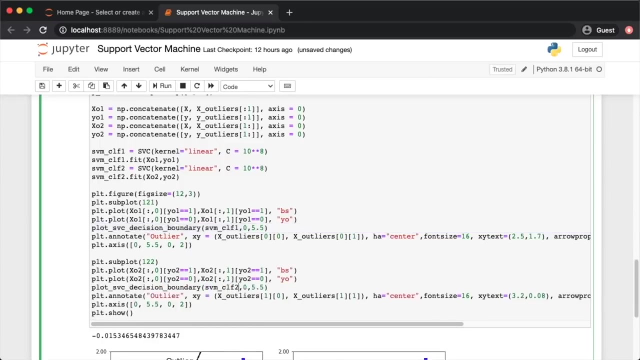 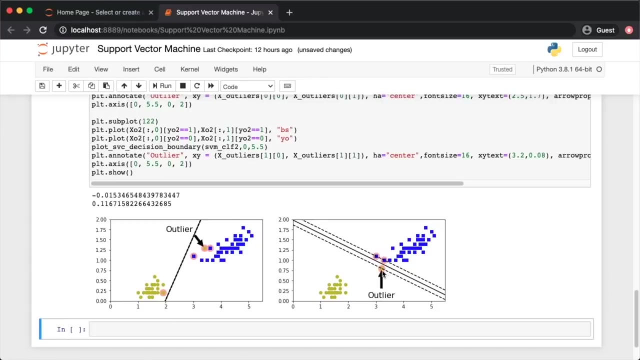 is covering my data set, so let me move that just a bit. um, let me change this over here. okay, better, and let's run. actually, let's plot the decision boundaries over here. as you can see, a small margin, of course, due to the out layer, but we managed to separate both. 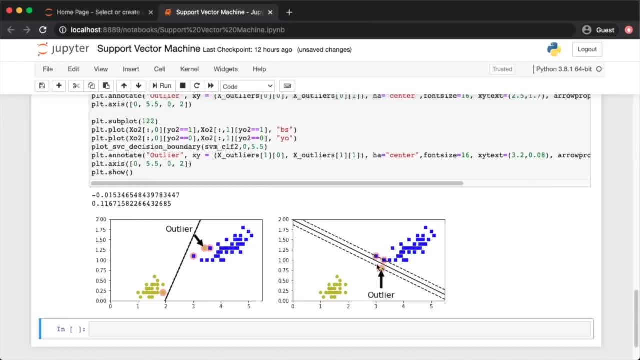 data sets. this out layer still falls here, but it's an out layer. it's not around them as normal as it should be. no, it's pushed away from its friends, right? okay, so we have a problem. what is it? it's when i'm given a data set that is not linearly separable. 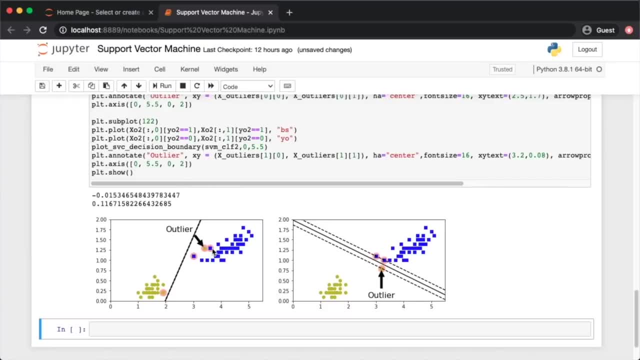 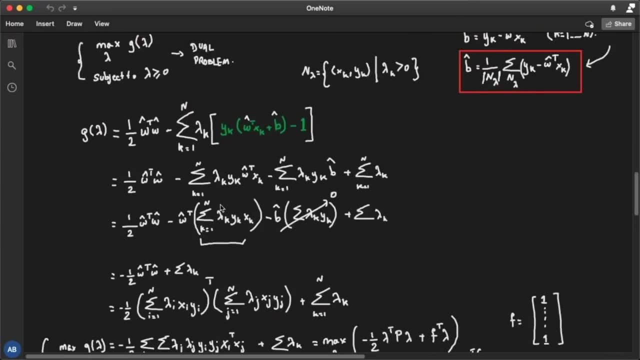 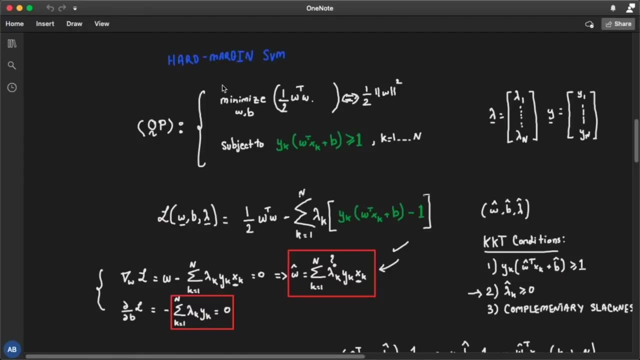 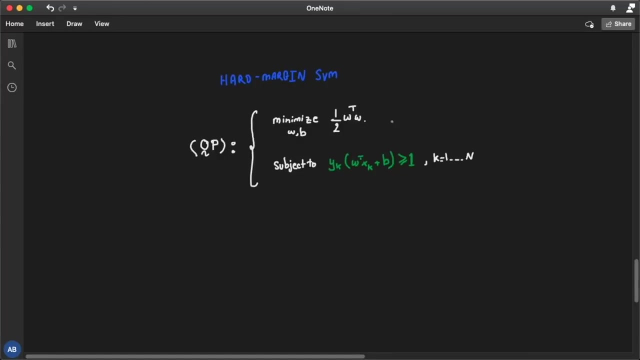 i cannot run this type of svm. that is a hard svm and that's where the smooth or soft svm comes into play. so, instead of this problem, instead of the hard margin svm, which looks like this, we're going to take a smooth approach or a soft approach. so we're going to add new variables over here which we're going to call 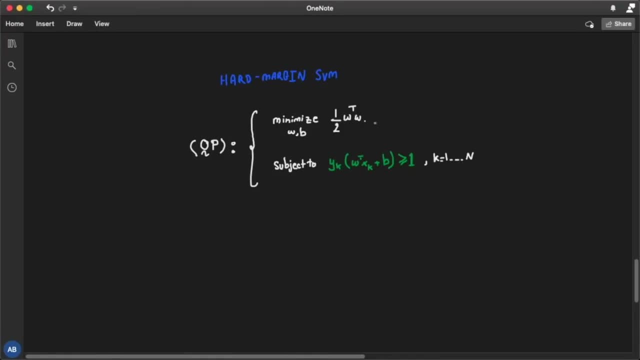 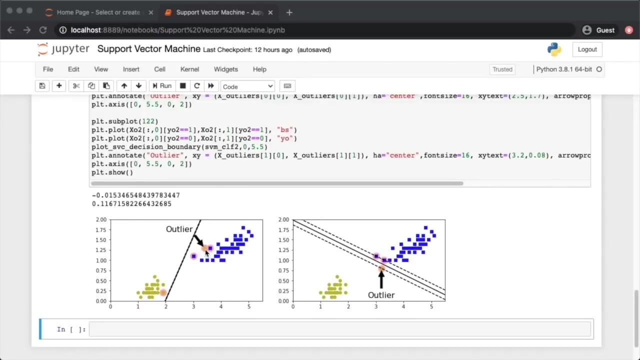 the soft approach, which we will be calling xi. right, that will you know, make this problem softer, and what i mean by softer is that i'm allowed. so if we go back here, i'm allowed, or let's put it that way, and i'm going to let this outlier for a moment, i'm going to cover my eyes. 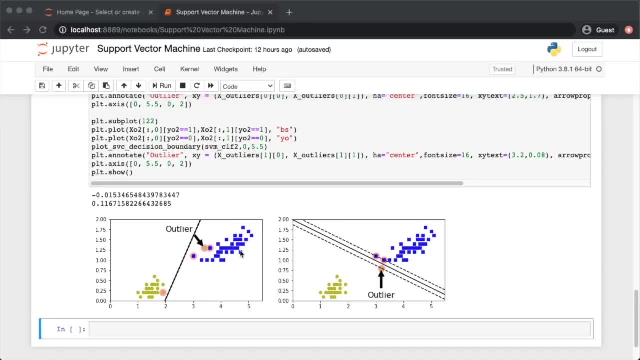 and allow this outlier to fly away from my diagram, fall with the blue curve, with the blue class, okay. so, with that said, this will change the problem completely, that is, we're going to have a new line over here that pretends that this outlier falls with the blue within the blue class, okay. 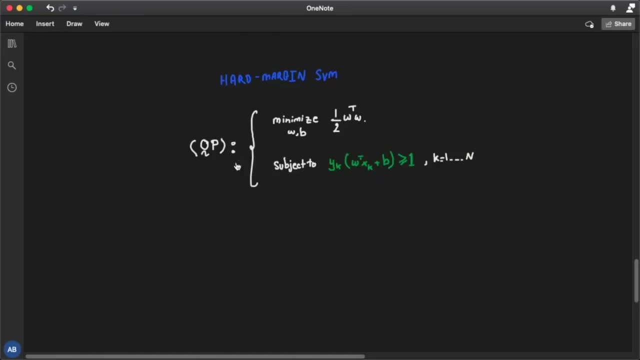 and we're going to carefully modify the problem so that we're allowed to do so. so we're going to have a softer constraint. so over here, instead of a one, i'm going to have a 1 minus xi i, xi k. so i've got n? xi's, xi k's for the kth. 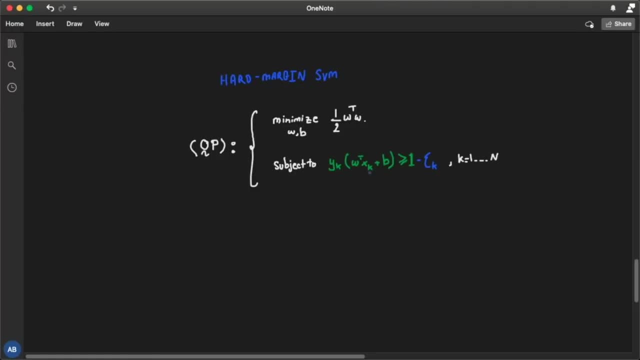 training set. so for each x, i, i, xi k. so i've got n, xi's, xi k's for the kth. so for each x, i, i, xi k, so i've got n, xi's, xi k's for the kth training instance. so for each instance i label, i attach a psi k with it. 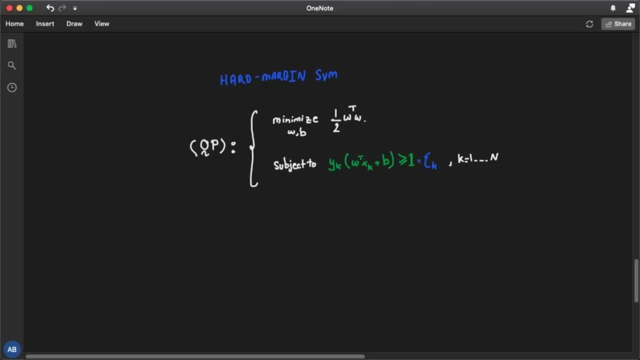 which is going to serve as a smooth, smoothing parameter. that allows me, to you know, move the margins, to you know, fit the data better. formally speaking, this new constraint will allow us, will allow an adaptive margin. that is so here. my psi k's are positive. they're not allowed to be. 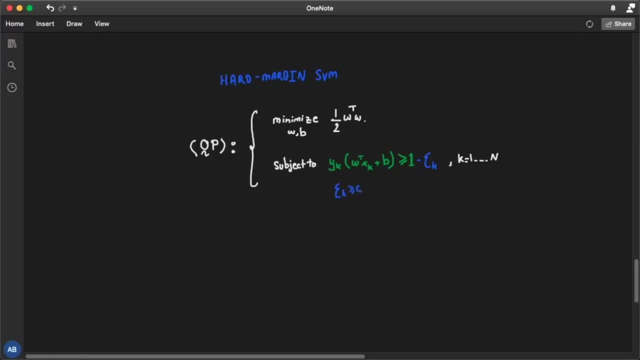 negative. if it's negative means i'm getting a smaller margin. so those psi's are are allowing an adaptive margin and the cost will thus penalize those size. so we're going to have a hyper parameter over here that operates a certain trip, that reports a certain trade-off and we're going to sum over all size as such. so if a certain 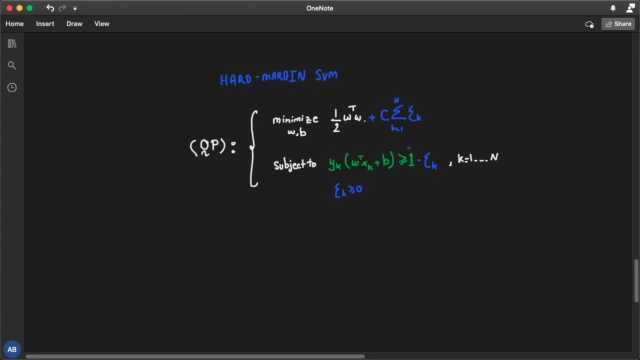 data point is not an outlier. xijk should be, you know, between zero and one, so that this term over here is positive. so in that case, you know, i have a small penalty. i don't penalize this instance, okay. however, when a certain outlier is classified in the 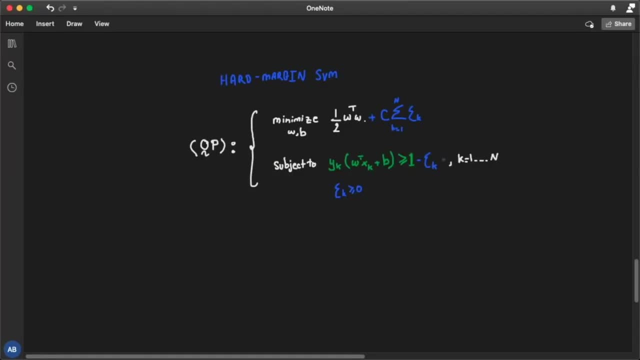 wrong class. this psi k is going to be greater than one and if that's the case, then my cost function is going to, you know, um, it's going to increase. so, that said, i'm going to try to minimize all misfits. so not only am i doing hard, so this term is the hard part, right is hard margin. 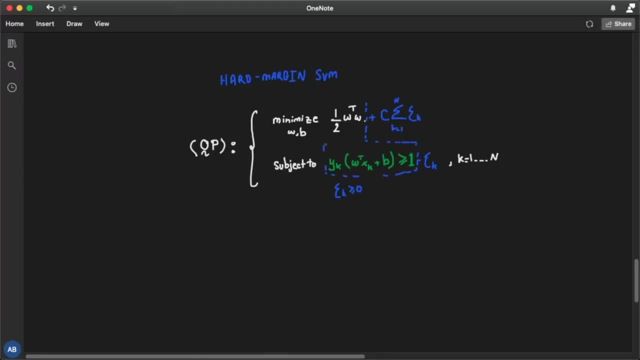 so not only am i applying hard margin, no, i'm trying to minimize the effect of outliers, right? so if there is an outlier that you know i can't do anything about, it's going to be penalized in the size. okay, and you can see that i'm trying to minimize the effect of outliers. 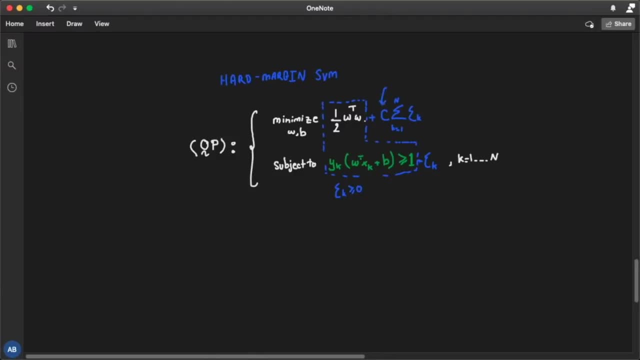 as you can see, we have a c parameter over here that is a hyper parameter. it will control the relative weighting between the cost of making the margin small and ensuring that most training instances have adaptive margins that are at least one in the ideal case. therefore, we're going to minimize the total sum of penalties as well. okay, does that make sense? 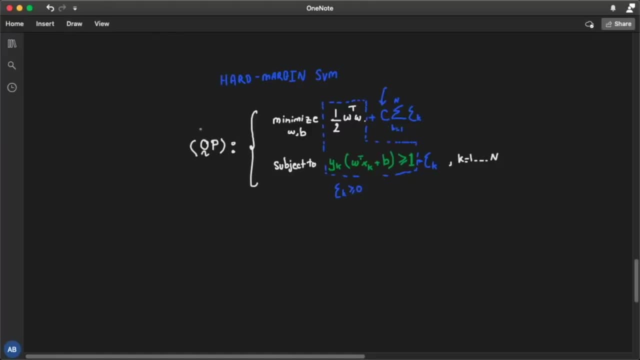 so if i were to write down the lagrangian, it is: oh, and, by the way, the minimization is also with respect to xi, and this problem is now the soft margin, svm. so the lagrangian right here is a function of w, b, xi, xi and. 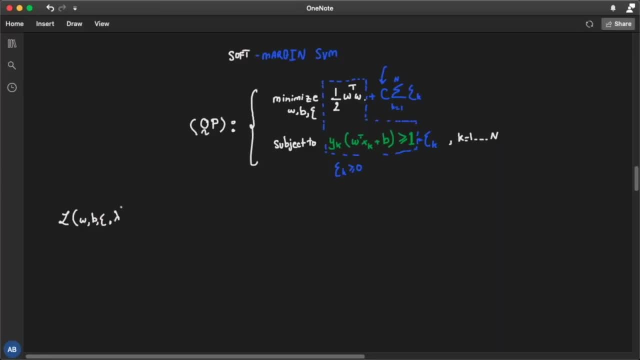 our lambdas, which is the cost, half w. transpose w plus c sum on xi, i's minus sum on i. going from 1 to n lambda i multiplied by this thing minus I, I x procedure, this thing, That is yi into w. transpose xi plus b minus 1 plus xi i. Now, as 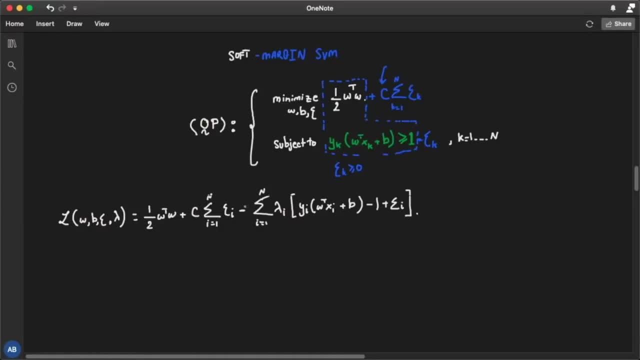 before. this problem is a quadratic program. The cost is quadratic in terms of w, linear in terms of xi, and we've got linear constraints And they also satisfy the KKT conditions. So I'm allowed to, you know, solve the partial. 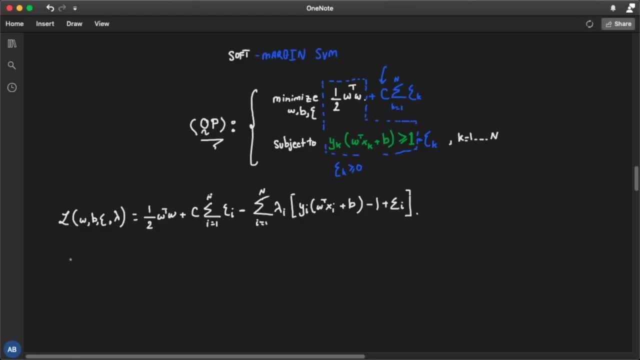 derivatives with respect to L. So setting the gradient with respect to w. on L, we get that. over here we get a w, And right here we get a minus sum on i, lambda, i, yi and xi. right, Setting this thing equal to 0, we get the same. 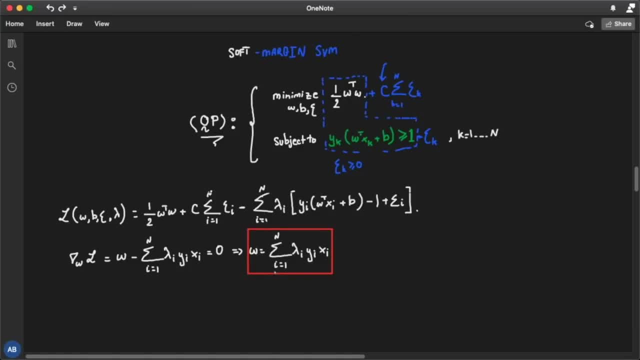 expression on w. Now let's derive with respect to b. on L We get the only term depending on b is the sum of lambda i yi b. So the derivative of that with respect to b is sum on or minus. sum on lambda i yi, That is 0.. So right here we have another condition that should be. 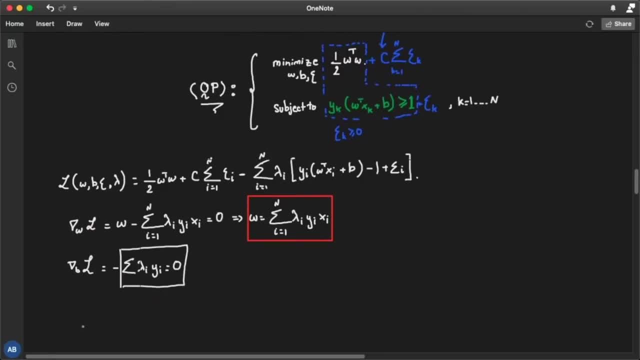 satisfied. And last but not least, we need the derivative on xi i of L. But but which is so? over here we've got a c sum on xi i, That is a c Okay. Then over here, the only term depending on xi i is lambda i. xi i, That is a c Okay. 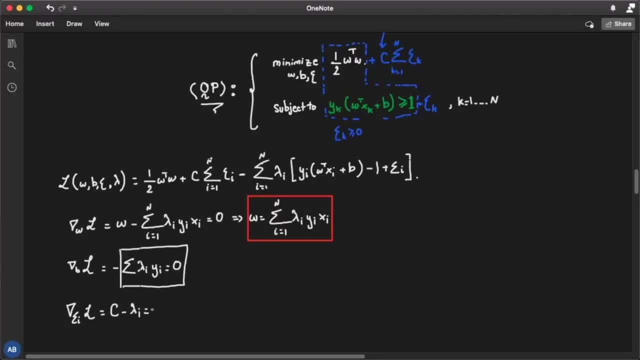 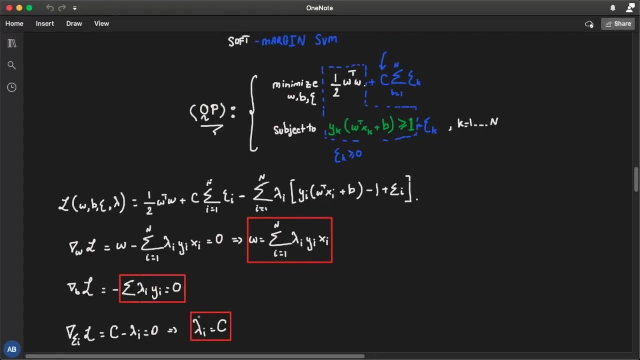 minus lambda i, that's zero. so we get that lambda i is c. actually, this guy over here is an upper bound on lambda i because we're solving the problem with equality constraints and all my lambda i's should be positive according to kkt. so this guy translates to: 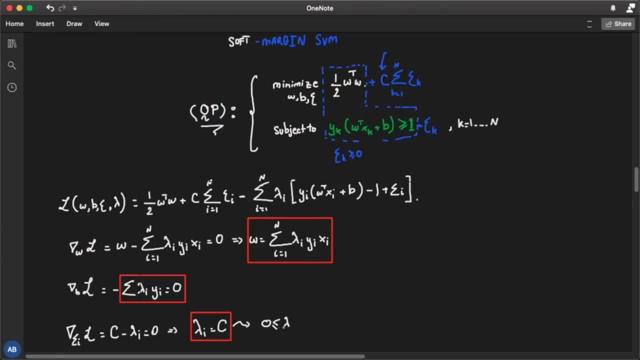 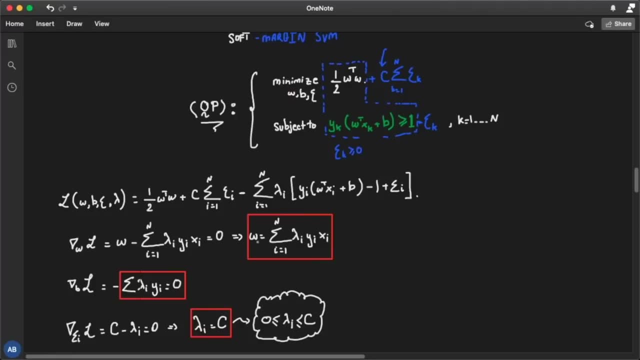 all my lambda i's is positive and my c is the upper bound. right now we have an expression for w, we need we need an expression for b and, as we did in the hard margin case, the b could be achieved from the equality, from the, from the 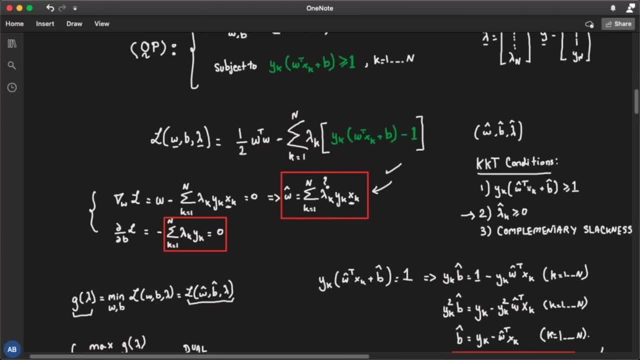 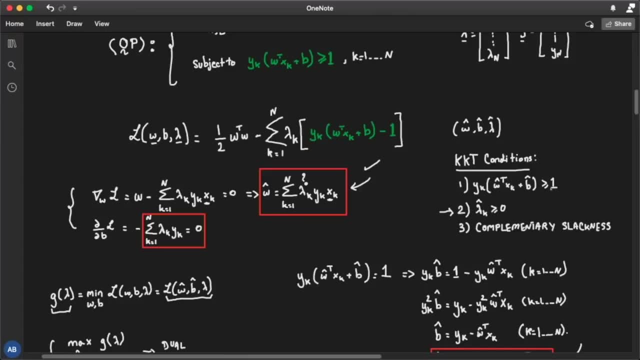 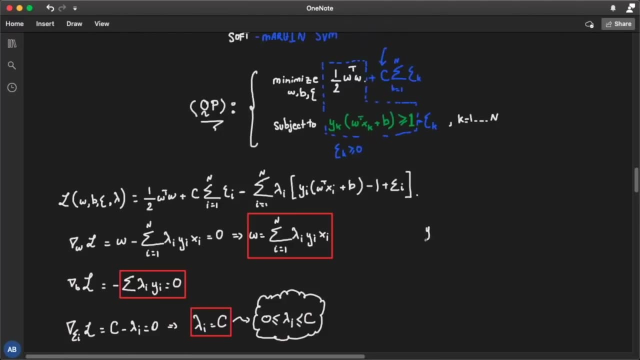 kkt condition. the first kkt condition, that is yk, w hat, xk plus b hat is equal to one. so we satisfy the kth constraint with equality. in our case it is yk into w. transpose xk plus b is equal to one minus xi. k. 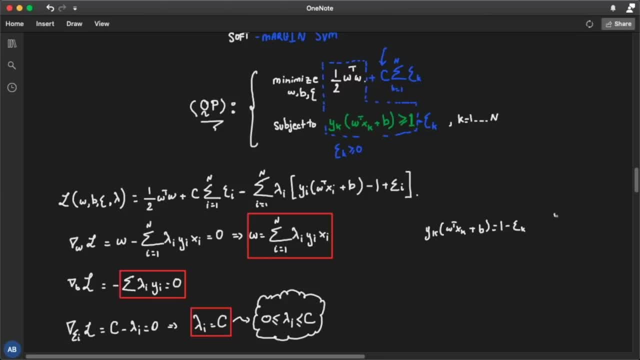 multiplied by yk on both sides and use the fact that yk square is one, because yk is plus or minus one, we get that w transpose xk plus b is yk into one minus xi k, then b is yk one minus xi. k. 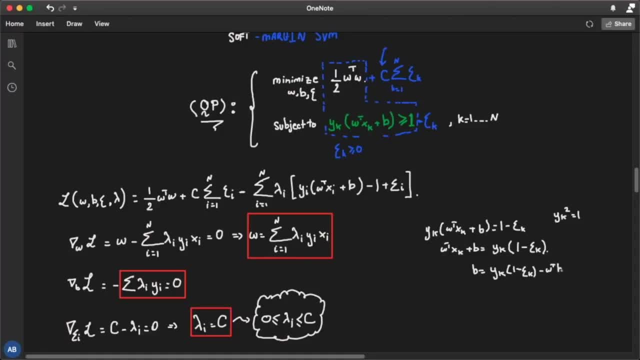 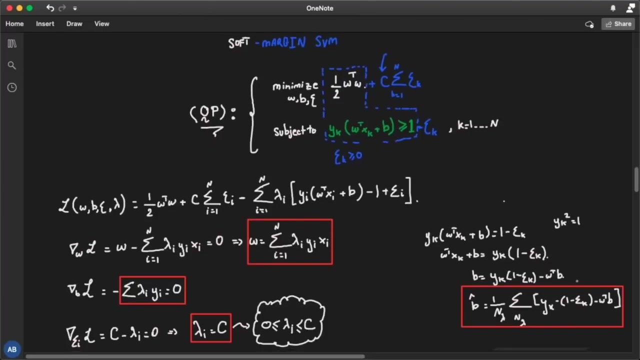 minus w transpose b. okay, and of course you can average to, as we did in the hard margin svm. you can average over all instances to achieve a more robust estimator. if b as such, minus w, transpose b. now, as previously, we need the lambdas to compute the w and the w to compute the b. 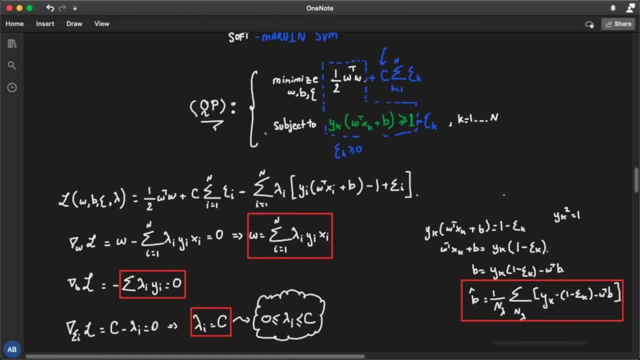 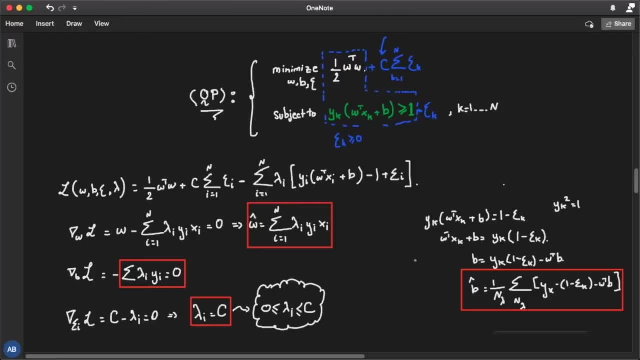 so we need the dual over here and the dual is achieved by replacing w hat and b hat and the cost. so, as previously, we can see that if we replace w hat and b hat over here, so w hat, b hat hats everywhere w hat b hat. we have that. the sum on lambda i y i times b hat that has to be zero because of this. 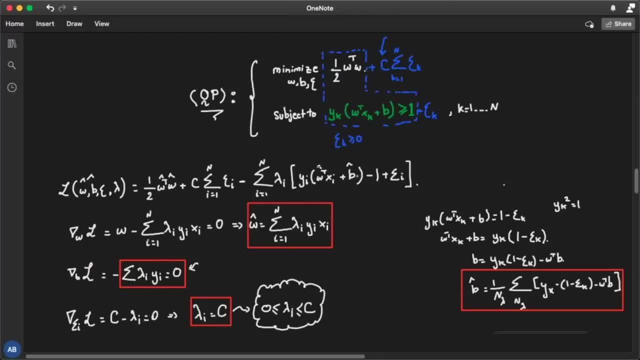 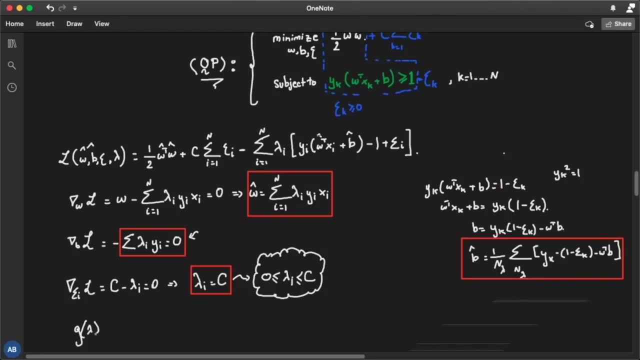 condition over here. so this term is gone and this term is actually combined with this term to give me uh. so going down here it gives me a minus half w hat, transpose w hat, w hat and the c sum on lambda i, on xi i, and right here you have a minus sum on lambda i, xi i, where lambda I is. 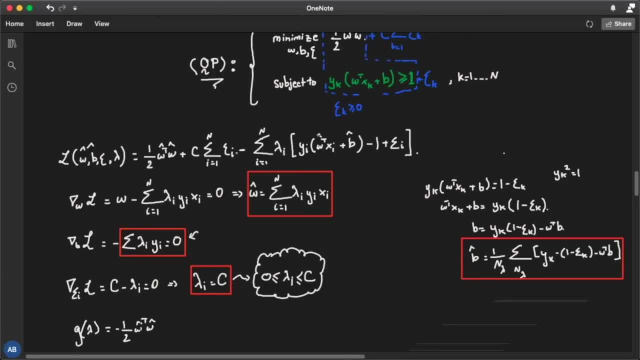 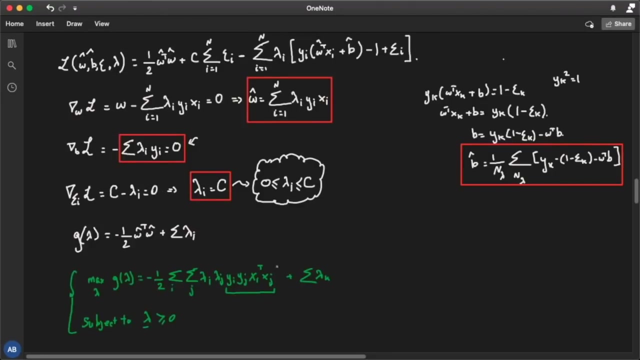 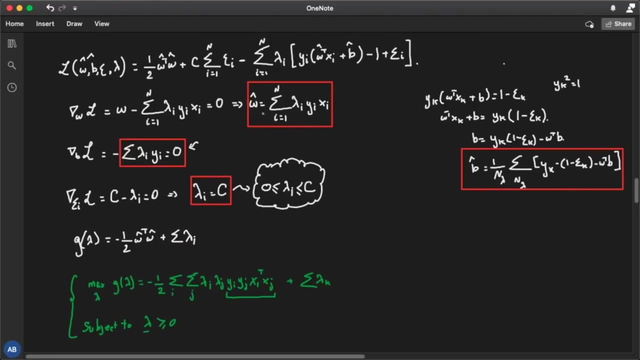 c. we're solving with equality. so both cancel and you're left with a plus sum on lambda i. so you get the same exact dual function as before to compute the lambda case, which then you can compute the b hat and then the w hat. okay, and that's how you solve soft margin. 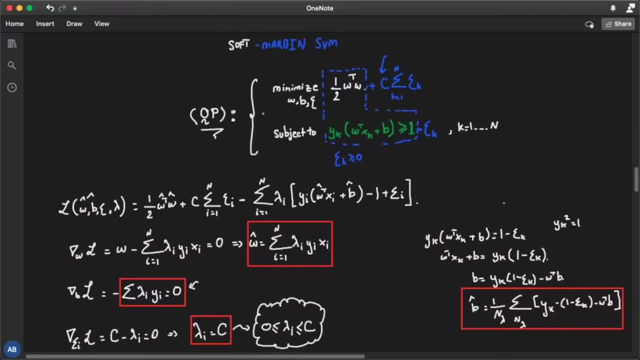 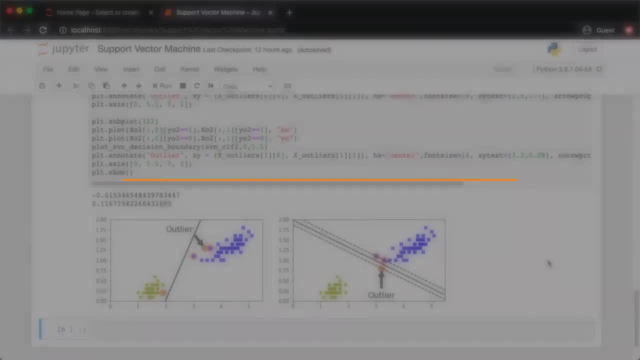 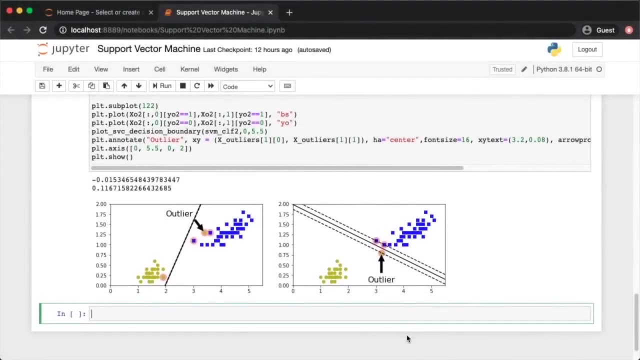 using its using the lagrangian function. okay, now let's see how to implement soft margin svm on python. so since i'm going to be training more than one svm, it's better to use pipelines. so from sklearnpipeline i'm going to import a pipeline, so let's first get. so i have my iris up here. 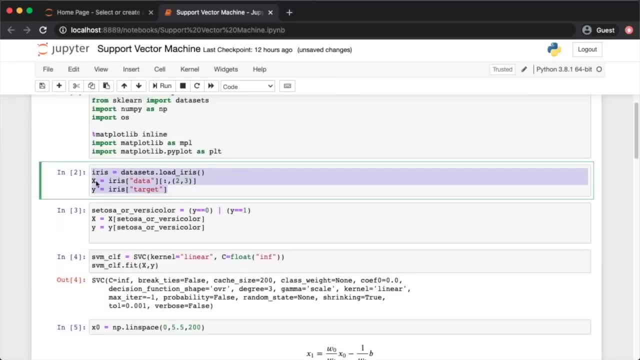 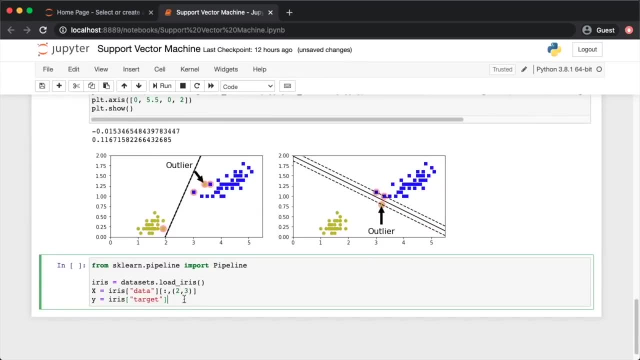 right here. copy paste this code right here. but this time i'm going to take the iris, that is, two, as one class and one and zero as another class and i'll use as type mp float. so i'll copy paste the the code that i had previously. 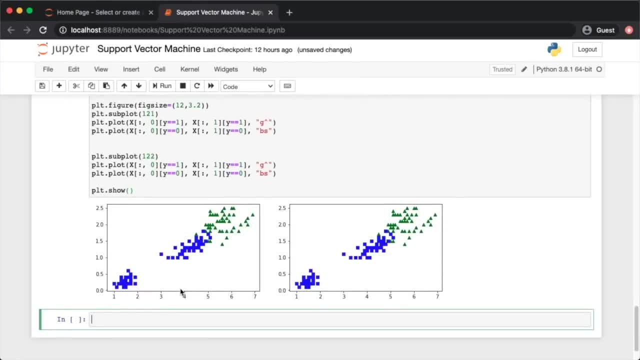 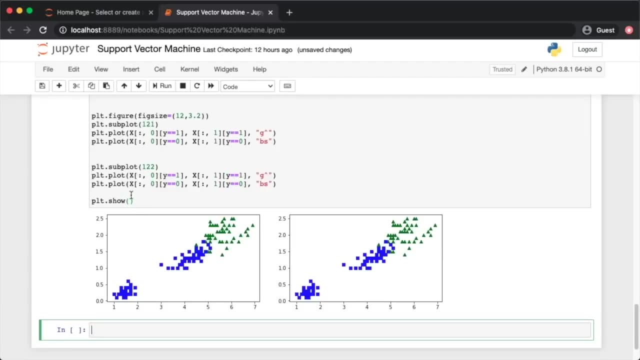 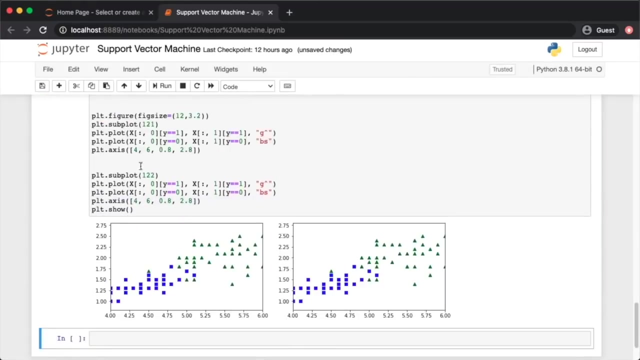 so this is the data set and, as you can see, we've got some outliers over here. they're overlapping. let me limit my axis in both plots: x-men, x-max, y-men and y-max. okay, you've got here some outliers. now let's see how two different 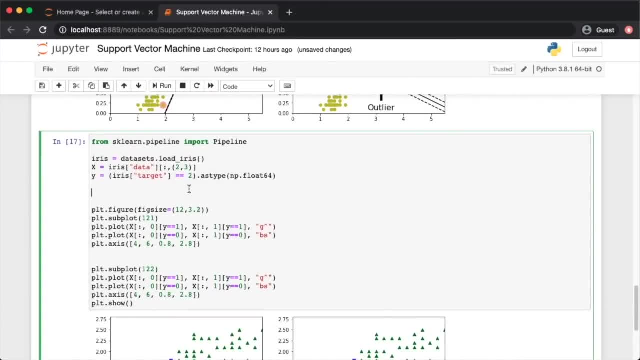 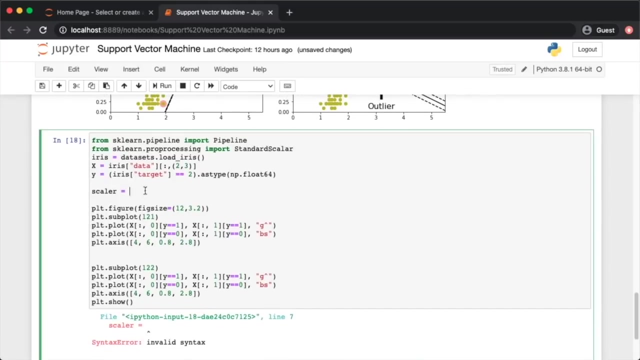 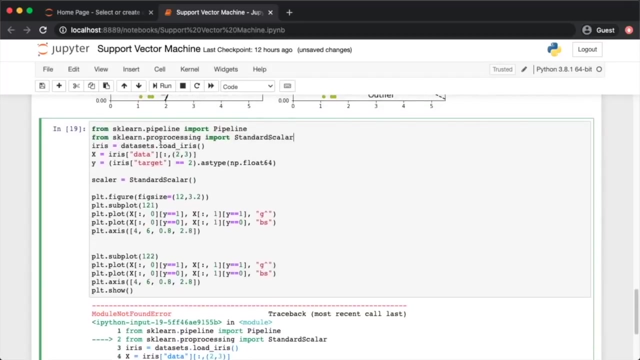 soft margin svm perform okay. so to launch a pipeline i'm going to first use the scalar and for that i need to import from sk learn dot pre-processing. going to import the standard scalar. the scalar is a scan is a standard scalar. oh, it's not pro processing, it's pre-processing. 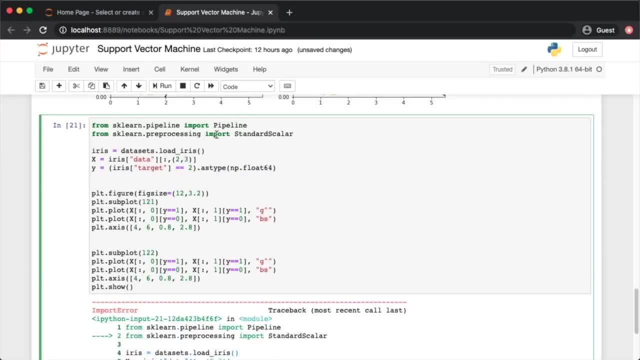 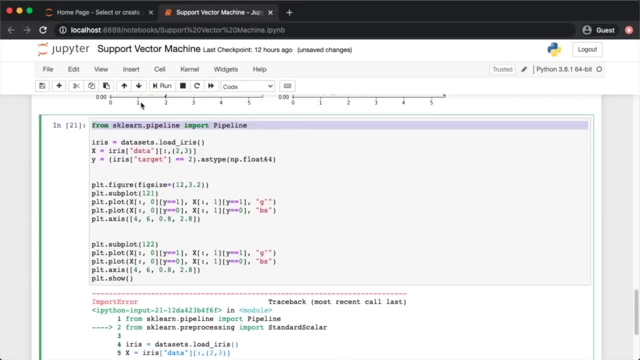 okay, we can do without this pipeline thing. whatever, i'm using python8 and it seems that it's not working. okay, so let's go, let's do each one separately. so, linear svc: i'll pass the c hyper parameter one first. i'll indicate a hinge loss. 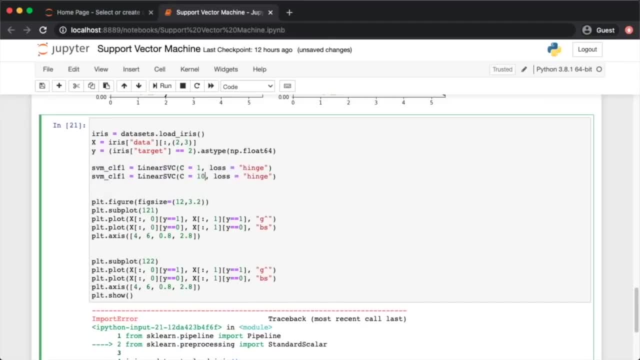 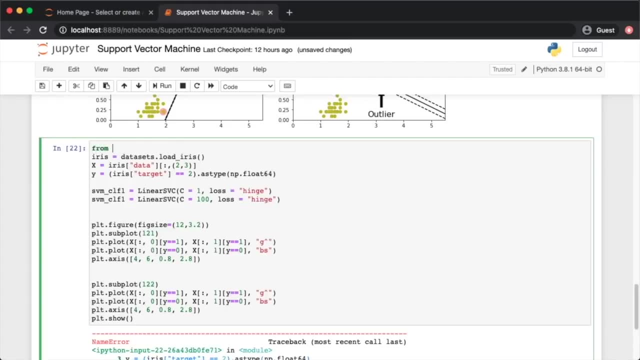 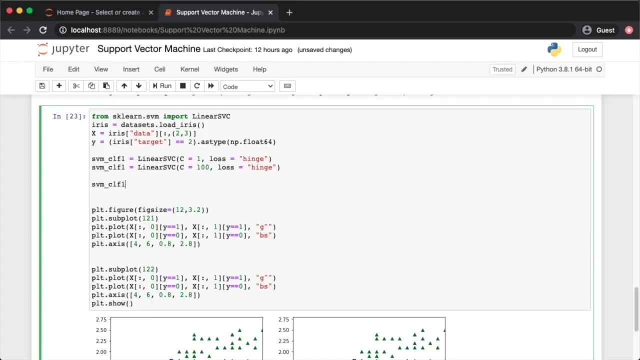 and another one, but with this larger c, let's say a hundred. so to get your linear svc you go to sklearnsvc and import linear svc. okay, and now let's fit. so svmclf1.fit y versus x and same thing for 2. okay, we have a warning. 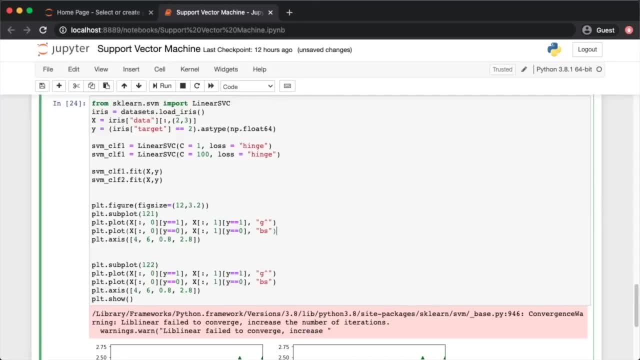 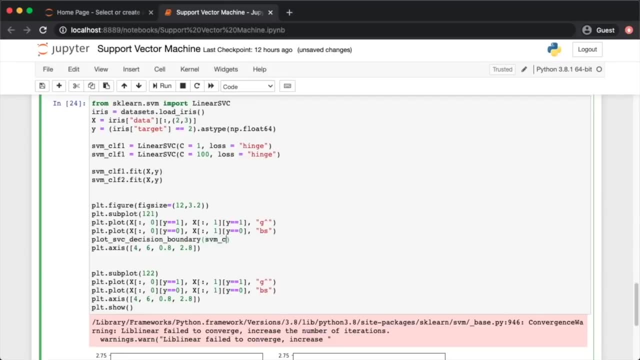 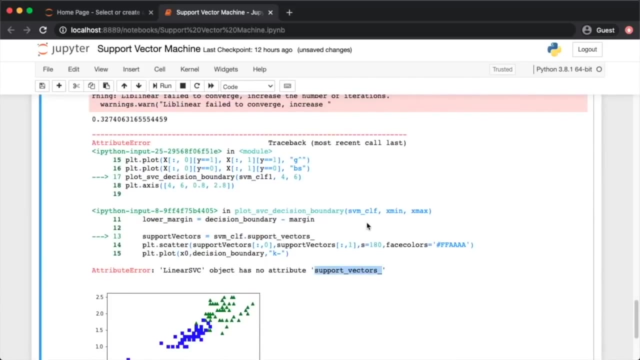 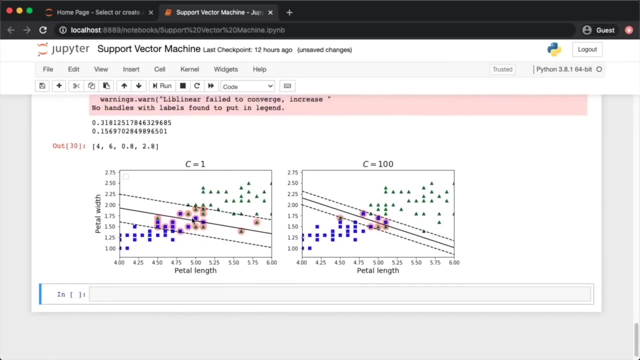 no problem, and right over here i'll call the function that we implemented earlier on: svm: underscore clf1 x min, x max, and we don't have support vector attributes right, so we need to compute that we need to do this manually. and there you go. so, as you can see, with a smaller c, 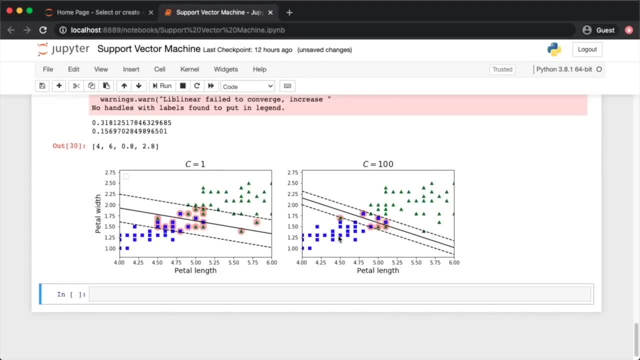 we accept more outliers, right. as c goes large, we have less and less outliers, right. so the c is a trade-off hyper parameter. the larger it is, less outliers but also a smaller margin. smaller c is: we have more outliers but a larger margin. okay, so that's about it. 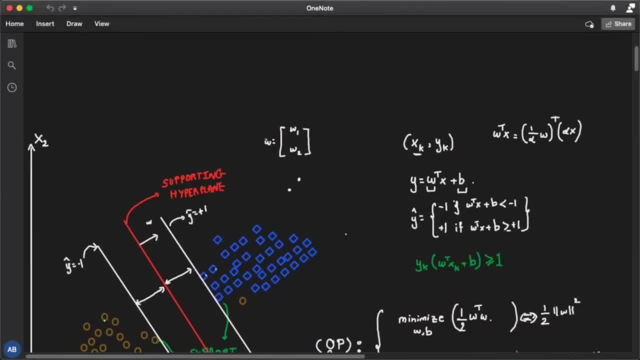 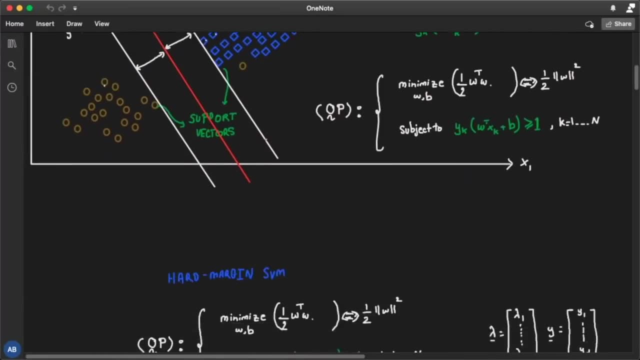 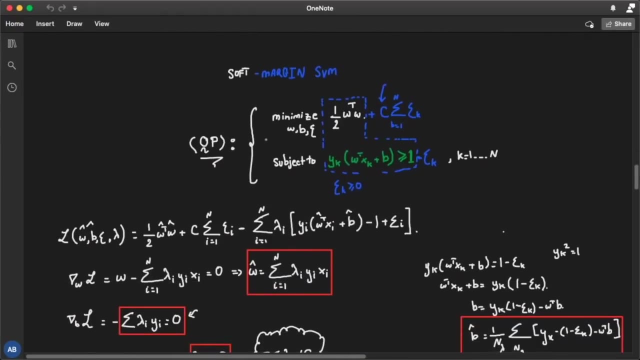 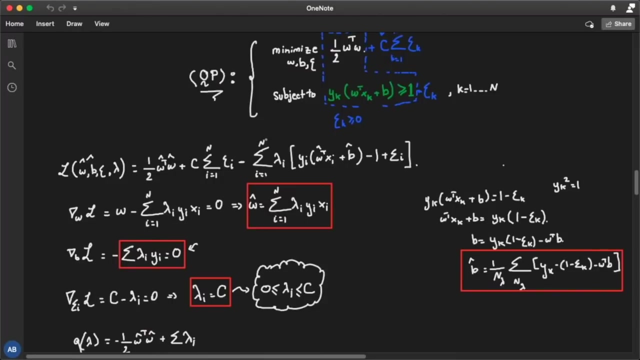 for this lecture. we pretty much did a lot of stuff. we started out by what an svm is, how to formulate both hard and soft margin svms, how to formulate their corresponding convex optimization problems and how to solve them using the lagrangian and kkt conditions, along with their respective python. 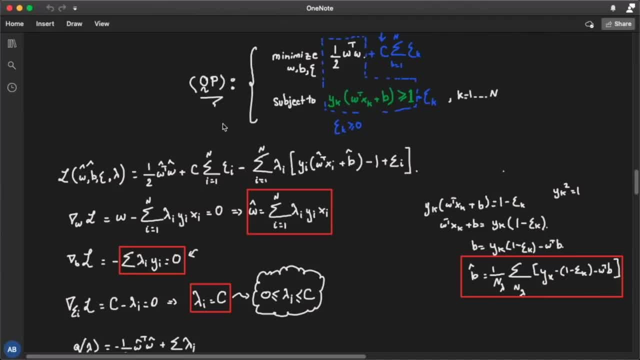 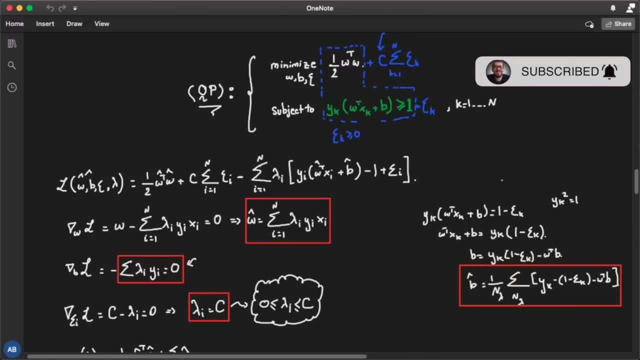 on implementations. so thanks for watching. if you found this lecture beneficial, please leave a like on the video. subscribe to the channel. if you have any questions whatsoever, kindly leave a comment down in the comment section below and i'll make sure i'll get to it as soon as possible also. 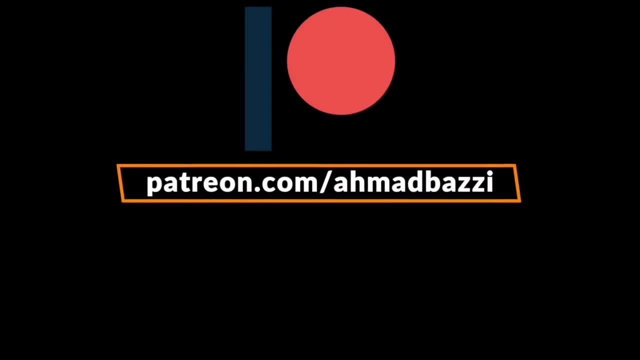 consider donating to my patreon account any amount you wish. thanks for watching and i'll see you in future lectures.